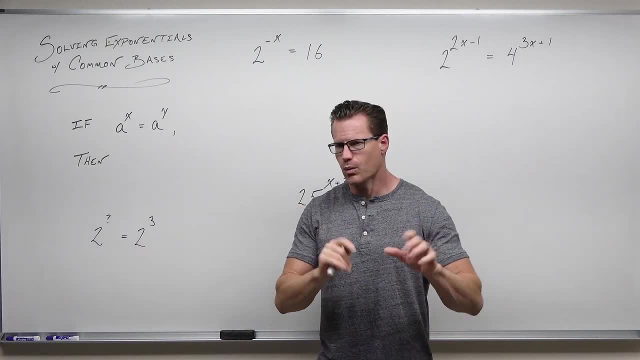 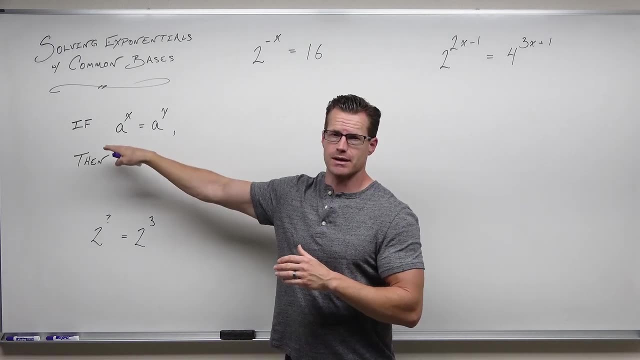 we can find common bases. Now, why does it work? Well, if you have an equation with exponential expressions and that's it all. your terms are exponentials. basically, it looks like this: You have one exponential equal to another exponential. If you can make it so that you have 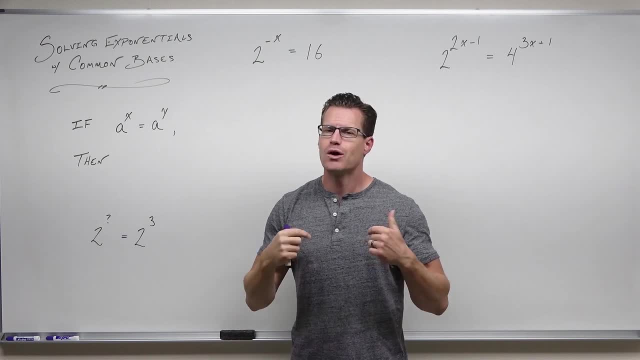 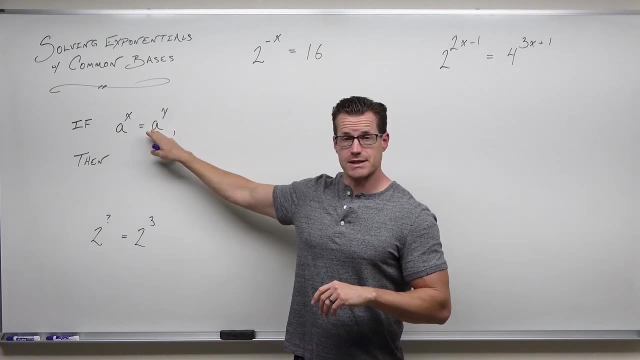 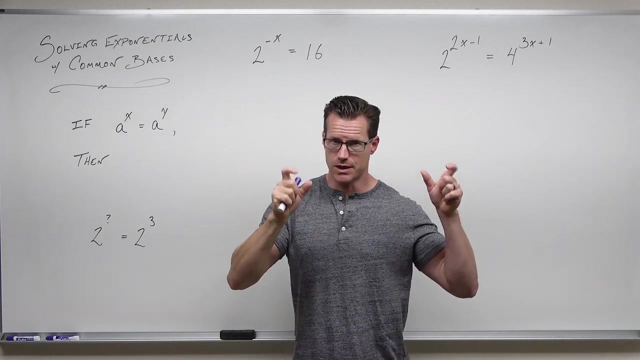 the same exact base on both sides of your equation, we can make something happen. We can say: hey, does it make sense that if this and this have the same base and these are equal? the only way that can possibly happen is if the exponents are also equal, And that's. 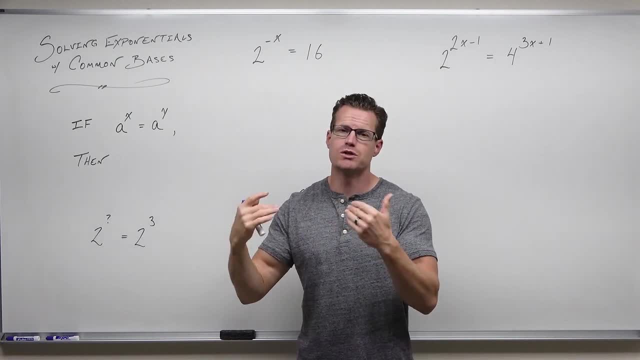 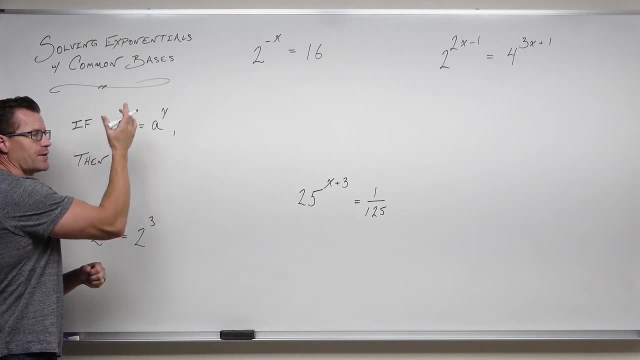 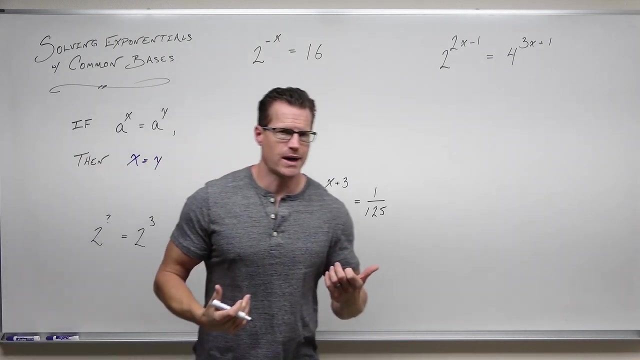 a statement. That's the special case for solving exponential equations. when you don't need logarithms is if, and only if, you have these common bases here. So if a to the x, you equals a to the y, if our bases are the same in an equation, then your exponents also have to be. 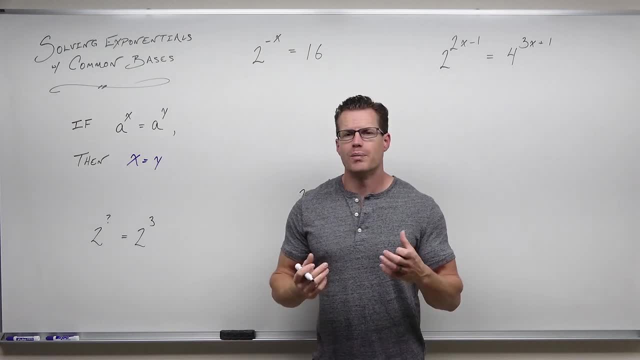 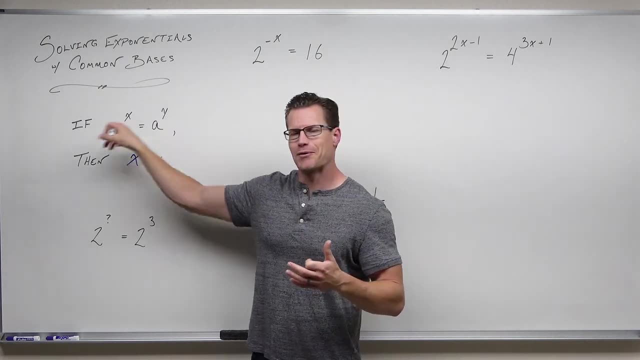 equal. That seems pretty straightforward, I hope, But here's the point. There's really nothing happening here. There's no real math that you show. You don't need to cross out the a's. You can- I love crossing stuff out, but you don't have to. This is just a blatant statement saying: 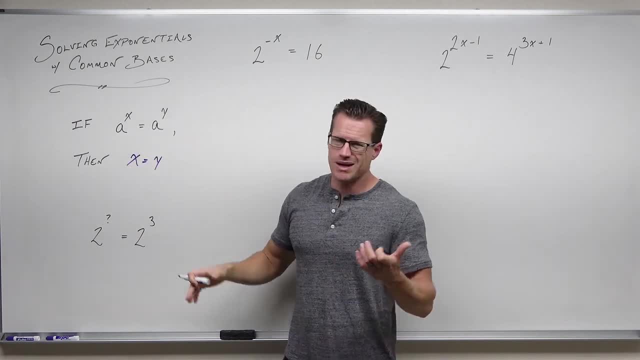 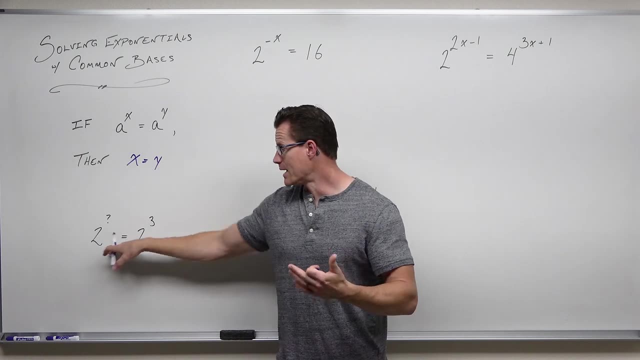 if you have an equation with your bases, the same exponents also have to be the same. Take this, for instance: If you have two to the- I don't know, equals two to the third. well, the only way these can possibly be equal is if you have. 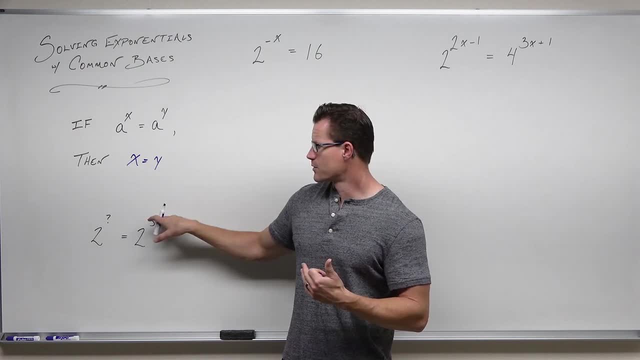 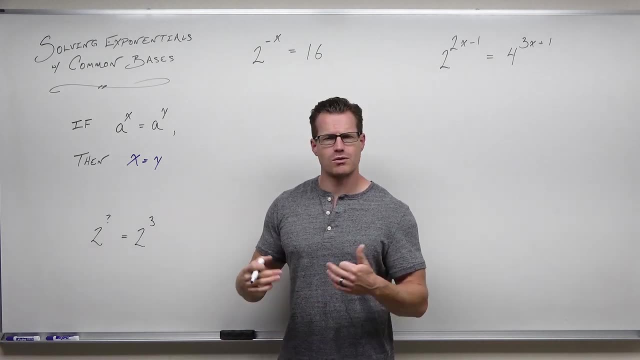 the same base here. you have the same exponent here. Two to the third is eight. Two to what power gives you eight. Well, two to the third would be eight. So we'd say this question mark equals three. Well, question mark's a really awkward way to write something we don't. 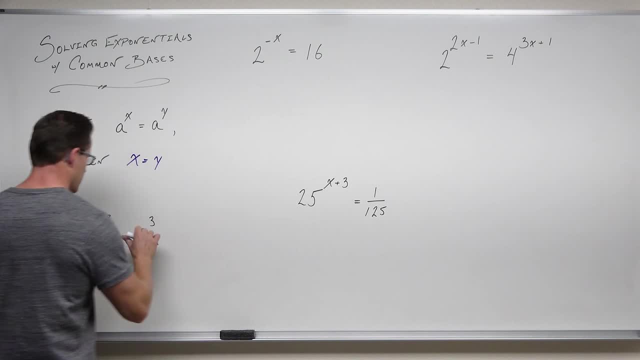 know Why don't we use a variable? And we can. So we'd say, hey, if two to the x- this thing, I don't know- equals two to the third, you don't know why don't we use a variable. 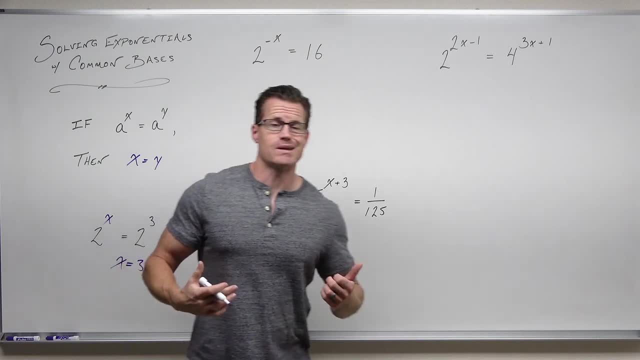 And we can. So we'd say: hey, if two to the x- this thing, I don't know- equals two to the third, then x would equal three. in this case, That's the only way to make this statement. true is if those exponents are the same, considering that our bases are the same. So we're going. 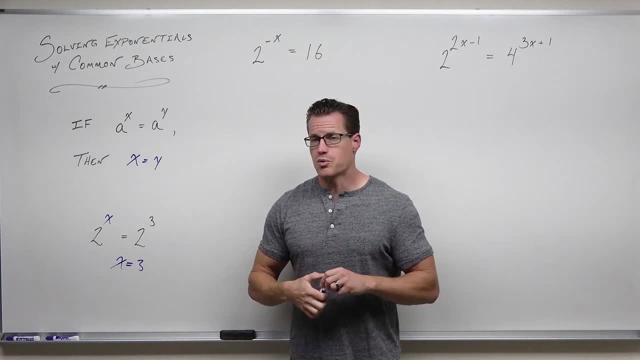 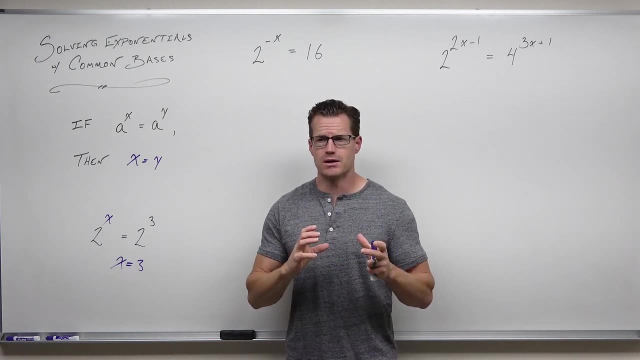 to use that technique for a few examples just illustrating this. You probably have seen something like this before. I'm going to show you some special situations where you need to know what to do with fractions. You need to know what to do with some quadratics. 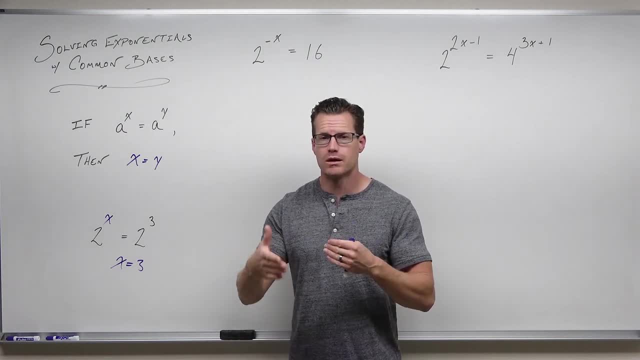 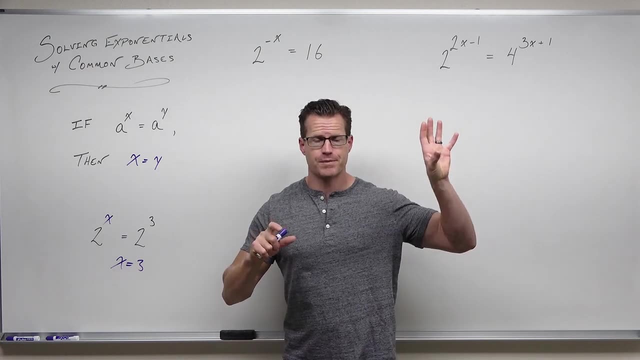 that are going to come out of these equations. but that's basically it. We're just digging a little bit deeper. So long story made hopefully shorter, is that with exponentials in general, you need their inverse, You need logarithms. But there's one situation where we can avoid all that, If we can make. 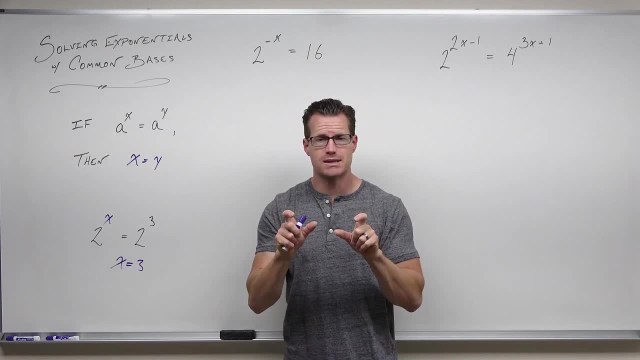 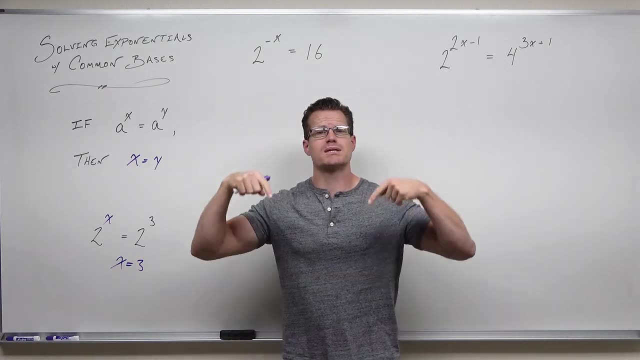 an equation, have all exponentials with common bases and we get one exponential on one side and another on the other side of an equation and we have the same base. then we can set our exponents equal. Let's practice. So how about two to the negative, x equals 16? You? 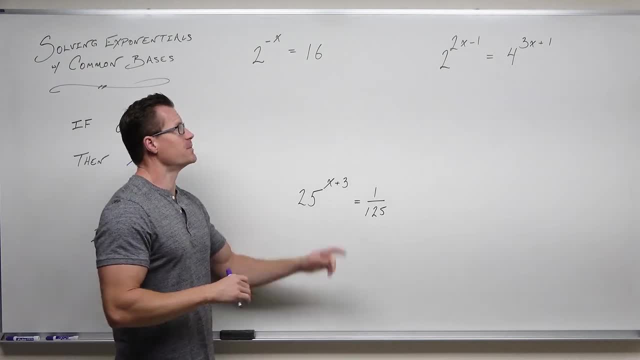 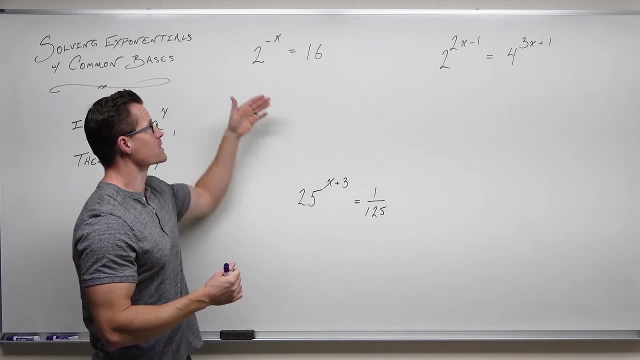 go. those don't have common bases, That's true. but sometimes we can manipulate this so that we get common bases. That's the only way We're going to get around this. We're going to get around not having to have logarithms to solve exponential equations. So two to 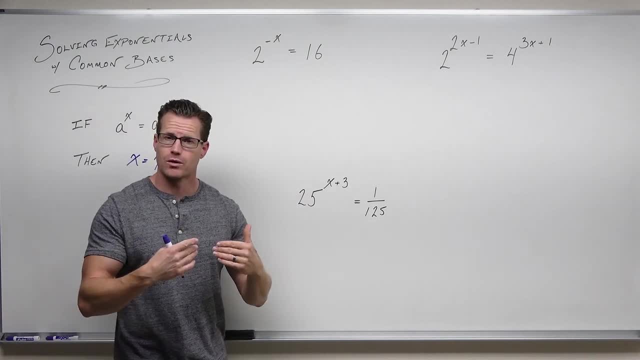 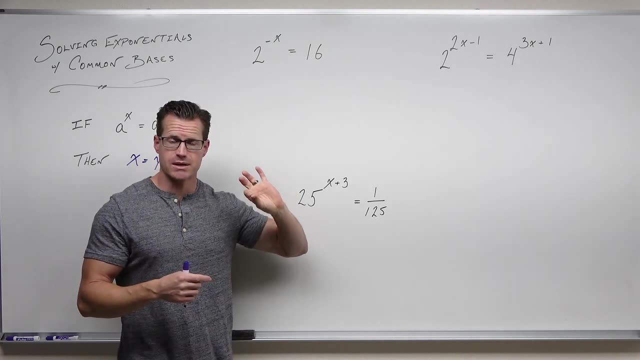 the negative x. two is a prime number. We can't get any lower than that, a sub base if you want to. but 16 is not prime. So we're going to think: can I write 16 as the same base raised to some power, the same base being two. So I know that two to the negative x. 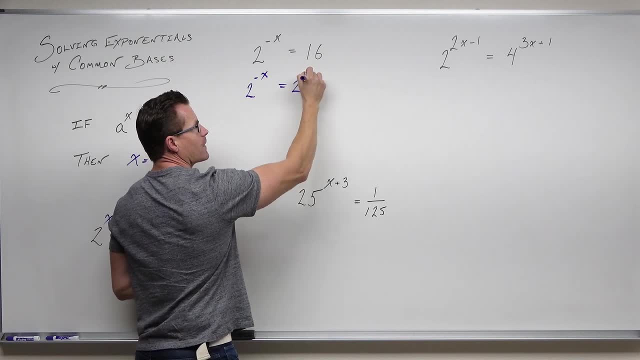 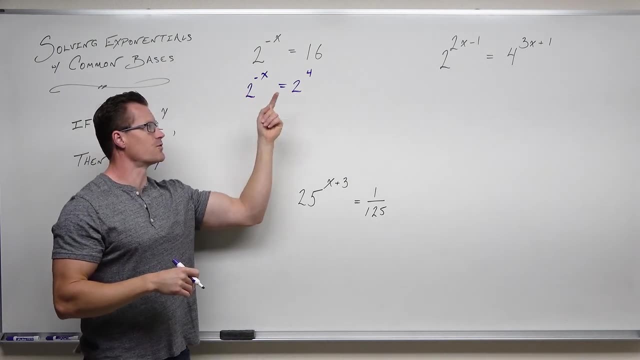 that looks really good. 16, we can write as two to the fourth power And we see right away that this is the case that we're talking about. If you can get an equation with common bases, then of x equals two to the fourth. the only way this is possibly equal is if our exponents are also. 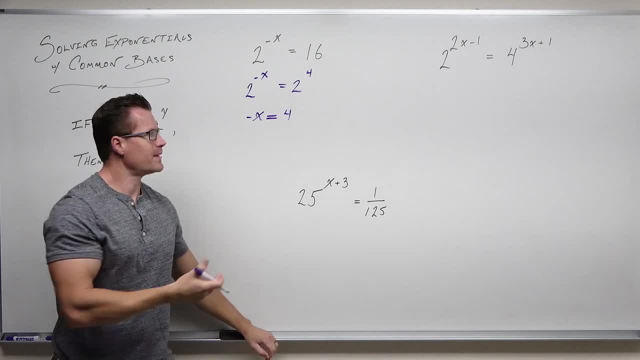 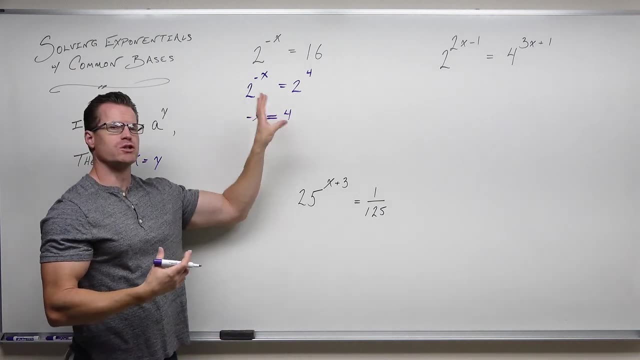 equal. Now, if our bases are not equal, then that goes off the table. We can't use that, And then we need logarithms to figure it out. But if your base is the same, the only way this equation is true is if your exponents are also equal. And so if you need to show this man, I have to show. 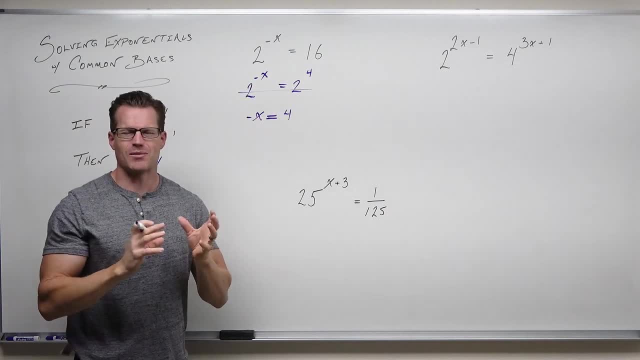 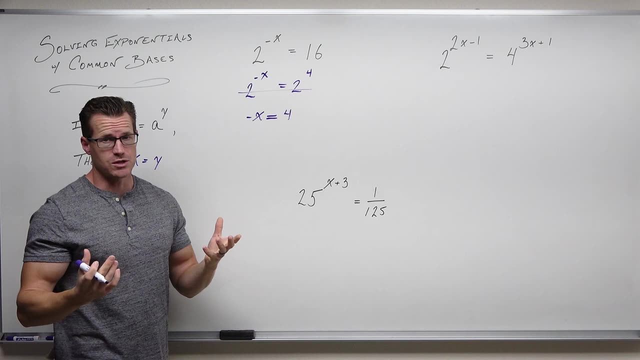 something. I just got to cross it out. You can do that, but it's not real math. It's just using this principle right here that says: base is the same, exponents also have to be the same, And then we can solve something that's much, much easier. Can you do some of this in your head? 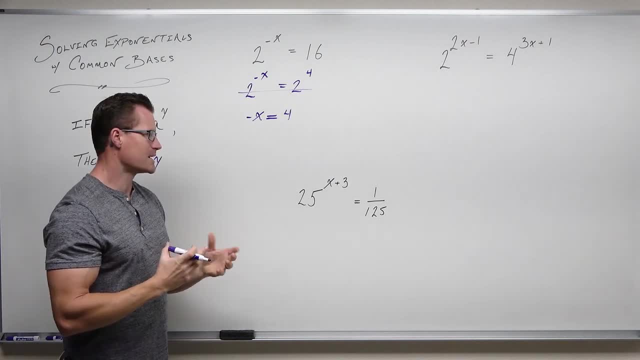 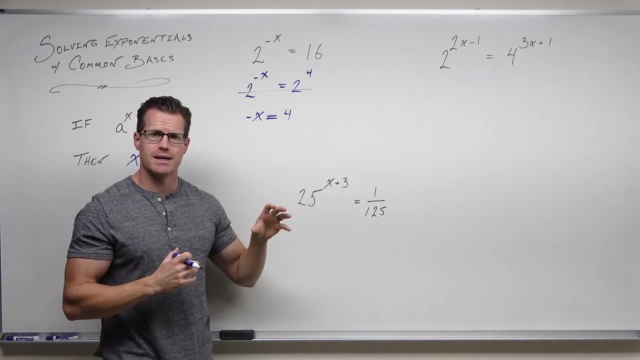 Yeah, yeah, but I'm going to really encourage you not to, because it's fairly difficult to do something like this in your head and it's really difficult to do something like that in your head, And so finding the common bases and setting your exponents equal is very useful for us. 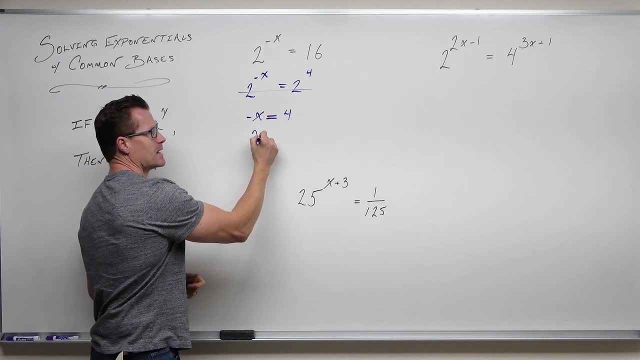 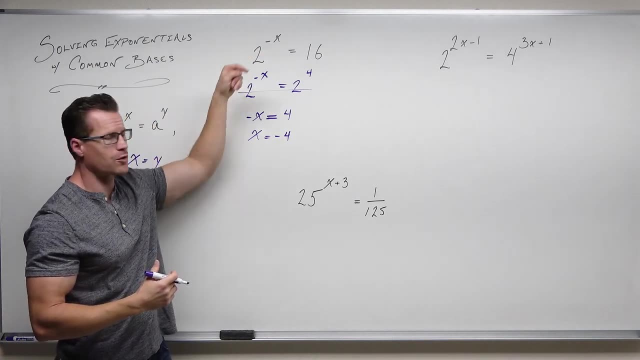 So cool, we got this. We set them equal. If we divide by negative one, we get this. Then we get x equals negative four, and that's actually true. Two to the negative negative fourth power or opposite negative fourth power is two to the fourth, and that is 16.. 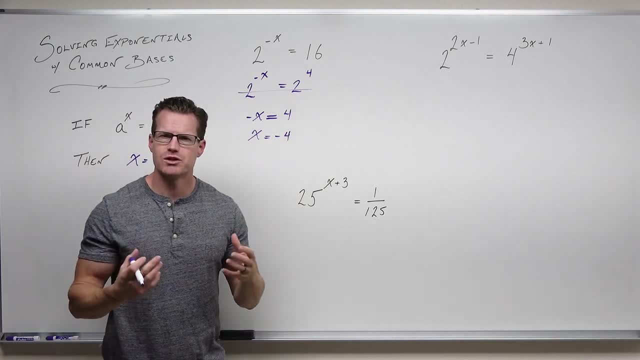 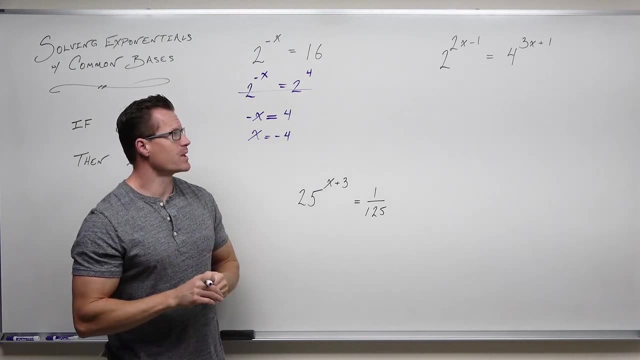 Let's go ahead, let's move over here, So we have another exponential equation. This is where we have one exponential expression equal to another. That's what we're looking for here. We notice that we have a base of two and a base of four. The first idea, the easiest idea, 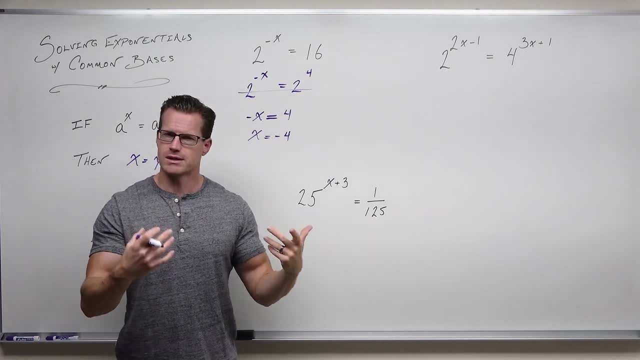 for us, so that we don't have to go down logarithms- is: let's check to see if we can get common bases Now, with a base of two being a prime number. we can't go any lower than that, But a. 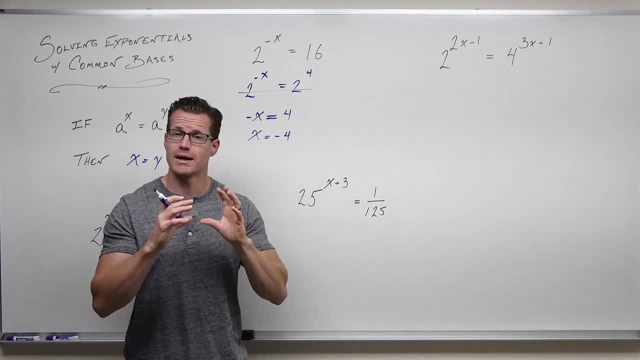 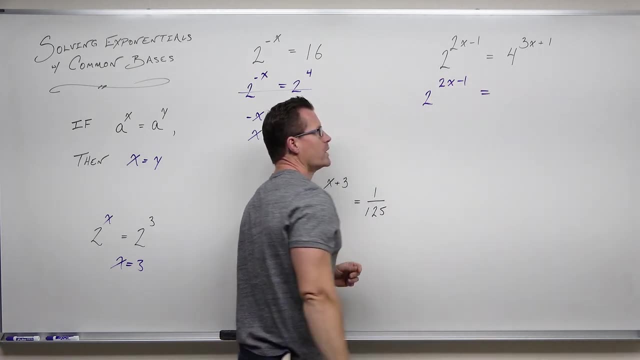 base of four that's different than two we can. So here's the way that I'd like you to do this, Number one: when you are going to take some sort of a base and write it as a different base, I need you to use parentheses. 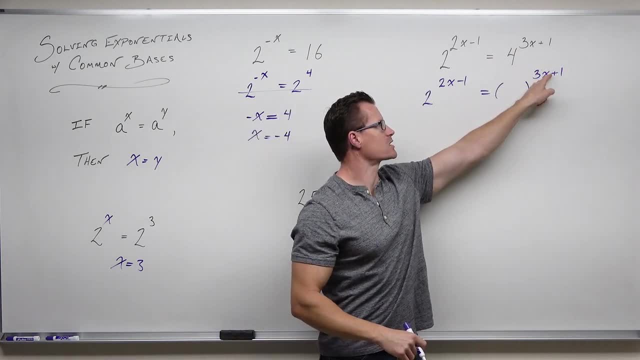 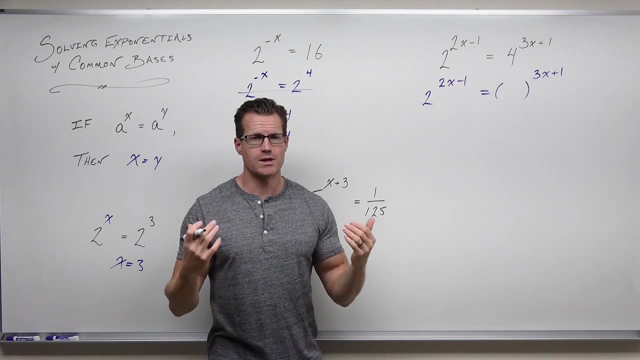 And I also really, really need you to write this x exponent exactly the same way. Most of the mistakes here, in these cases, they're not sign errors Only a few times, and sign errors aren't the major thing. One of the major things about: 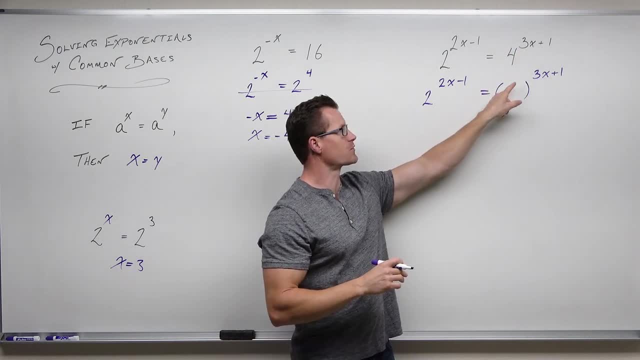 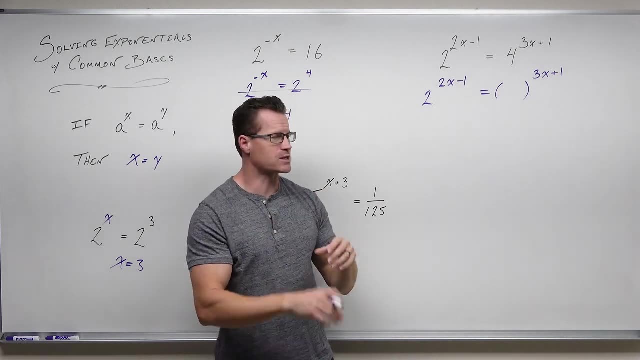 this is: students start losing exponents and students forget to distribute when you start changing bases, And those are two really, really important concepts. So the way that we solve that, the way we fix it, is: rewrite your base in parentheses, but then also do not forget to 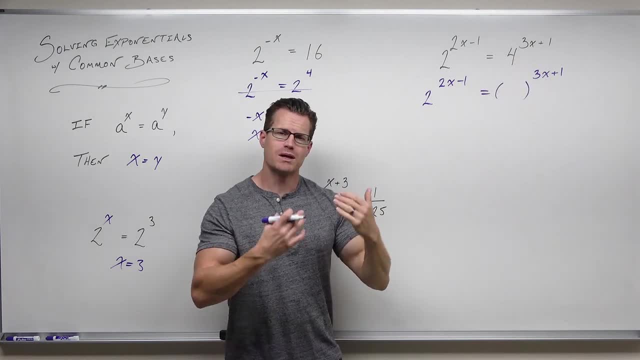 write your exponents. So I'm writing my exponent first, so I don't have to do that. So I'm going to forget it. When we get too wrapped up in changing this, we tend to forget that, So write it first. 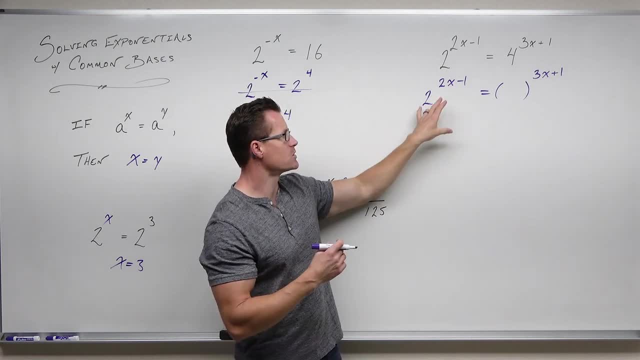 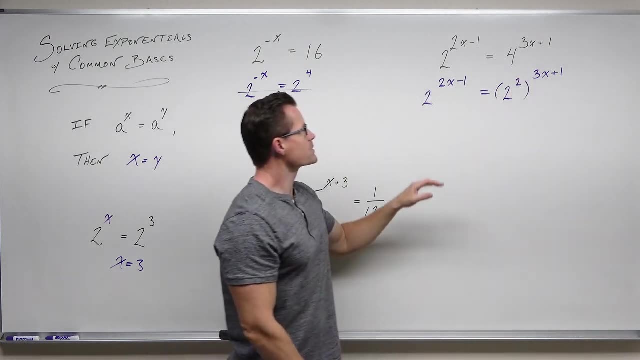 And then look at the four, Look at your base. Let's try to write this as two, the base we want to some power. I know that four is two squared. So this says two to the two x minus one. That's what we have. This says this right here, says: 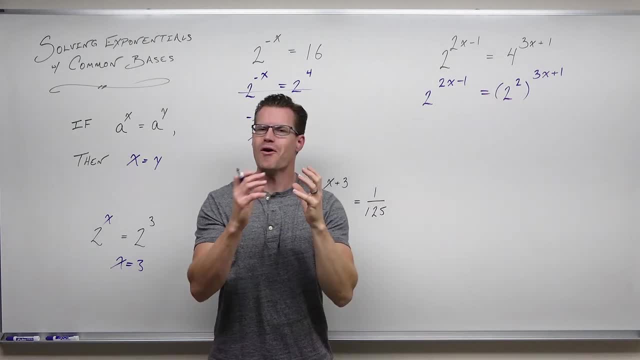 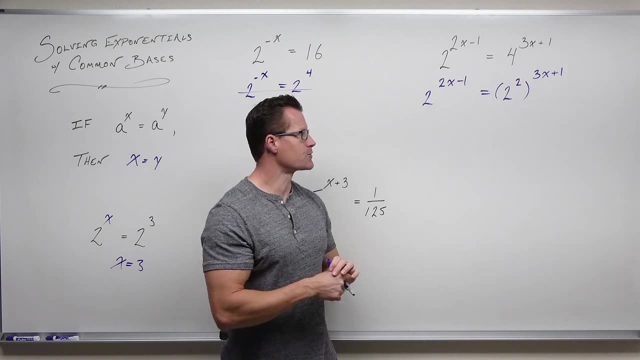 four to the three, x plus one. We're just writing it as two squared. And then we all know, we all know that when we take an exponent to an exponent, we multiply it. Well, what that means for us is that when we have two to the second, 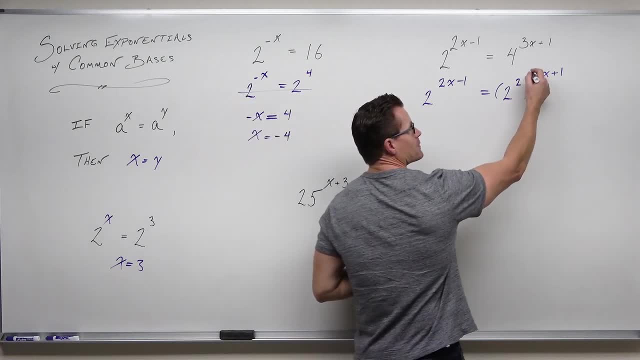 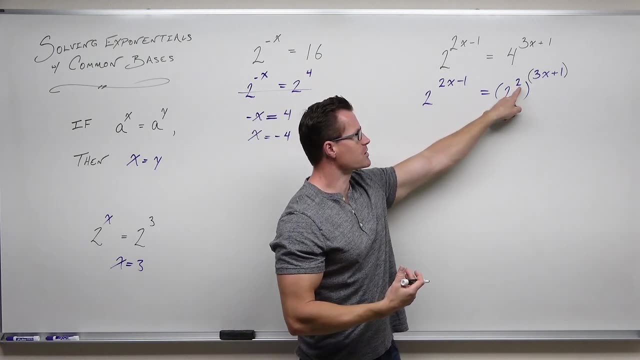 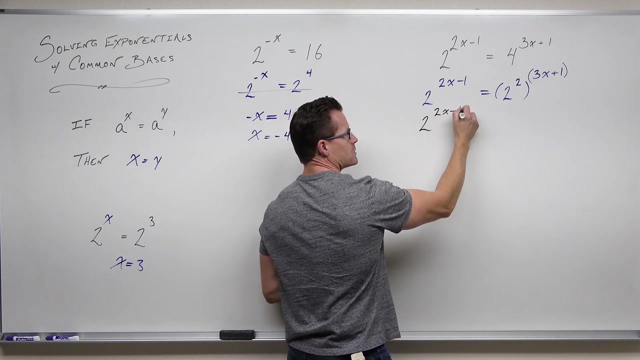 raised to three x plus one. we're going to have to think of this in parentheses. We're going to have to think of this as two. That's our exponent, not our base. Our exponent raised to another exponent. You need to distribute that So sure we get this two to the two x minus one, That's. 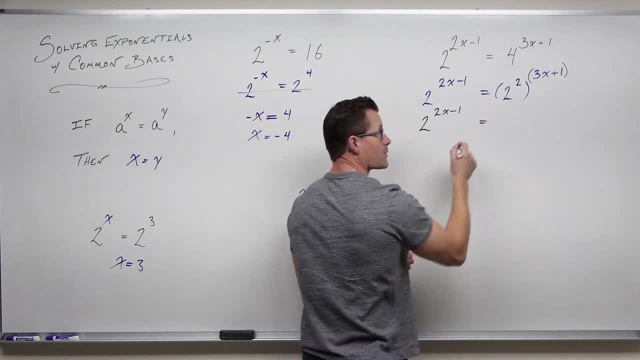 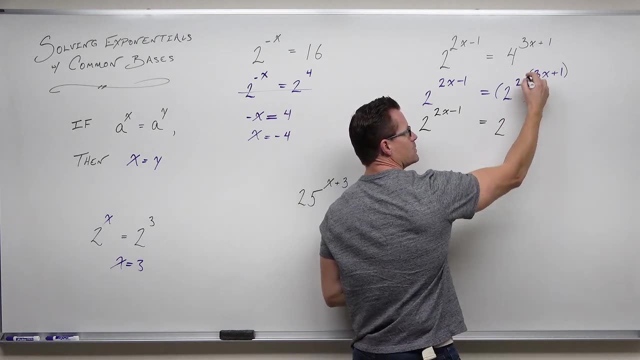 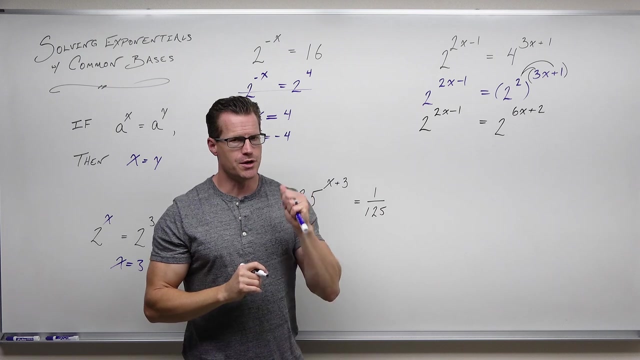 totally fine, We did nothing that would change the base. We didn't have to. But on the right-hand side we've got two to the two times, essentially times three x plus one, That is two to the six x plus two, not six x plus one. We must distribute that. It's an exponent times an. 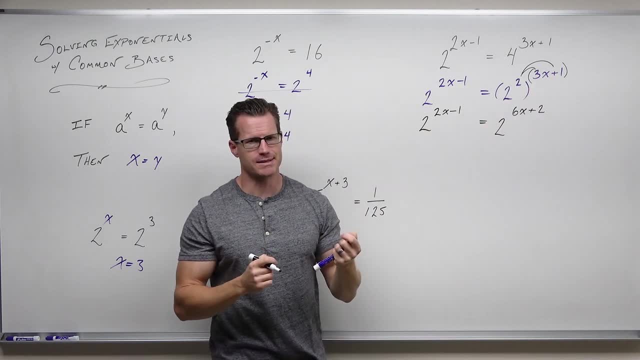 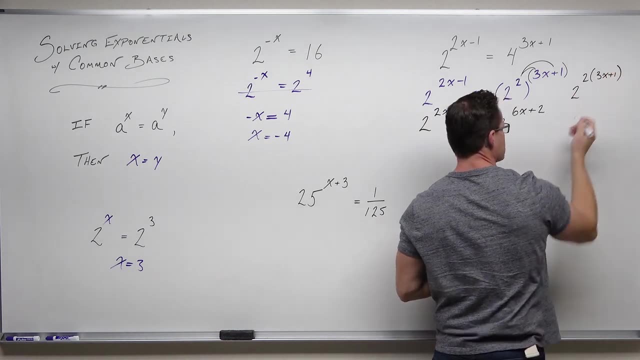 exponent And because this is our entire exponent, distribution is necessary. If you need to write this as an extra step, that's fine, That's taking an exponent, times an exponent, That's taking an exponent, And then you can really see the distribution. But once we've done that, once we've 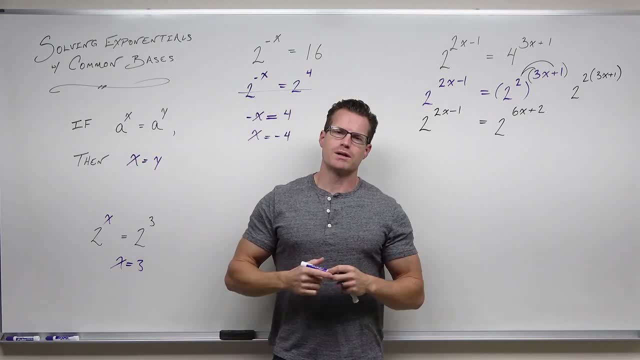 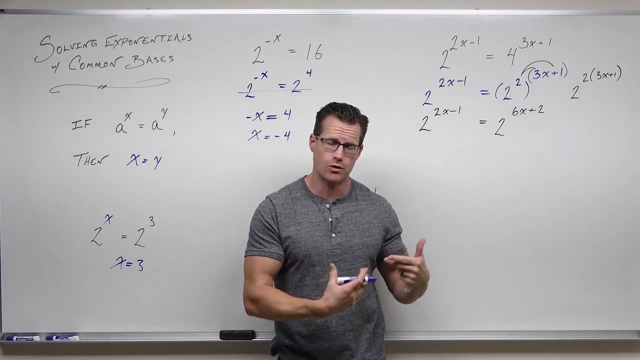 taken and found common bases. this principle takes over and says: hey, if your bases are the same in an equation, then your exponents are also equal. They have to be in order to make this equation true or make it equal. That also says that if you have more than two exponentials, you're going to 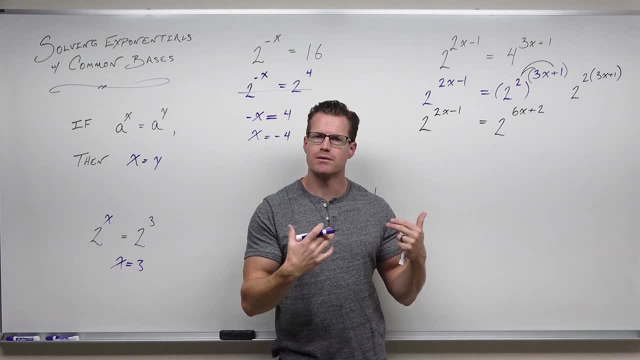 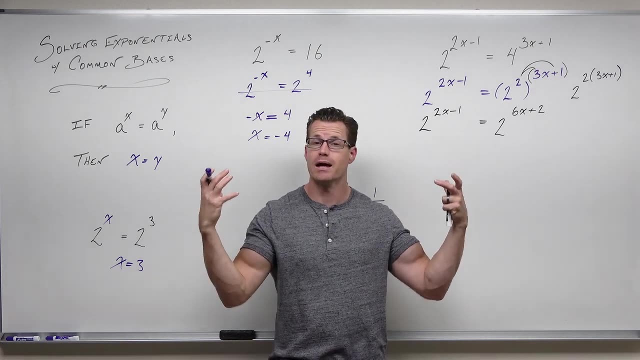 have to have some way to combine them, And if you can't, then we need another technique for that. This only works if you have one exponential expression equal to one exponential expression, and then you can set your exponents equal. Barring that very, very special case we need. 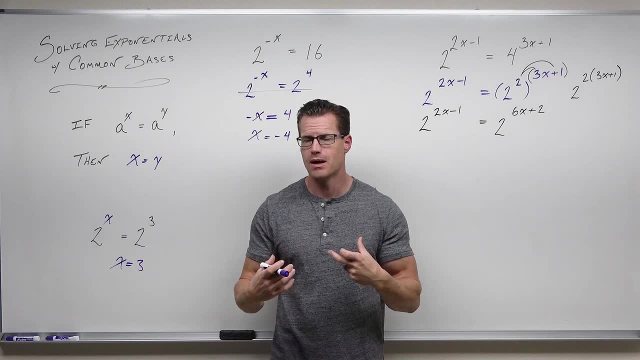 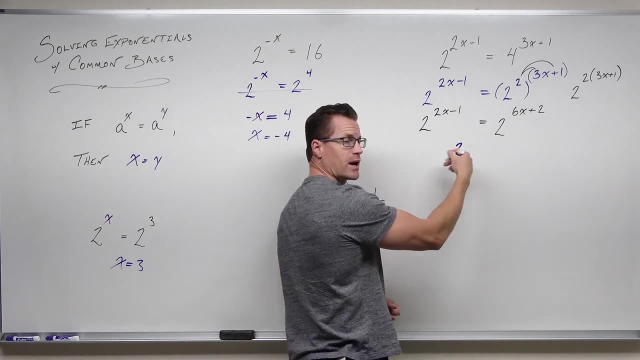 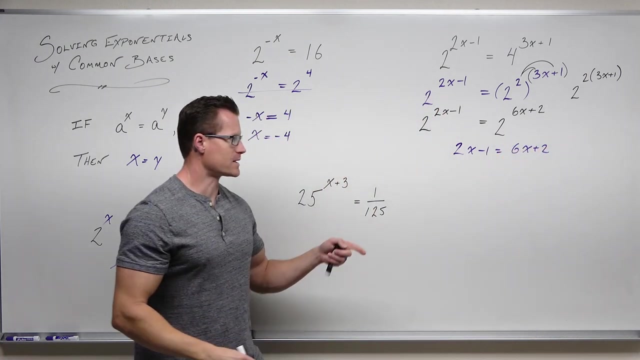 other techniques for that. If our bases cannot possibly be the same, then we need logarithms for that. So once we have it, we say all right now that our bases are the same. we know the only way that's true is if our exponents are also the same, And this gives us something really nice to solve. 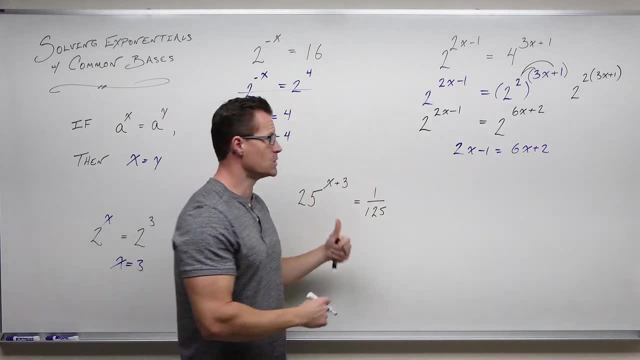 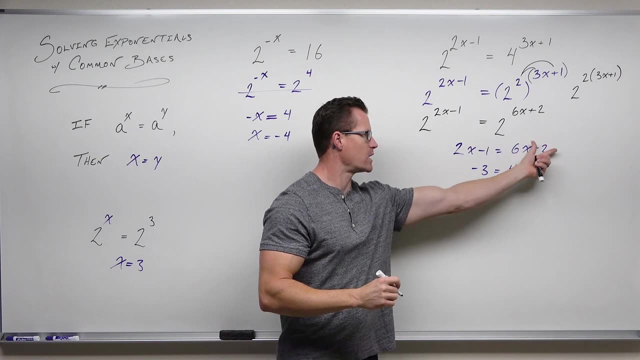 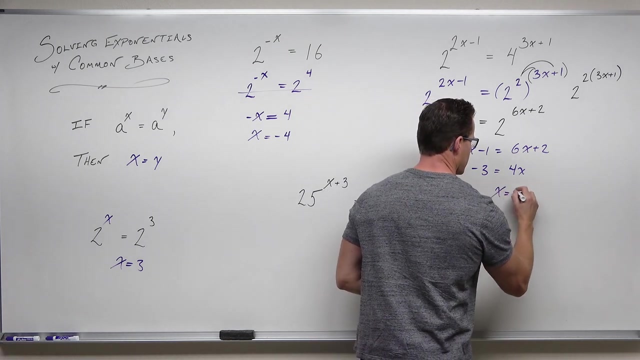 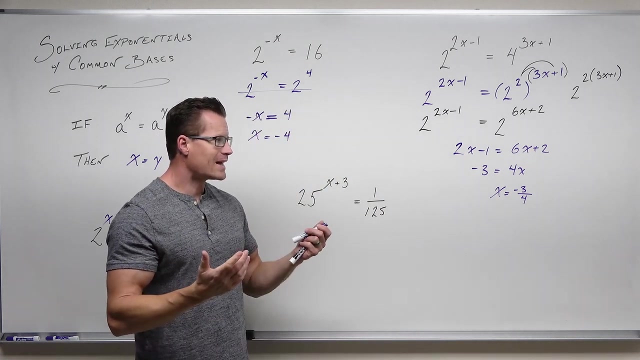 We're going to subtract two x and we're going to subtract two. So subtracting two x from both sides gives us four x. Subtracting two from both sides gives us negative one minus two is negative three. If we divide by four x equals negative three-fourths. So that's about what we're doing here. I'm going to start going. 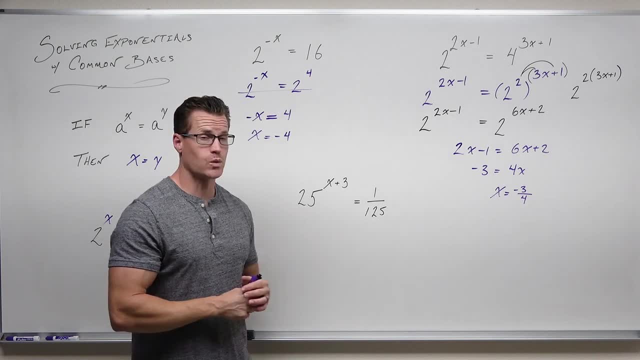 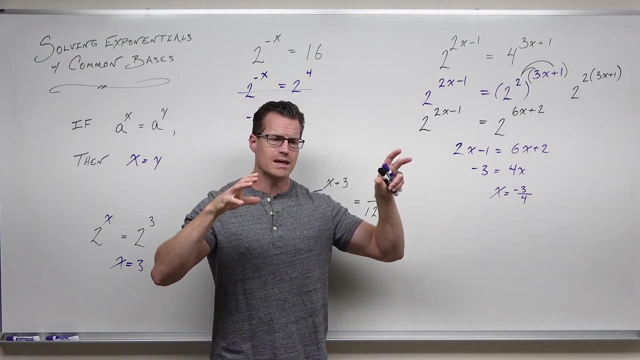 into some special situations that we can get like with fractions, what to do with those. But that's essentially what we're doing: We're finding common bases and set our exponents equal. When we get further on into this, when we get to where, what happens if this is a two and that's a? 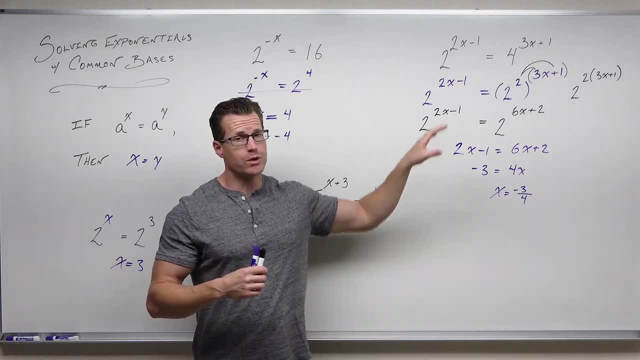 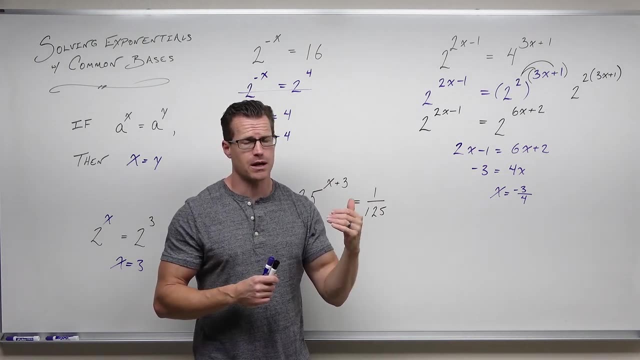 five, can you possibly get a common base? No, and we would not try any of this stuff. We'd go directly to the inverse of an exponential. Remember, I'm trying to build out in your head what that's going to be. Okay, we haven't got there yet, but I'm trying to build out that if these are not able, 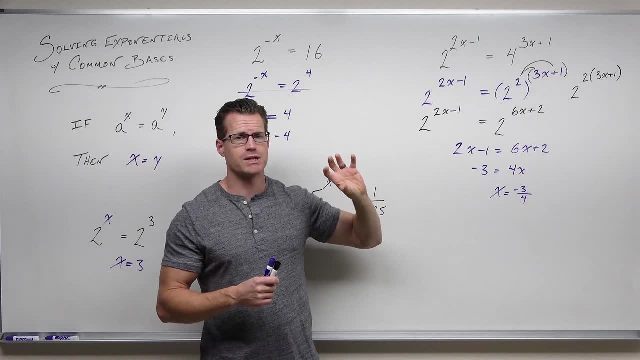 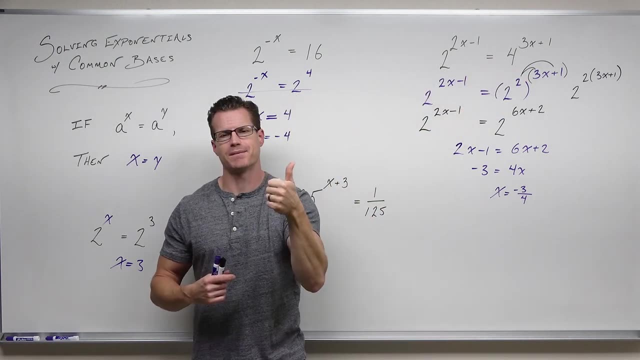 to get common bases, you're going to go directly to the inverse of an exponential, which is a logarithm. So right now, this is a real special case. If you can get these to be the same base, cool, do it. It's really easy, or easier than logarithms. but if you can't, you're going to. 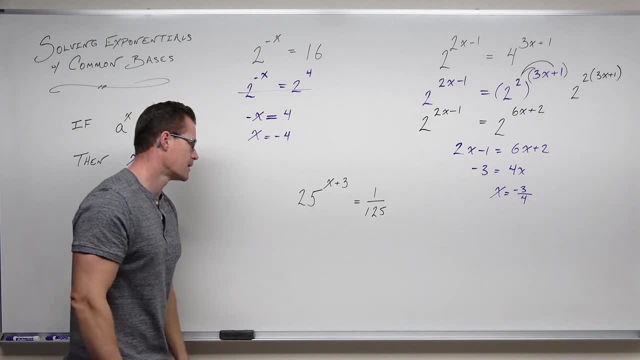 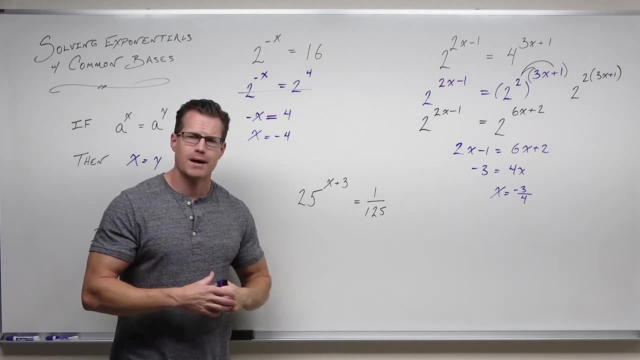 need the inverse. You're going to need logarithms for exponentials. All right, let's move on. If you ever get fractions and you're trying to do this technique, what we're going to do right away is we're going to get common bases, but for every fraction that you have, make sure that you write. 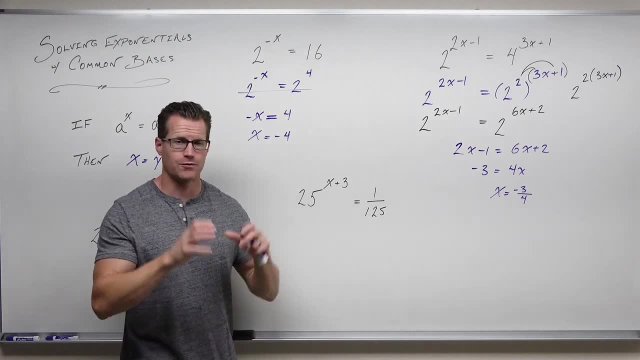 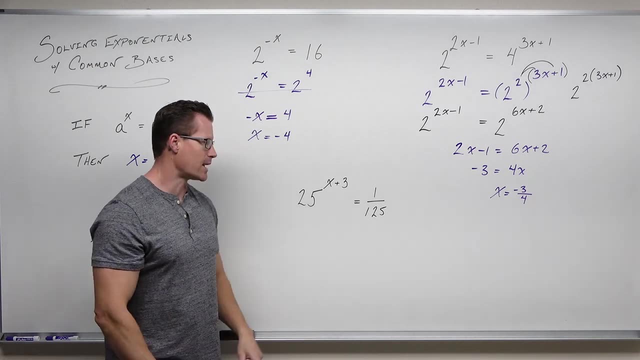 that as a negative exponent. It's going to save you so much time and a lot of headaches. So fractions are going to equal negative exponents for these exponential expressions and exponential functions. So let's take a look at it. We have 25 and we have something with a 125.. 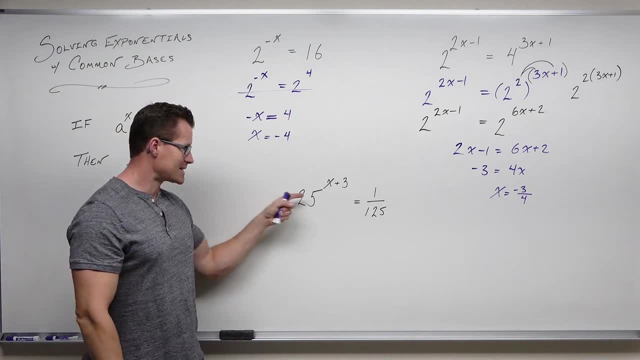 I go: man, that's really lousy. I don't like that. That's nasty. These are not the same. Let's try to look at these under this lens and say: let's try to get some common bases out of it. 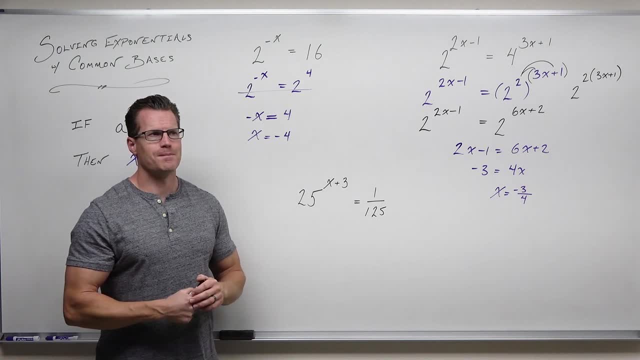 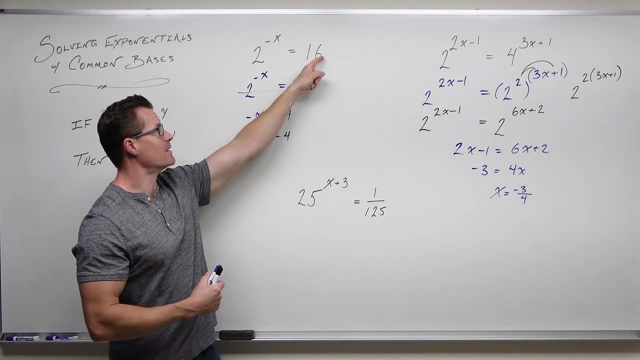 If I think about 25 and I think about 125, try to write the bigger one as an exponent of the smaller one. So here we were able to write 16 as 2 to some power. That was 2.. 4 as 2 to some power. 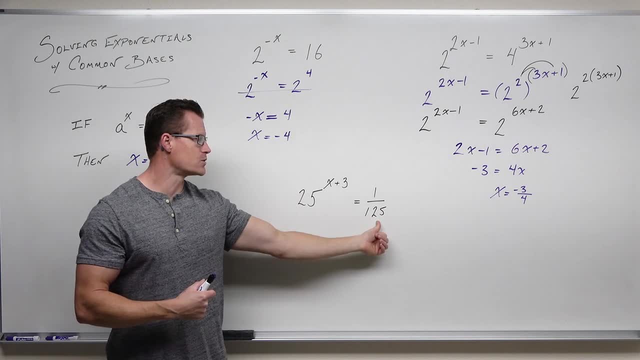 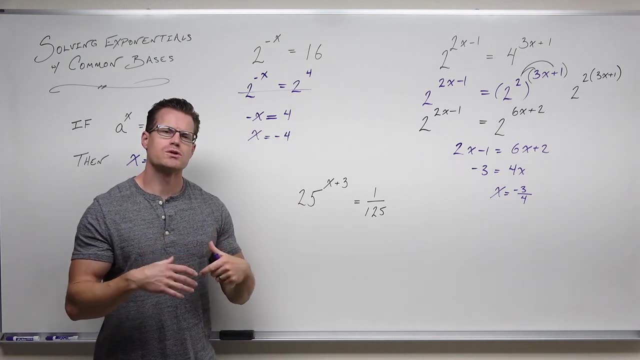 and 1 as an exponent of the smaller. Can I write 125 as a power of 25?? Well, no, I could like. 625 is 25 squared, So no. What that also means is this a little caveat here: You don't always. 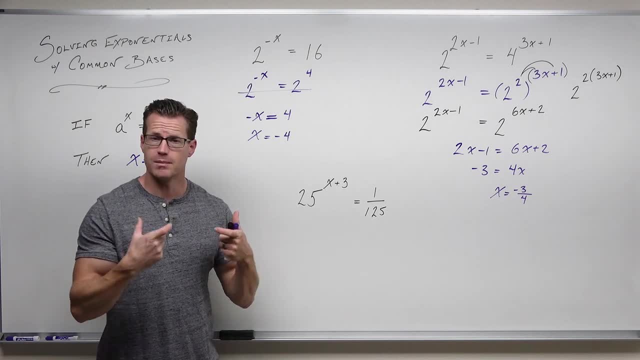 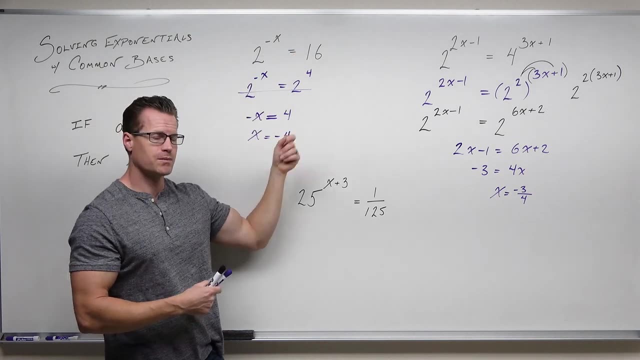 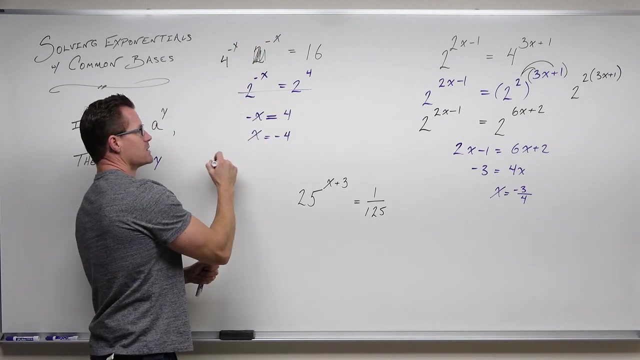 necessarily need to get down to the smallest prime number base. Sometimes you don't have to do that. If this had been 4, then I wouldn't have to break both of them down to 2.. If this had been 4, and not 2,, then I could have said: this is 4 to the negative x and 16 would be 4 squared, And I. 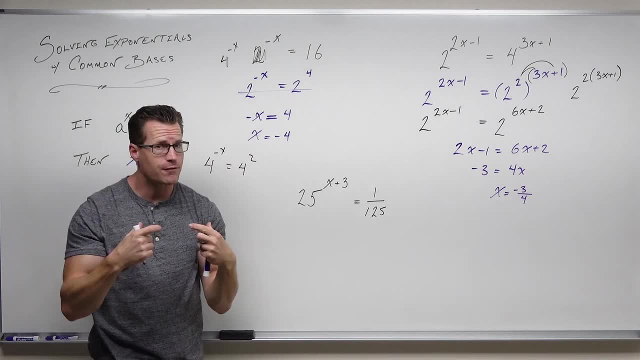 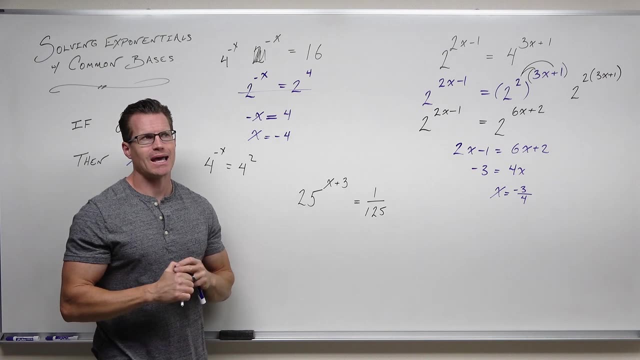 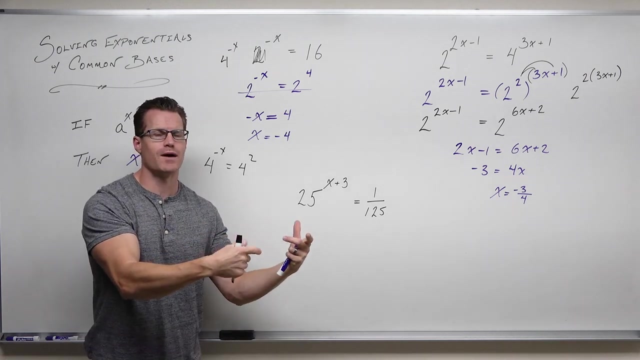 would set those equal to one another. You don't always necessarily have to get down to a prime number base to make this work. Just any common base will do. In this case we go. well, I can't really write 125 as 25 to a power, but I could write both 25 and 125 as 5 to some power. So we're 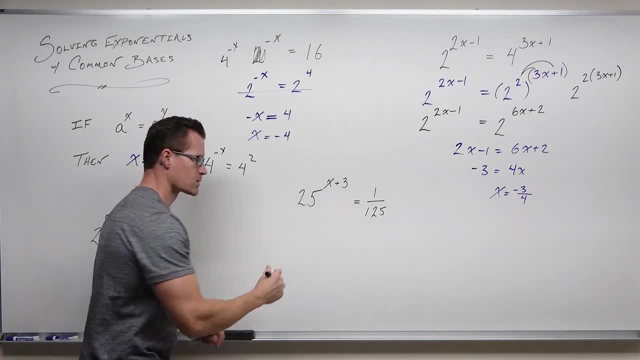 going to go through that. We're going to say, all right, 25 to the negative x and I'm going to 25 to the x plus 3.. I'm going to think I'm rewriting my base. I'm going to number one. 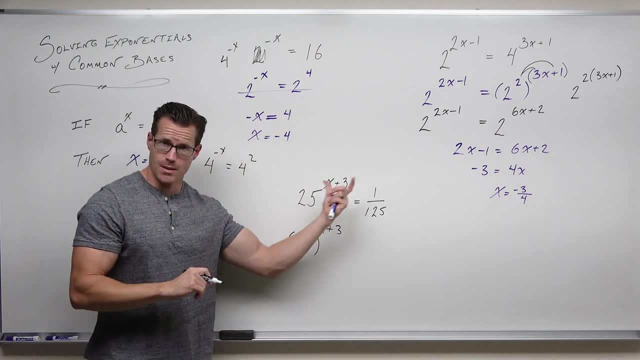 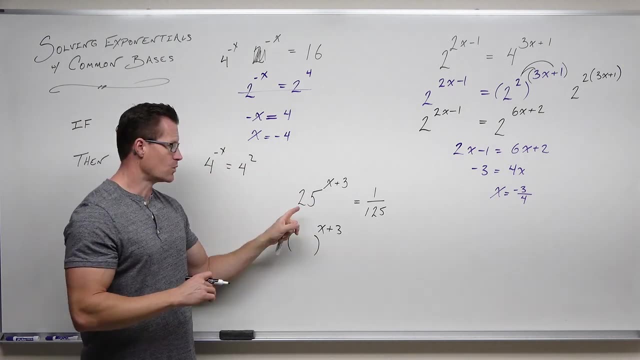 first show that I have my same exponent. I'm going to write that right there so I don't forget it, I don't lose it, I'm taking my 25, and I'm thinking in my head: let's find a common base between 125. 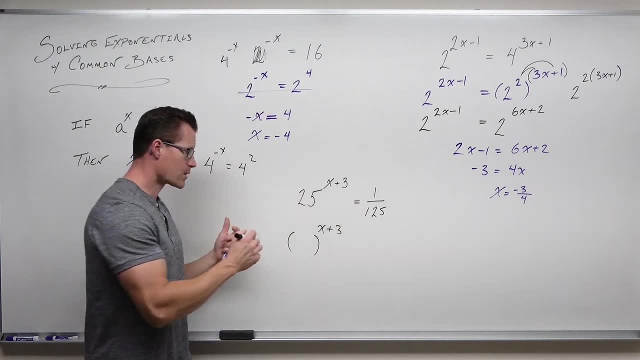 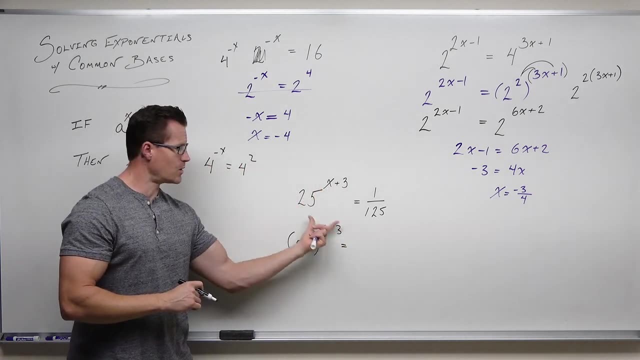 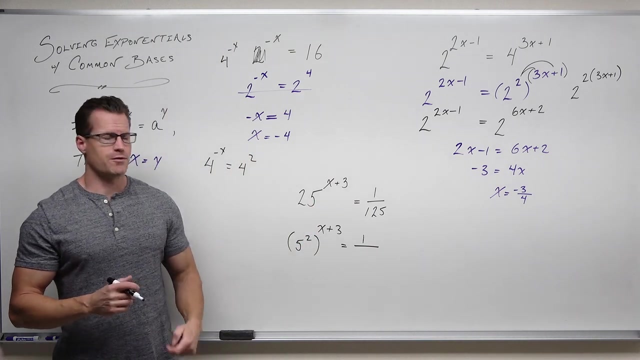 and 25, and that would be a power 5.. So I'm going to write this as 5 squared. This means the same thing. Here's my same exponent. Here's 25 written as 5 squared. Where could we go? I'm going to do the same thing with 125.. I'm going to think: how is 125 a power? 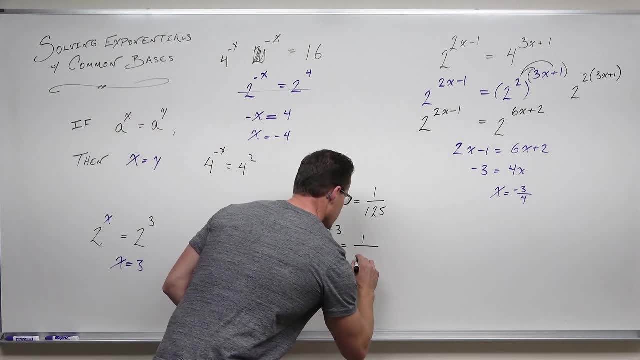 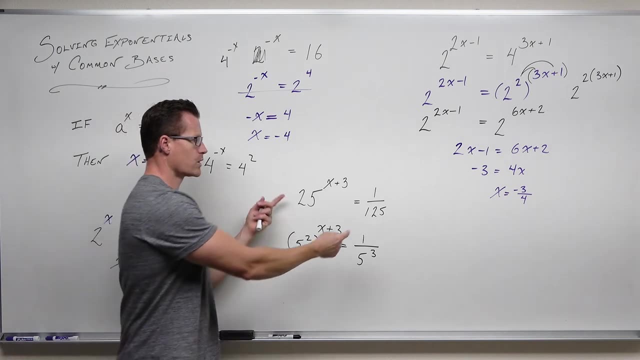 of 5?? Well, it's 5 to the third power. So we've just rewritten this with a common base, and that's the idea. Take a look at what your bases are. This is the base. Think of fractions as something over. 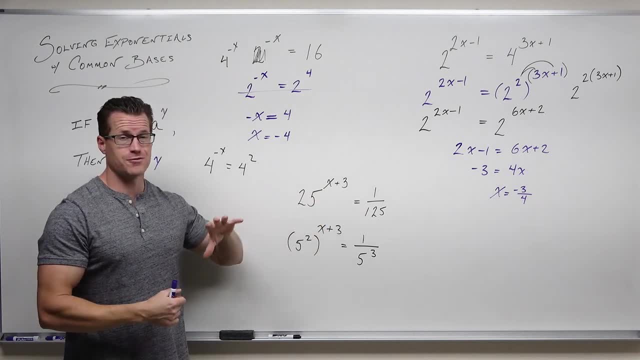 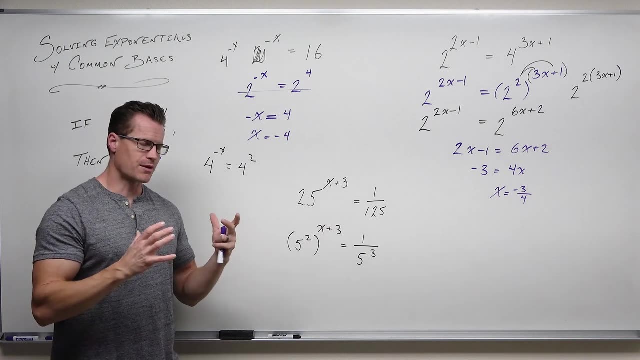 the base that you want. So 25 and 125, both have a base of 5 somehow: 5 to the second power, 5 to the third power. And now with every negative exponent, or sorry, with every fraction that you get after you've. 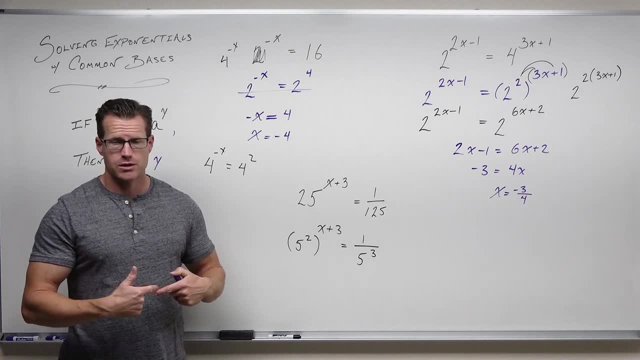 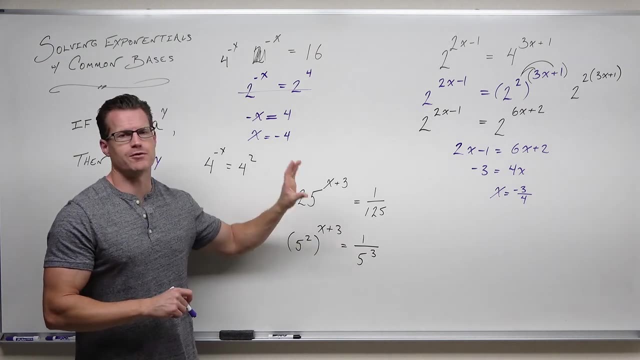 written that as an exponent, write them as a negative exponent. So we can always, on one fraction, change a power to a negative exponent by moving it from a numerator to a denominator or from a denominator to a numerator. So we can do that here too. 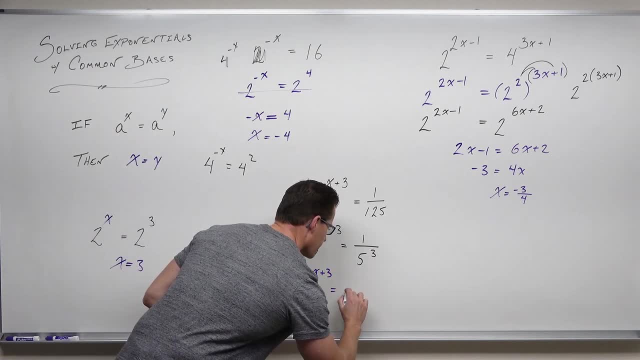 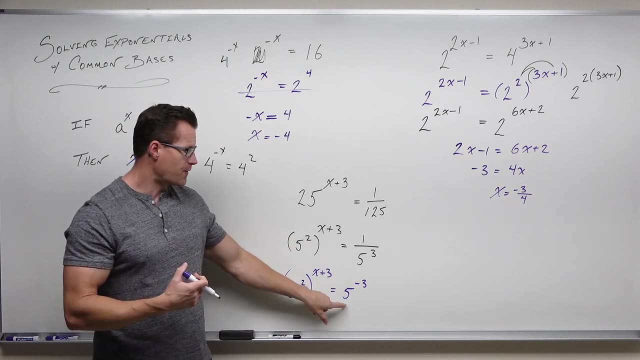 So, instead of 1 over 5 to the third, 5 to the negative third power is 1 over 5 to the positive third power. We can think of this as 5 to the negative third power. Consider that this is the same thing: 5 to the negative. 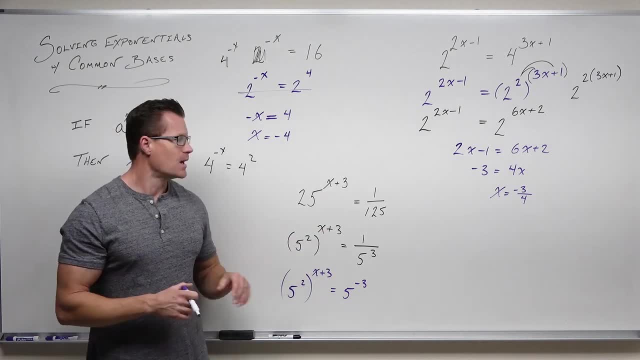 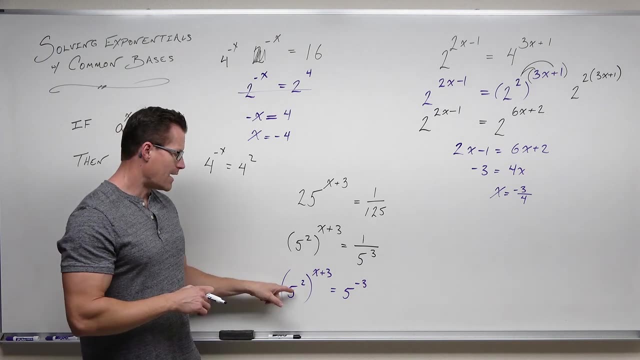 third power is 1 over 5 to the positive third power. So again, if you see fractions, sure get a common base, but then write them as a negative exponent. It makes everything a lot nicer. We're going to see it right now, after we take care of the side. So 5 to the negative third power. 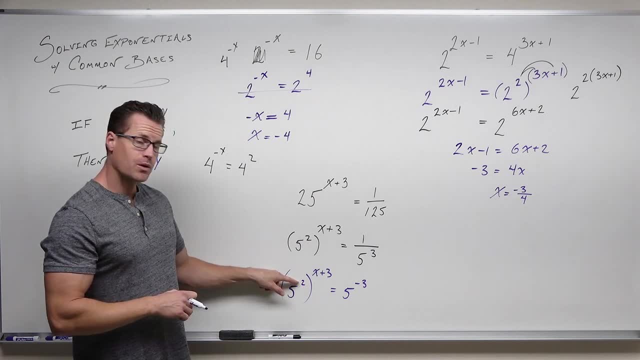 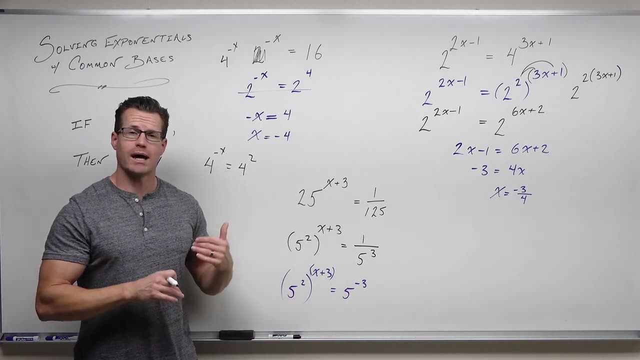 that's good to go. On the left-hand side we have an exponent raised to another exponent. If you want to write this out like I did over there- an extra step- that's fine. You don't have to, We can think. 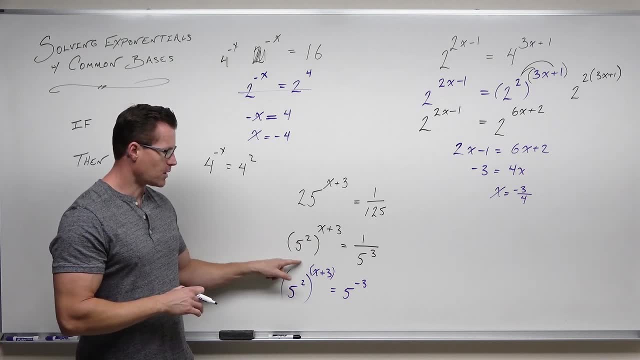 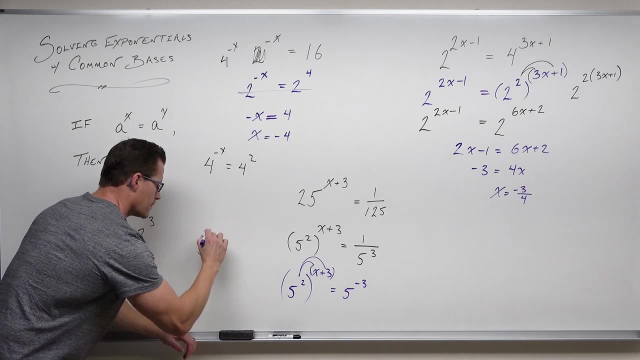 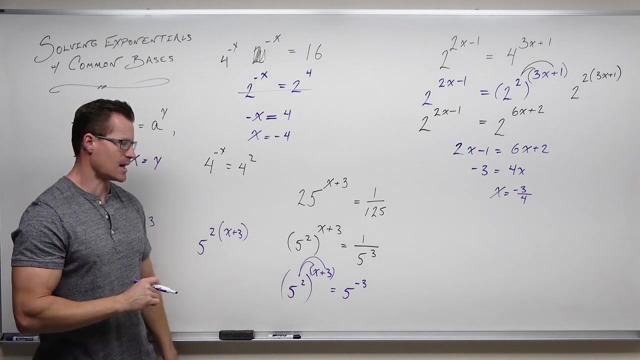 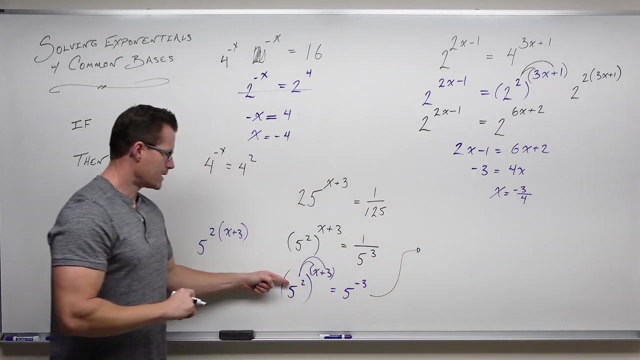 about this as distribution. This would be 2x plus 6, but we do absolutely need to distribute. This is really what we're doing: taking an exponent times another exponent and then that causes us to have to distribute. So we're going to get this 5 to the 2x plus 6. 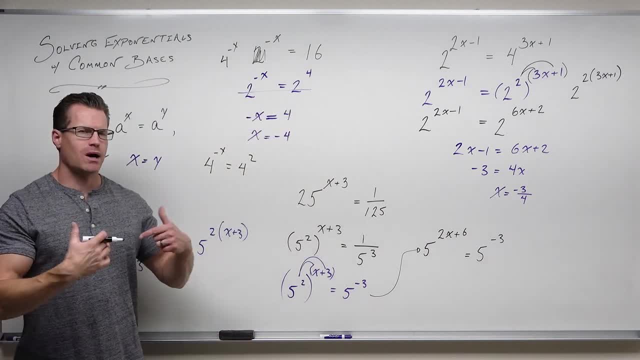 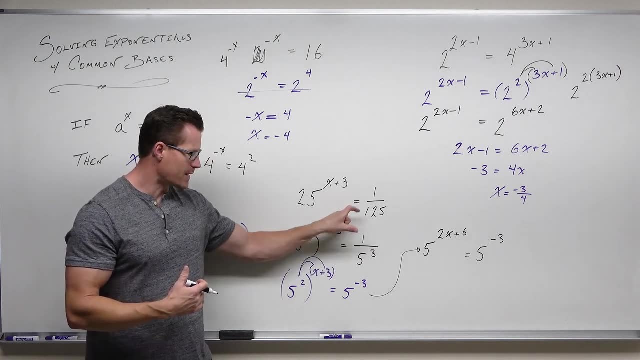 equals 5 to the negative third power. Now we see why we use that negative exponent. If we hadn't, it's really awkward to understand what's going on here with the denominator. So if we write that as 5 to the negative third power, we say, oh, this is perfect, This is exactly. 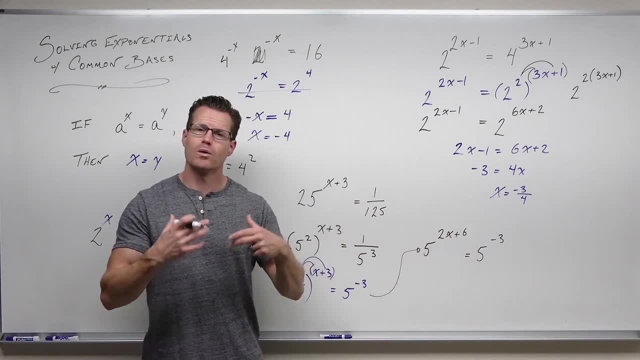 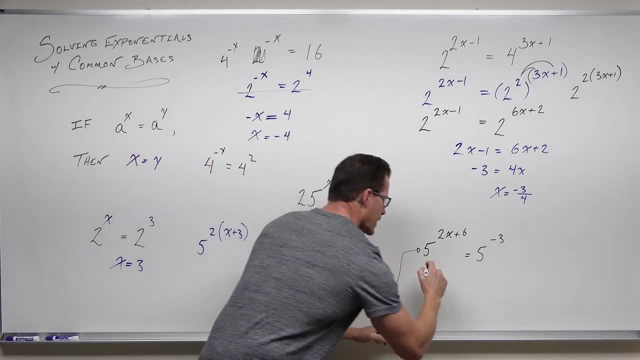 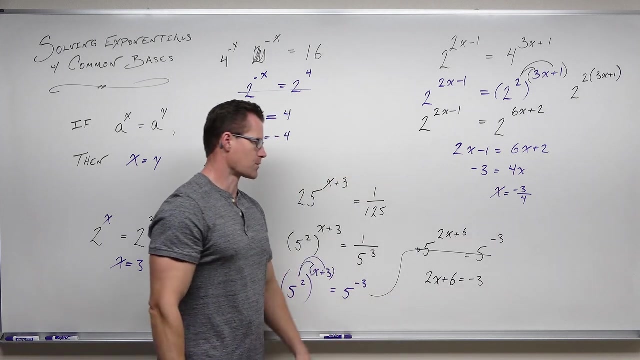 what we want. We've got 5 here, We've got the same base, And the only way this equation can possibly be true is if we have common bases, we also have equal exponents. So our 2x plus 6 equals negative 3. It gives us something really nice to solve, If we do solve that. 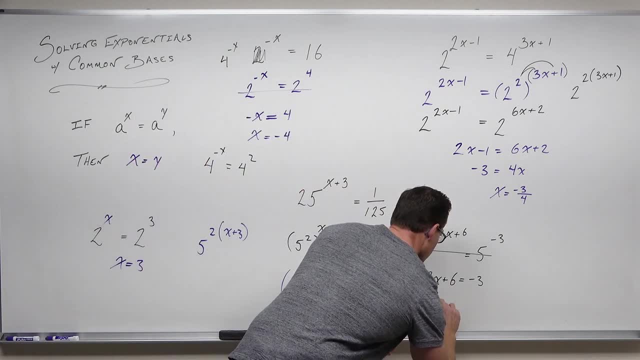 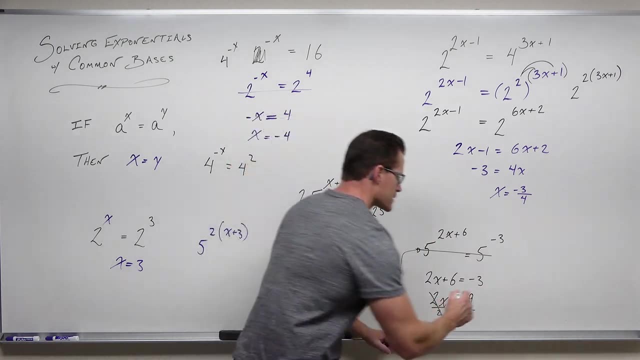 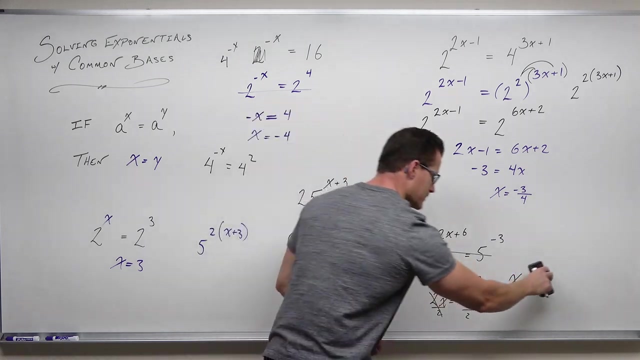 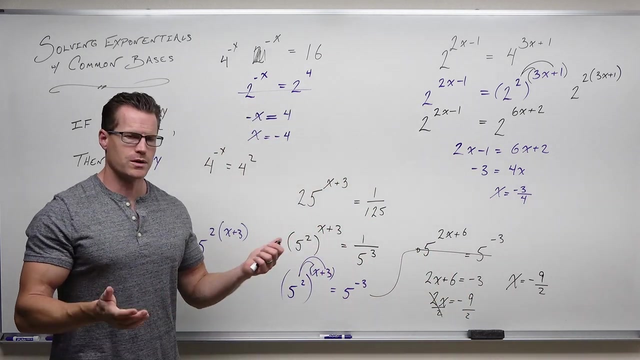 we're going to subtract 6 and divide it by 2.. We get x equals negative 2 ninths. No, we don't. Negative 9 1⁄2.. You can put negative 4 1⁄2 if you really want to, but it's fine to leave that. 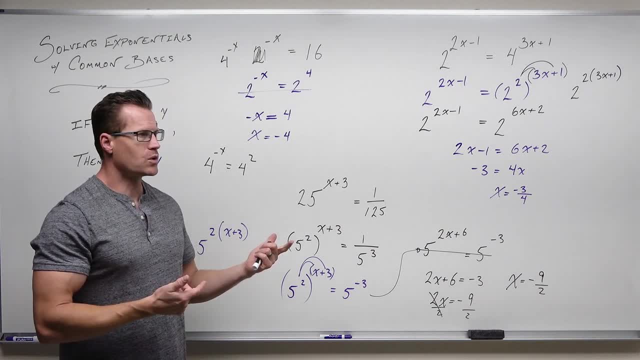 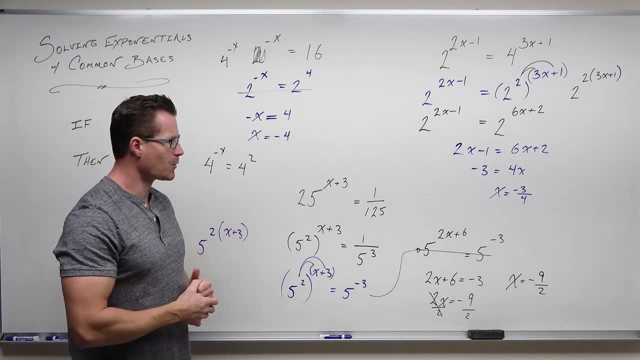 as an improper fraction. In fact, that would show you that this is going to be some sort of a radical expression anyhow with our exponentials, So I hope that that makes sense to you. I really want to make sure that you understand that the concept of get. 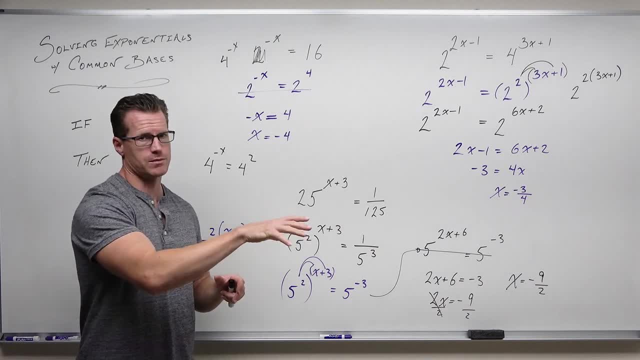 your bases the same, and if you don't have that, you will need logarithms. It's a must. So here, cool yeah, we've got 5 squared. 5 to the third, but that was a special case. 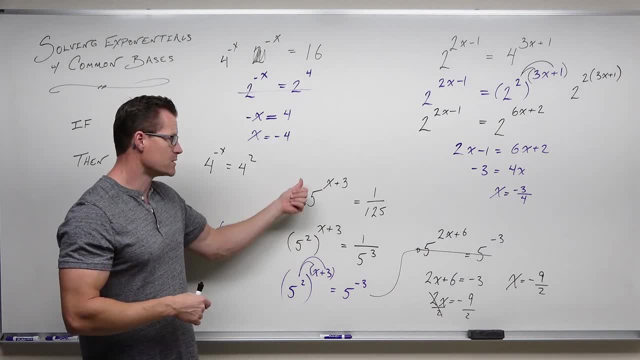 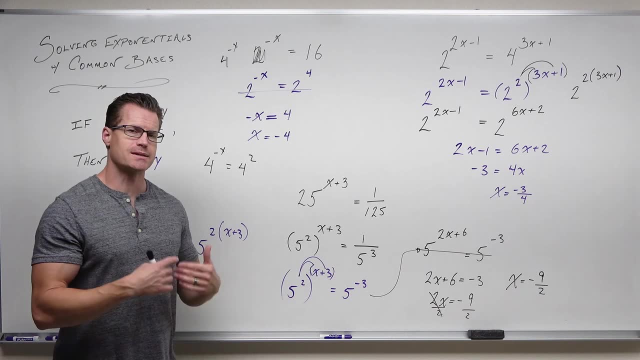 If that had been 27,. this won't work. We could have done 3 to the third and 5 to the third, but those would not be the same base And when we get down to here we get stuck. so we'll need something else beside that. 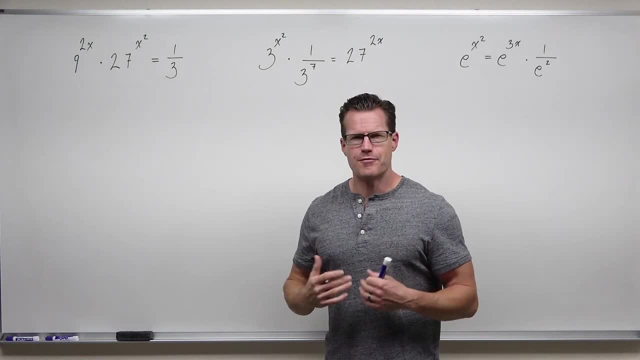 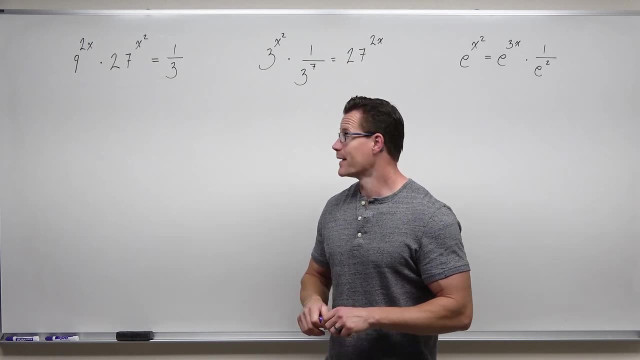 All right, we're going to work our way through three more examples. a little bit tougher, a little little bit more in this than we had in the first few examples, so a little bit more complicated. really, Let's just remember our goals. So our goal is: whenever you see an exponential equation, 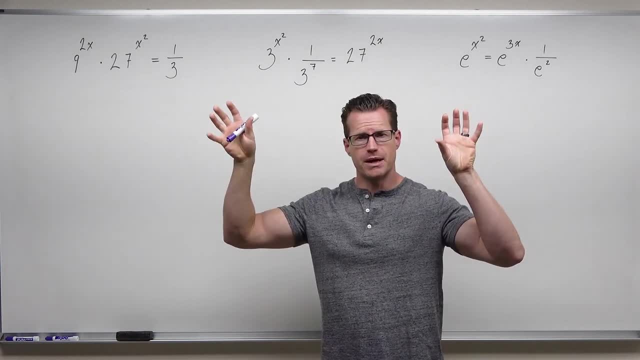 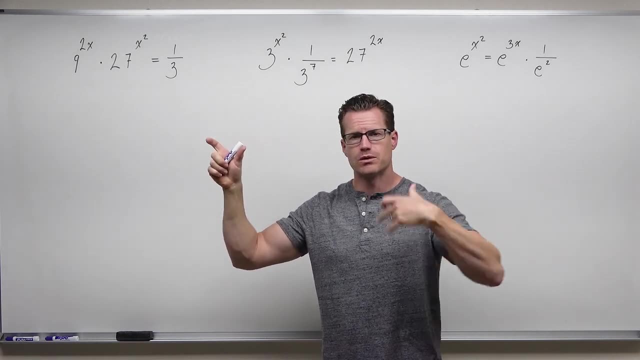 I'm trying to build these categories in your head. If you can find common bases, great. Set your exponents equal. but you have to have a very special case there. You have to be able to get one exponential equal to another, one with the same exact base, and then set your exponents equal. 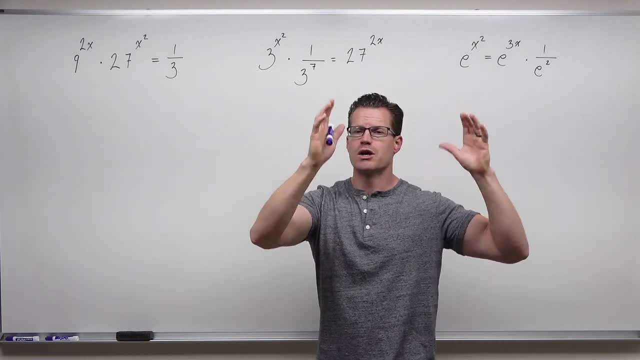 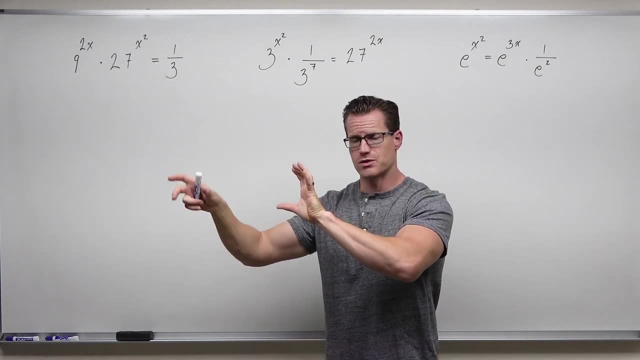 If you do not have that, the second category is you're going to have to use logarithms somehow. So in your head right now, common bases, great exponents equal, and you have to have two exponentials, one on one side, one on the other. That's it. But if that's not the case, logarithms. 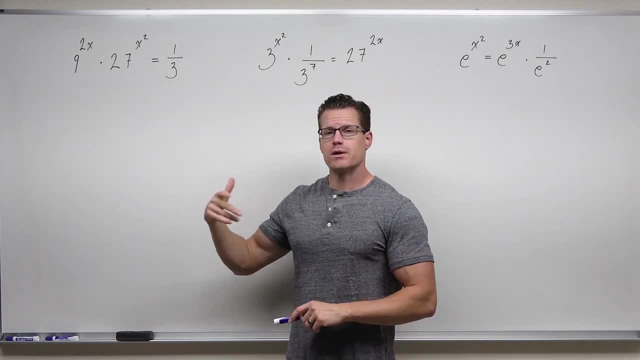 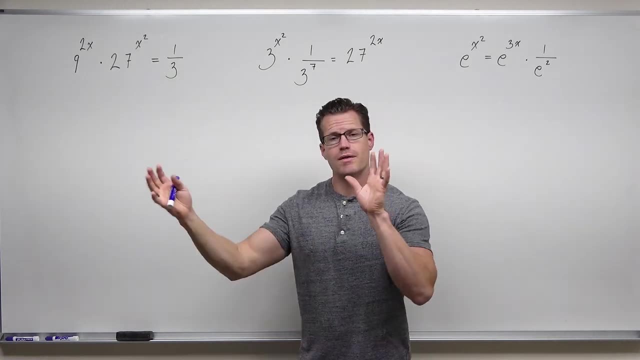 We haven't made it there yet, So let's take a look at it. Are we going to be able to write all three of these exponentials as one common base? If that's true, then we can start combining our exponentials, and that's great. That's not a problem. 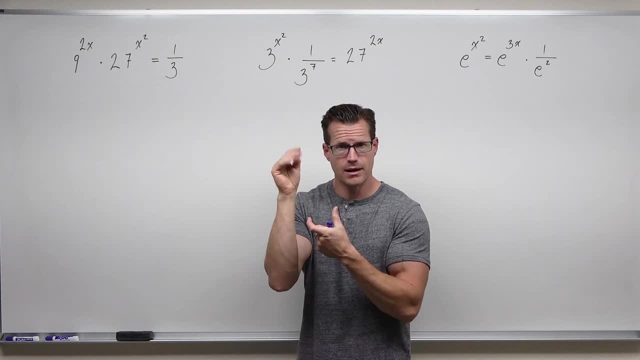 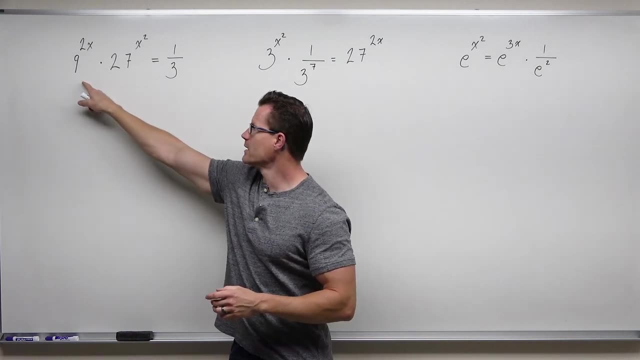 We know that when common bases are multiplied, you can add exponents, and that's a really good thing. If not, then we're going to have to use logarithms somehow. So we look at 9 and 27 and 3.. 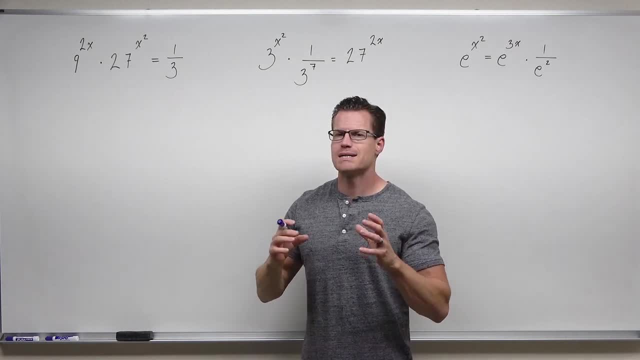 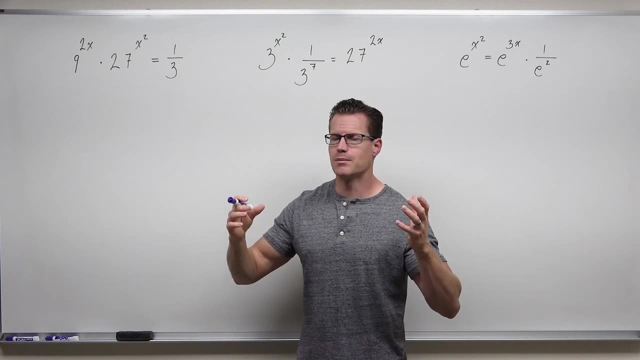 3 acts as your base here. Can I write all of those as one base? Take a look at your smallest base and see if you can write the larger ones as some sort of a power of that. So I'm looking at 9.. I'm 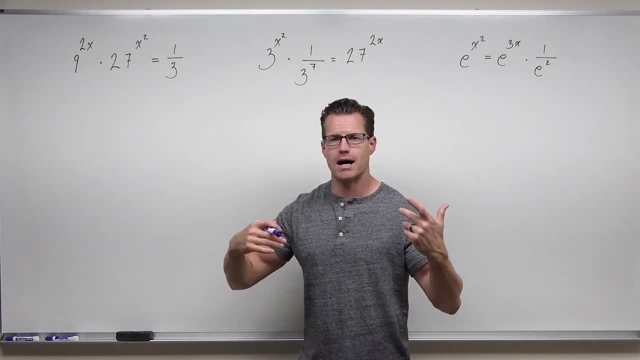 looking at 27.. I'm looking at 3.. 3 is the smallest one. Can I write 9 as a power of 3?? Yeah, it's 3 to the third, And so we're going to take a moment. We're going to do that. 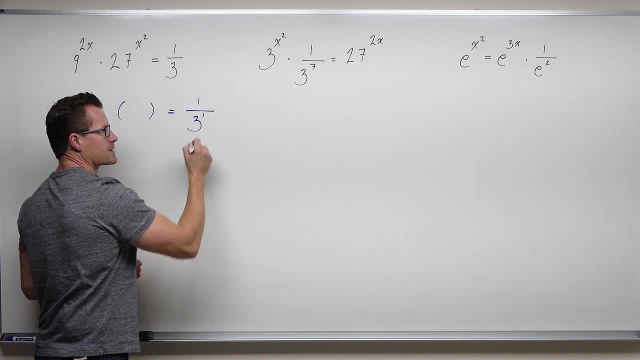 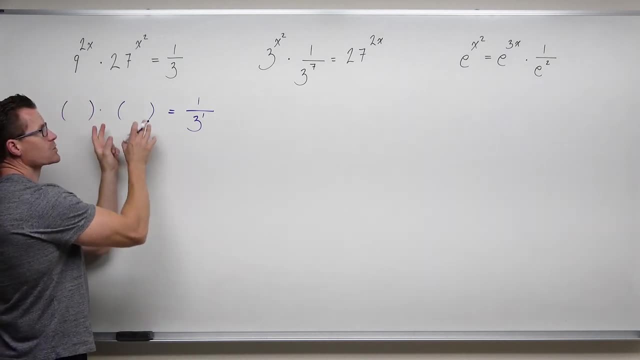 I'm going to start with my 3.. I'm going to remember that 3 has a power of 1, so that's going to be important because that's a fraction. We're going to be writing that as a negative exponent in just a moment. I'm also, before I do anything here, going to write my exponent. 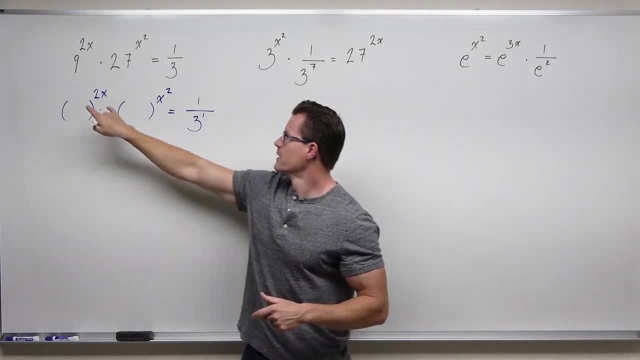 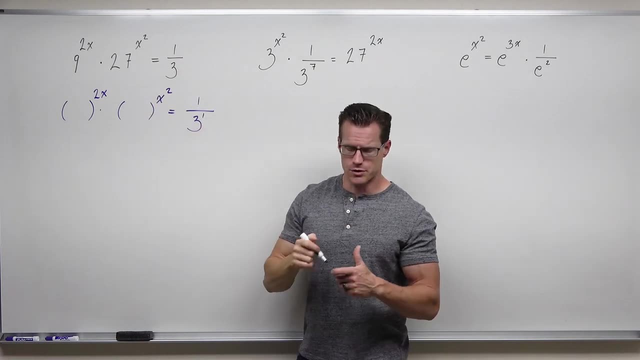 and my exponent, so I don't forget about it. So I know that. 9 to the 2x. I have my 2x. 27 to the x squared. I've got my x squared And this is 1 over 3 to the first. I have my 3 to the first. 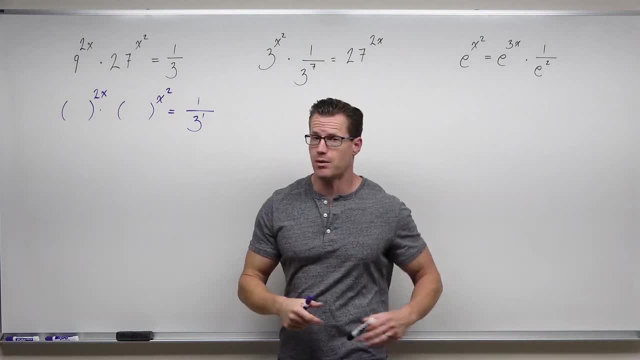 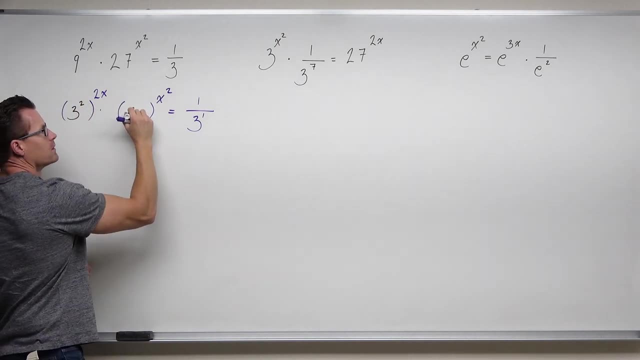 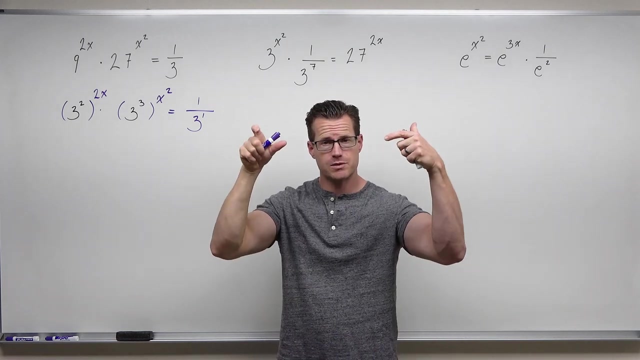 Then I go inside and I rewrite 9 and 27 as these powers of 3.. 9 is 3 squared and 27 is 3 to the third. But because of the way we wrote this- in parentheses and with our exponents already up there- 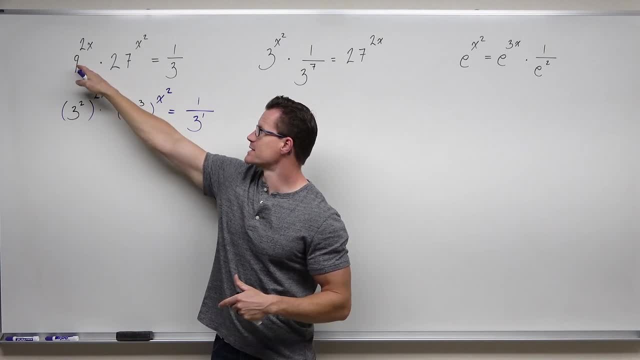 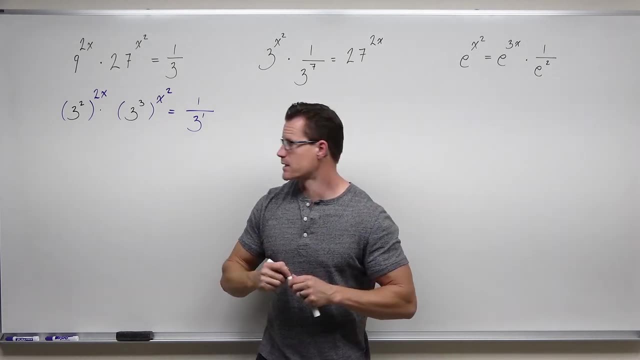 it shows us that we're going to have to multiply this, So this represents 9,. but to the 2x power, we know that we should get 3 to the 4x power. 2 times 2x is 4x. 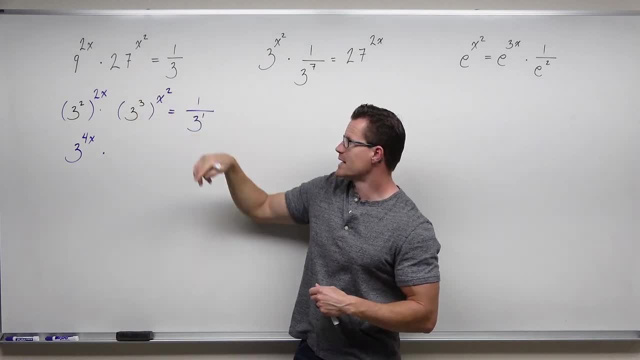 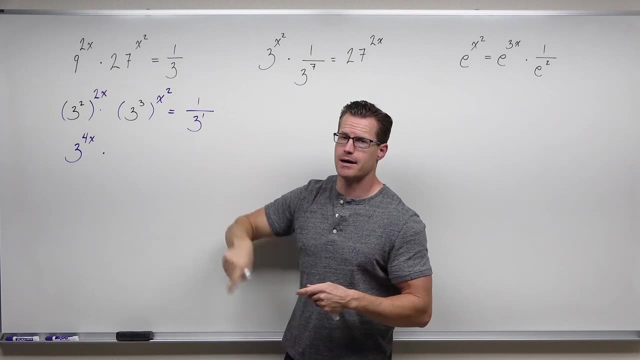 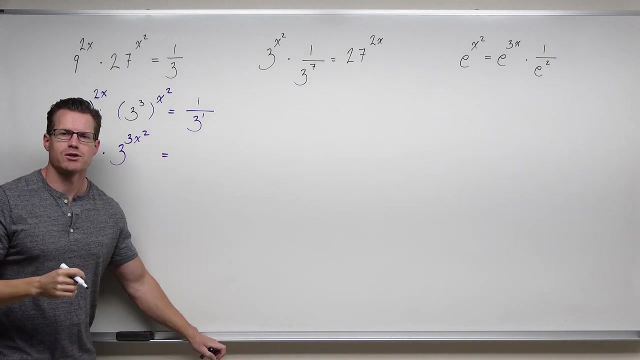 27 is 3 to the third and we're raising that to the x squared power. but because we have an exponent raised to an exponent, we're multiplying. This is going to become 3 to the 3 times x squared, Whenever you get a fraction and you're going to use this technique of solving these exponential. 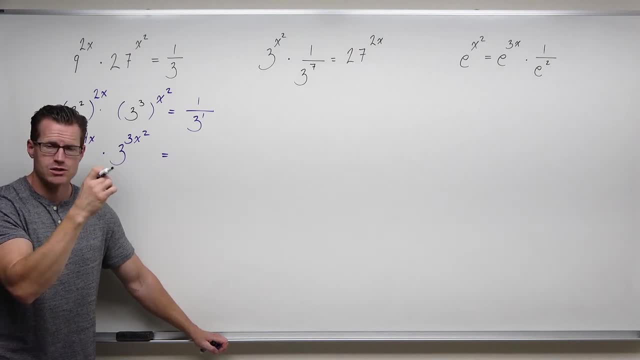 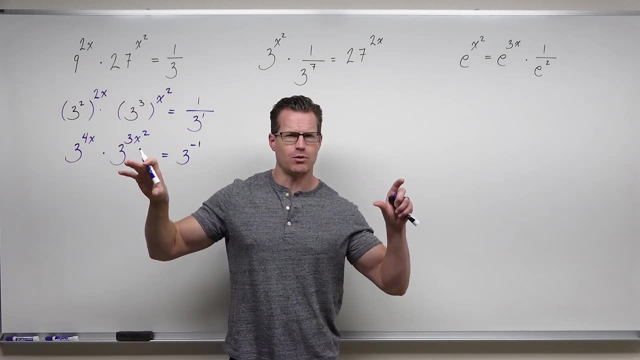 equations with common bases, make sure that you write any sort of fraction as having a negative exponent. So this would be 3 to the negative 1 power. That puts everything almost on the same level, if you will, where we have the same base, same base, same base. Now this looks really good. 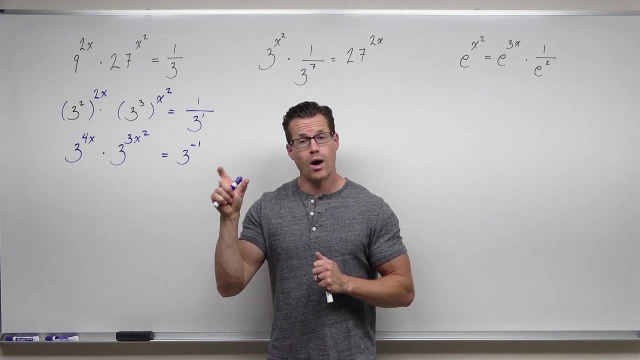 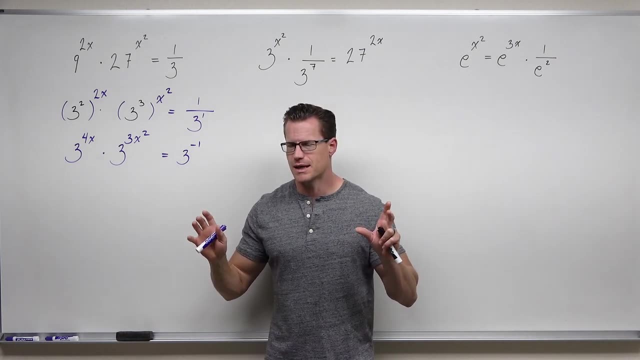 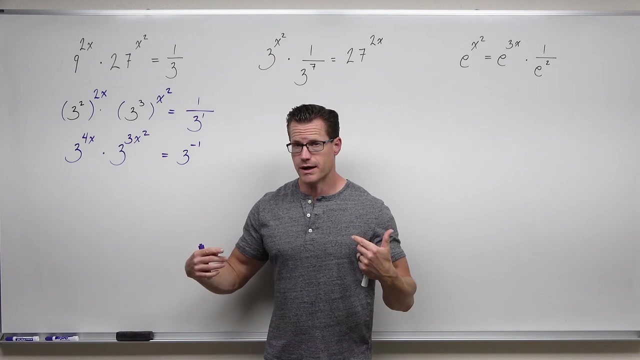 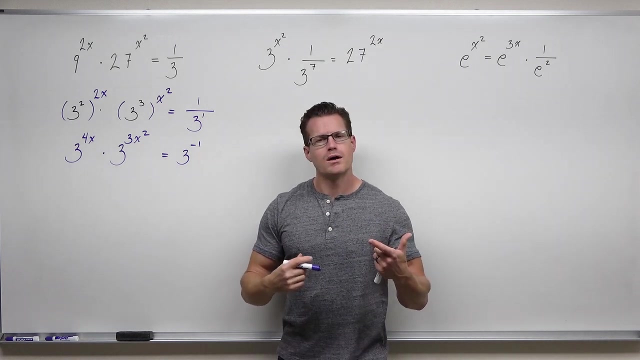 but the only way this technique works is if you have one exponential equation equal to another. However, the great thing about using this common base technique is if you can get common bases in all of your expressions here that are multiplied or divided, you can combine them. So 3 to the 4x power times 3 to the 3x squared power, you can combine. 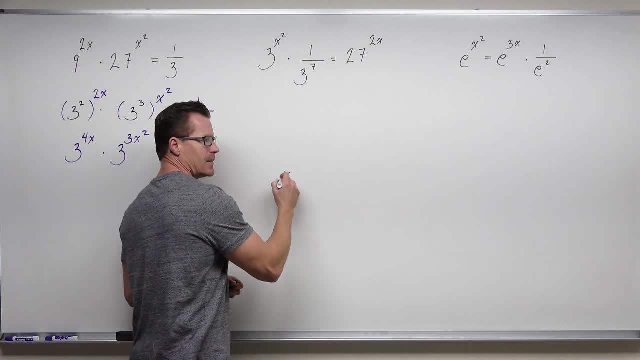 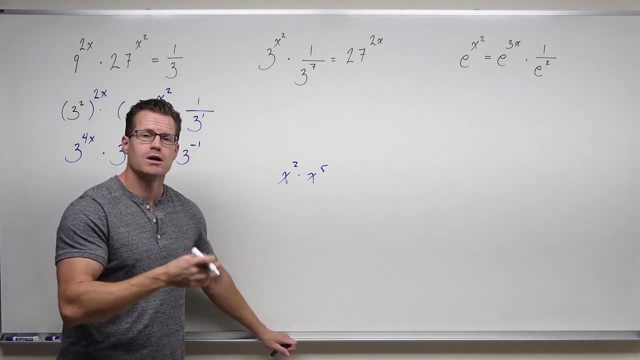 those. Remember this that if you ever had x squared times x to the fifth, you can combine those and make it x to the 7. You can add exponents, but this leads to a really, really common mistake. You can probably. 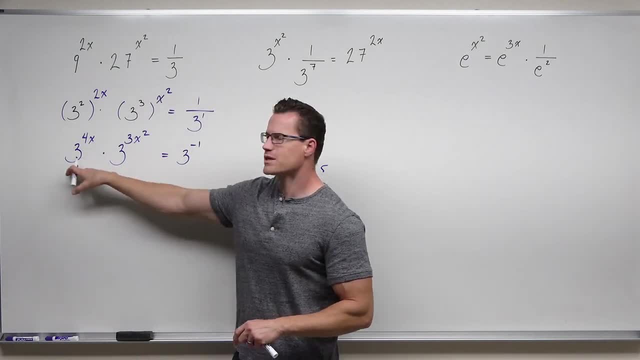 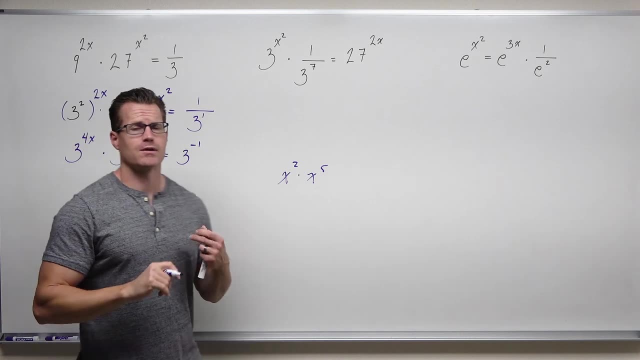 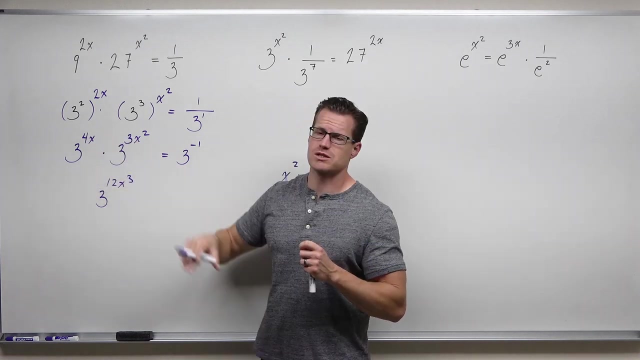 see it, I've seen this so many times, where students go: oh this is fantastic, I can combine these. I see it very, very often. It is so common for us to see multiplication and really, really want these two exponents to be multiplied, but that's not what happens. x to the second times, x to the. 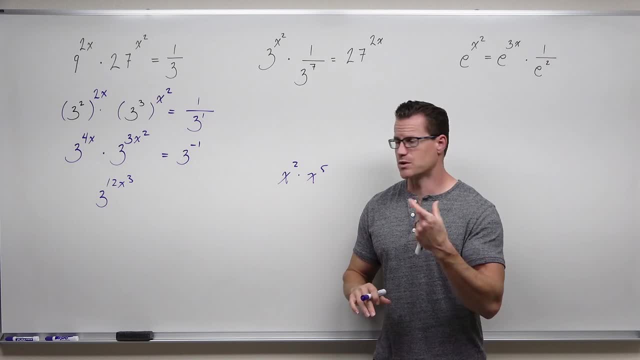 fifth gives us x to the seventh. You can add exponents but this leads to a really, really common mistake. So 3 to the 4x power times 3 to the 3x squared power, you can combine those 7.. Not x to the 10th. We add 2 plus 5.. 3 to the 4x times 3 to the 3x squared. We're going. 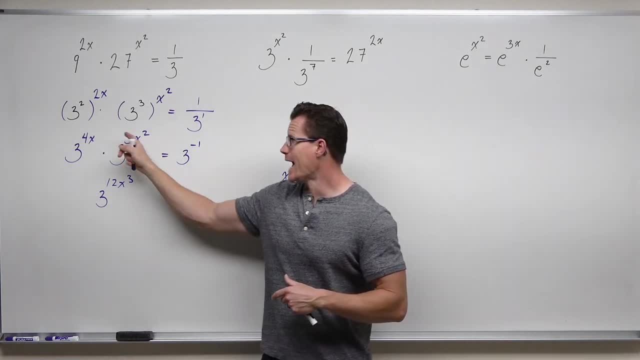 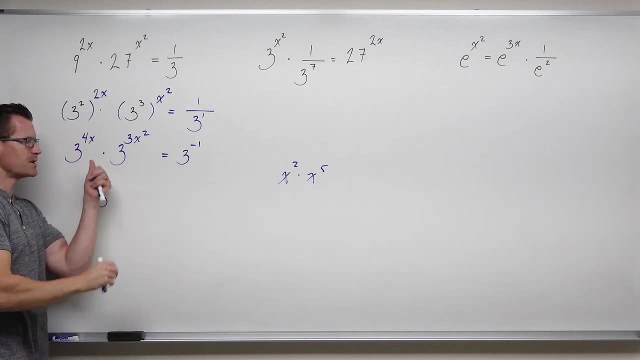 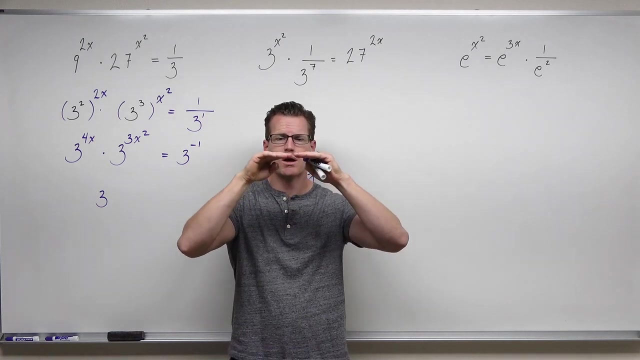 to get 3 to the 3x squared plus 4x, We need to add those exponents. Do not multiply. This is completely wrong. So common bases being multiplied. we know that what we do with exponents is one level below what we see. So if we see multiplication, operationally we're going. 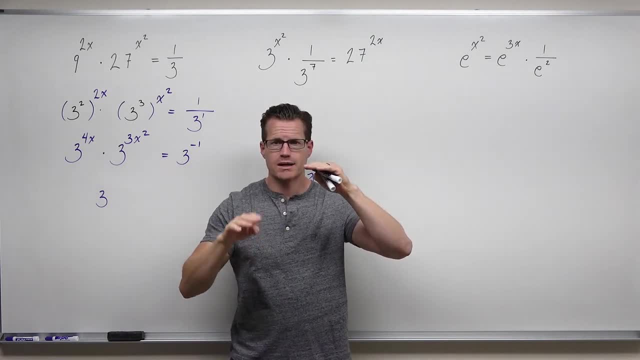 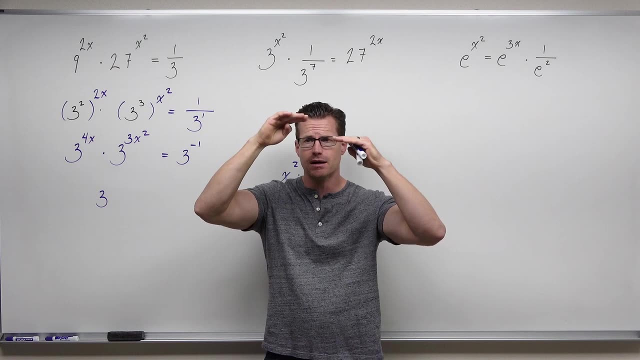 to be adding them. If we see division, we operationally subtract. If we see multiplication, we subtract. If we see exponents, we operationally multiply. That's what we've been doing here anyway. When we saw exponent raised to an exponent, that's an exponent level idea. But 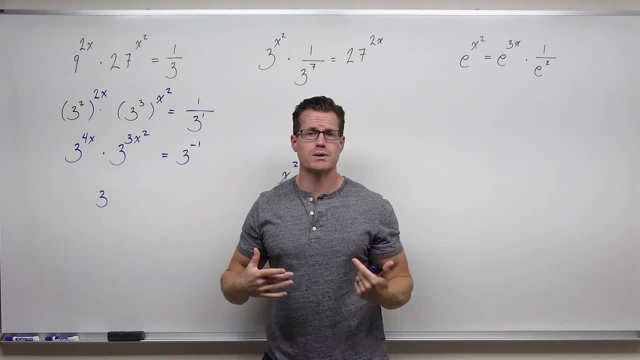 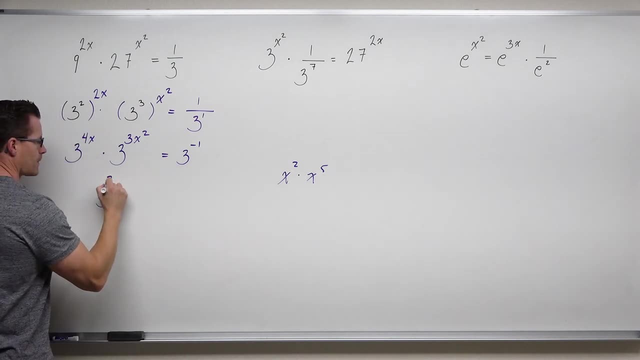 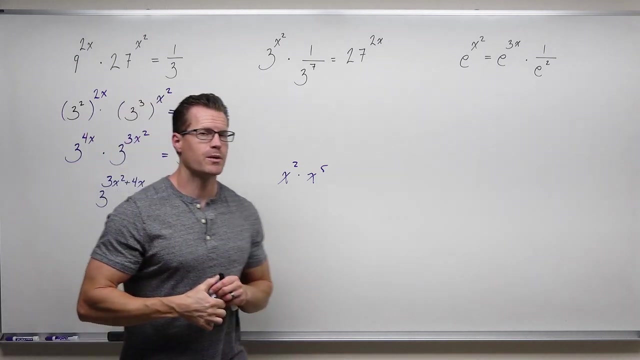 one level below that is multiply. So that's what we're doing here. We're doing one level below what we're seeing. One level below multiplication is you need to add those exponents. It looks a little bit more awkward, but this is exactly what we want. We have an exponential. 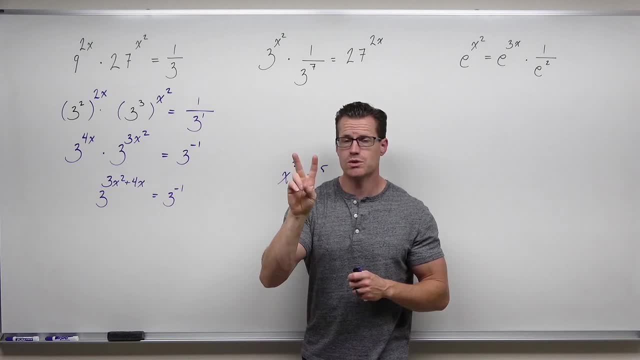 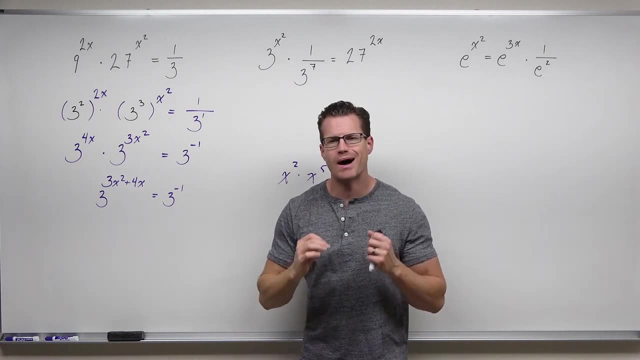 equation. We have the same exact bases and we have just two exponential expressions: One on one side- base 3.. One on the other side, base 3.. That's great. The only way these can possibly be equal is if our exponents are also equal. So this is the place. This is where we want. 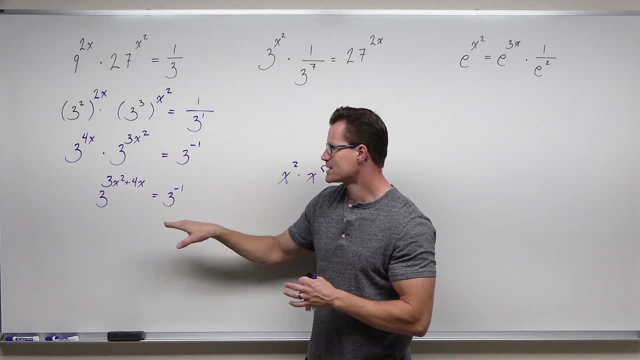 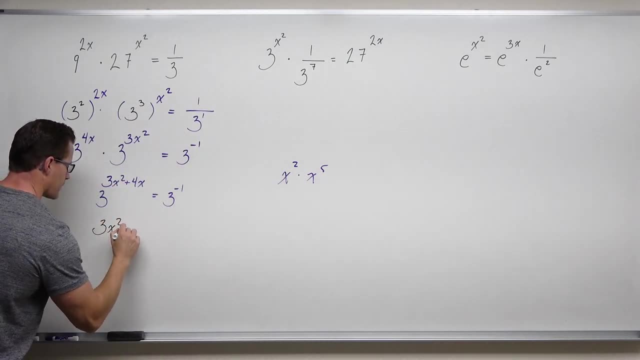 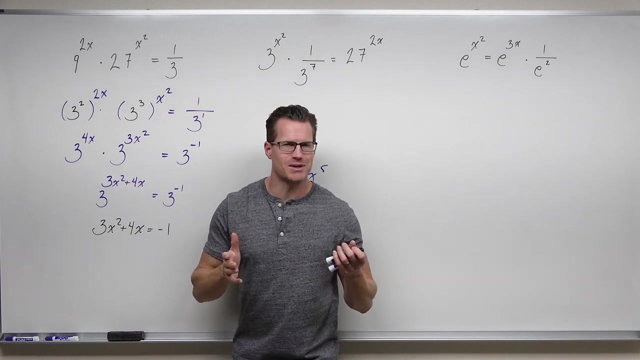 to be. essentially, We want to be at the spot where we can say: same bases, exponents are also the same. So we're going to do that. And now we get into something that sometimes we just forget what to do with. If you ever 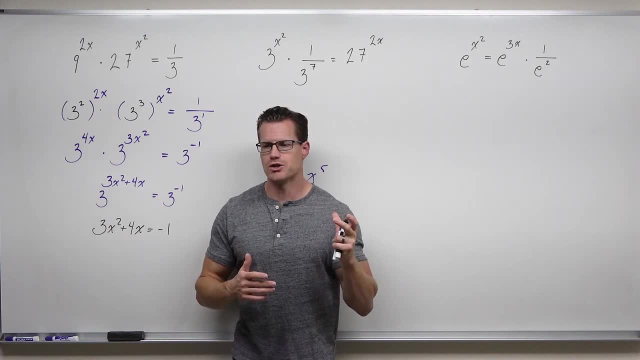 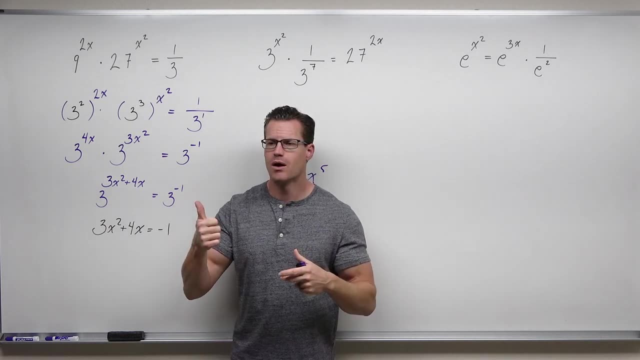 have a power 2 or larger in an equation. it's not a direct solving. It's something where you need another technique, And that's going to either be a square root method or factoring, some sort of a formula like difference of squares, something you're going to have to. 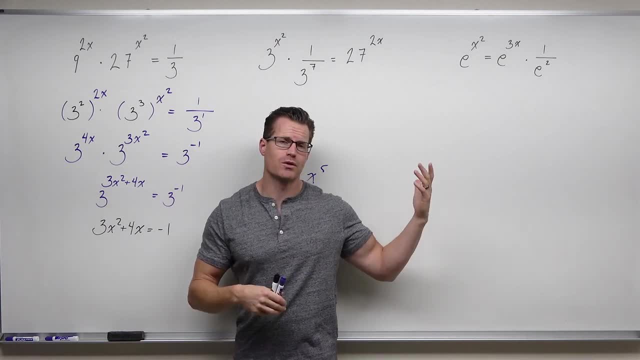 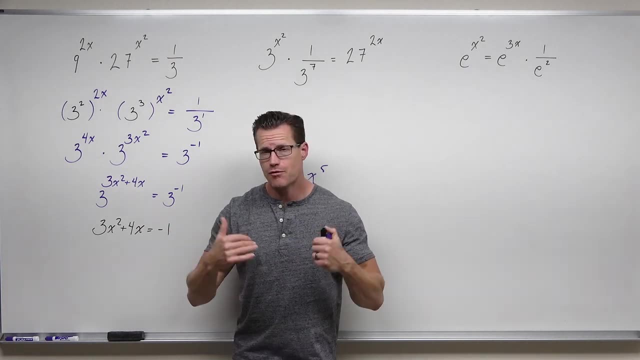 use in order to solve this. If you have power ones, like we had in some of our earlier examples, that's just fine. We can solve them directly by subtracting the smaller variable, adding strictly the constant and dividing. But if you have a power- two or higher, try factoring. So we're going to get everything. 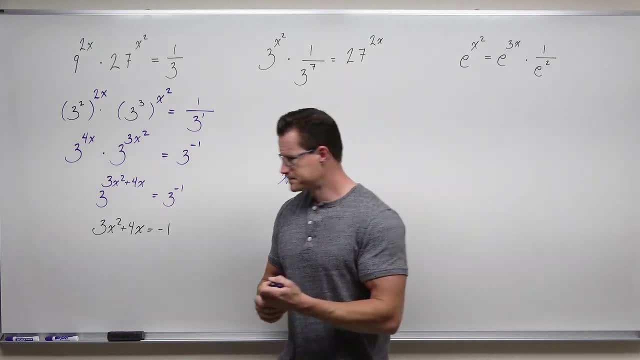 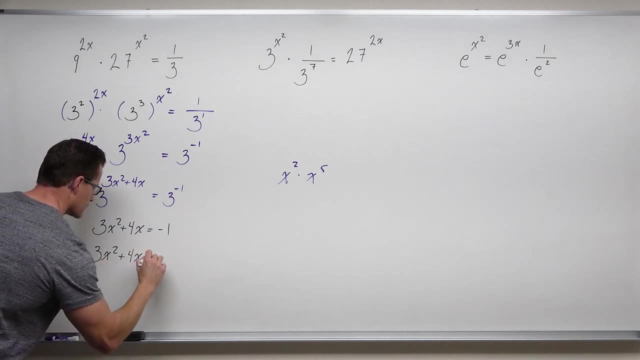 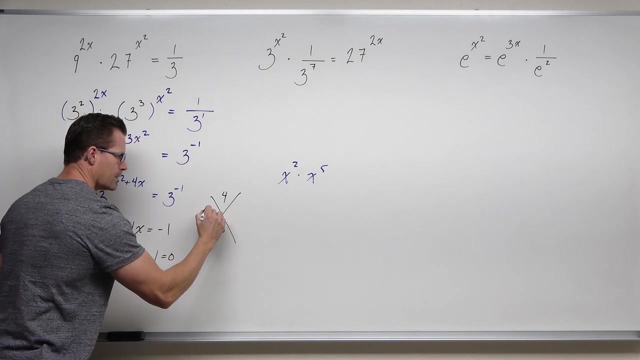 on one side in order first turn positive, and we're going to factor, Because we're really good at factoring. we know that we can put a 4, a 2, and then a 1 between them, Compared to a 4, a 4 and a 1.. 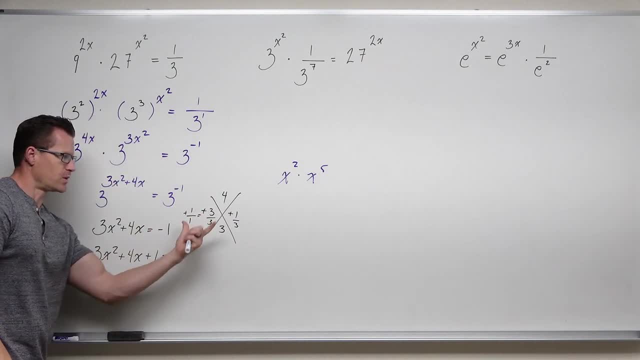 it's a condition that we dive right in our English degree and it's quasi-parallel. It's not a crazy thing, It's. and a 3, that's 3 times 1.. 1 and 3 add to 4,, multiply to 3.. If I divide by my a and 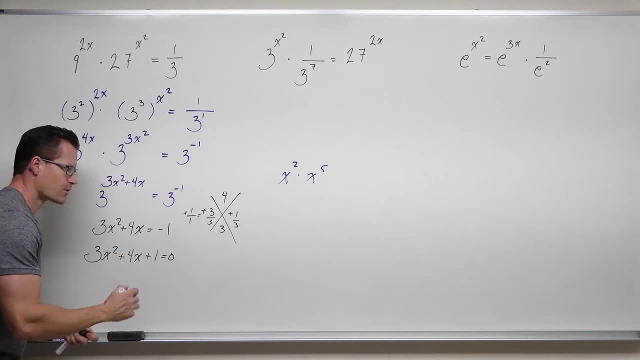 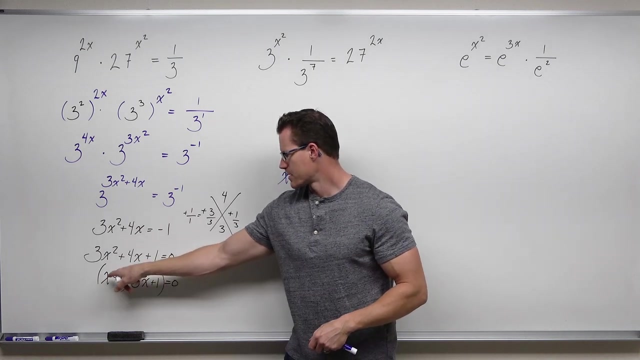 simplify 1. third doesn't simplify. 3 over 3 simplifies to 1 over 1.. That's 1x plus 1.. That's 3x plus 1.. And that actually works. Here's 3x squared plus 1 plus 3x, That's 4x. 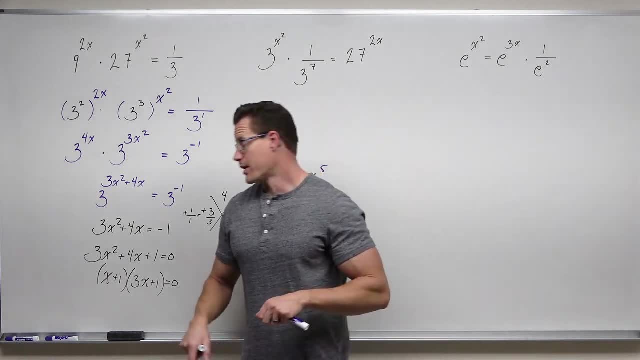 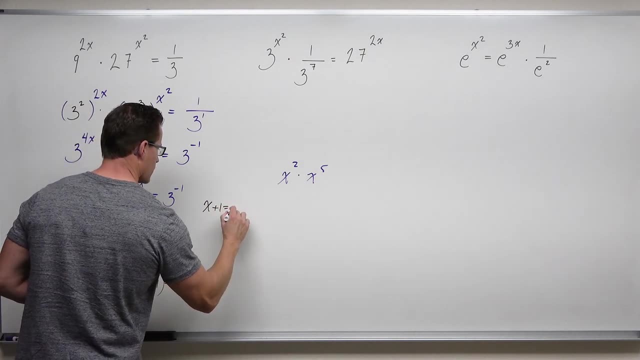 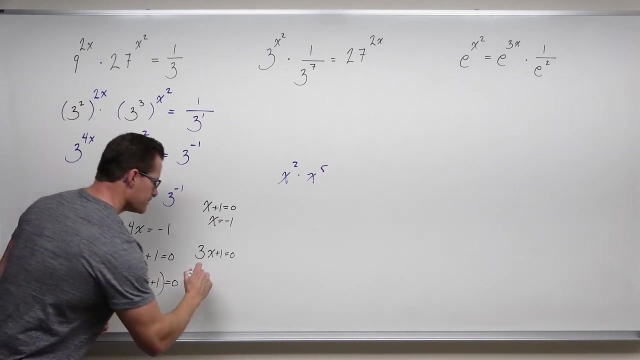 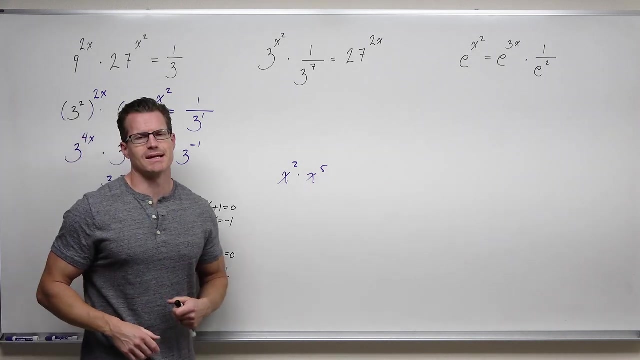 and then plus 1.. And if we set both of those equal to 0 by the zero product property, then x equals negative 1 and x equals negative 1. third, And we get our two solutions there. So I hope that's making sense. I hope you're seeing that the technique doesn't change. 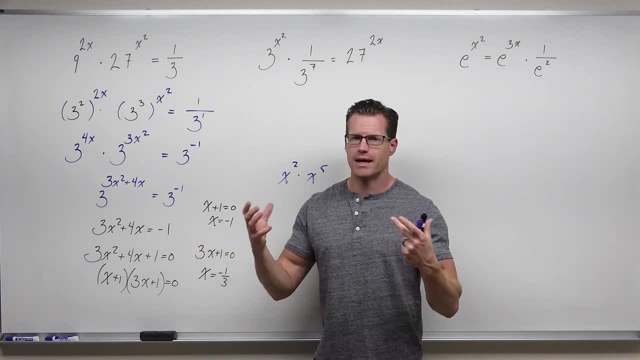 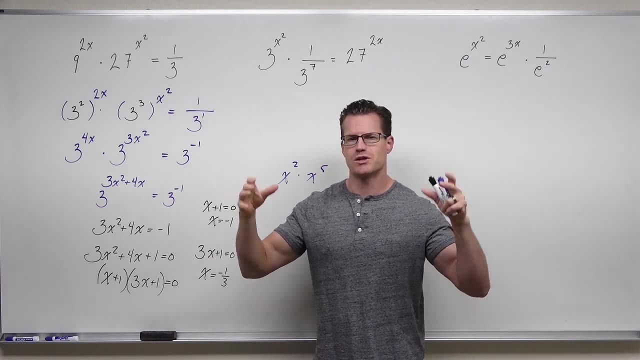 We're just a little bit more involved here And if you have more questions than one exponential expression on one side, you need to combine it. You need to have just 1 equals 1 exponential expression in order to set your exponents equal. Sometimes that takes some. 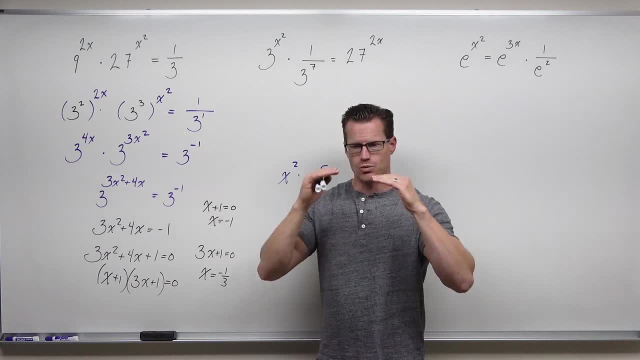 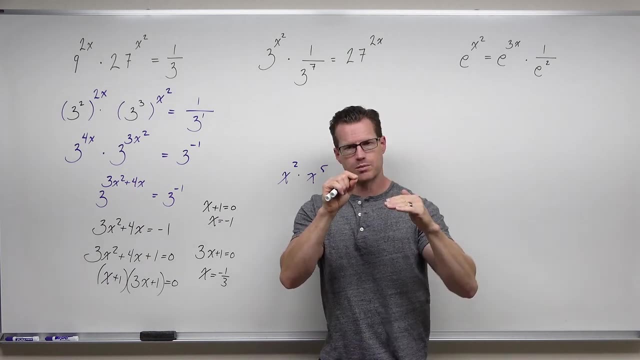 exponent work. Just remember: what you do with exponents is one level below what you see. So if you see exponents raised to exponents, you're not powering them. if you will, You're multiplying them. If you see multiplication or division, you should be adding or subtracting your exponentials. 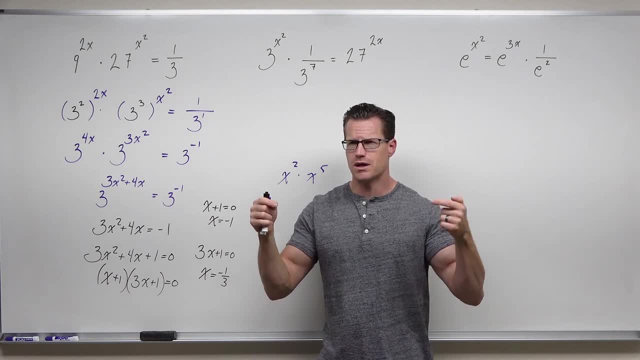 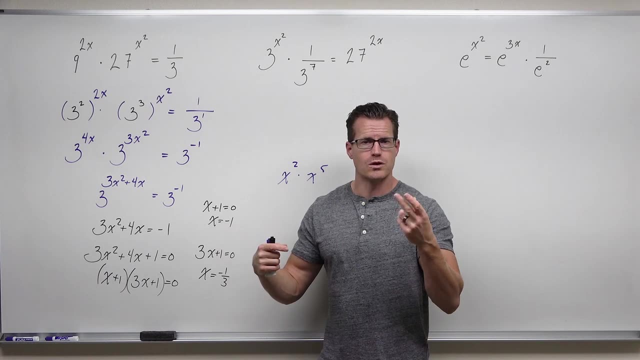 If you see addition, subtraction, well, wait a minute, there's nothing below those. So you don't do anything with your exponents, which means that's why you can't add or subtract your non-like terms. And let's say the same problem. 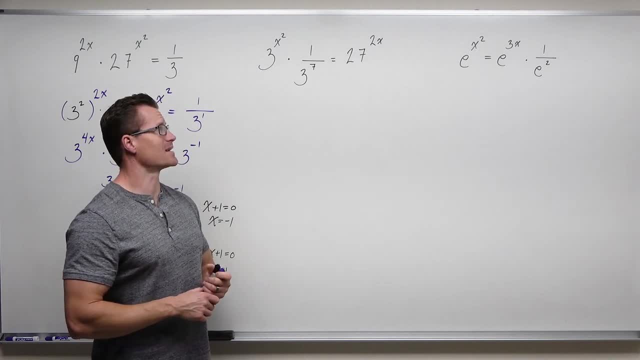 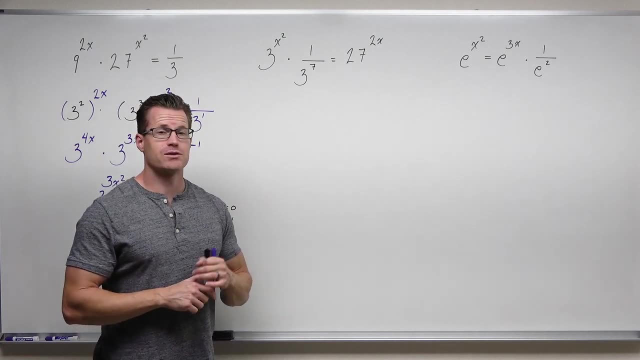 All right, let's move right along. So we have this next one. That's really nasty. It's got a fraction. It's got three different exponential expressions. Two are multiplied. If you do have any that are added or subtracted, so you might get to those, We'll deal with those a little bit. 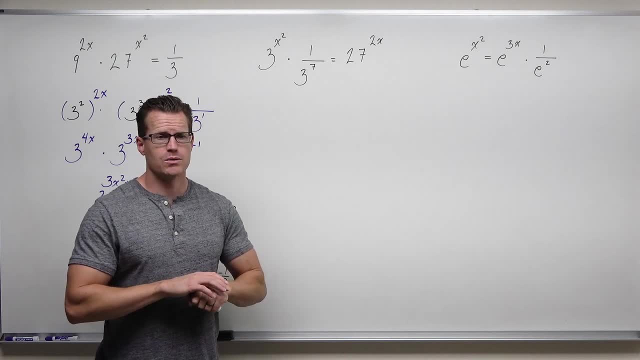 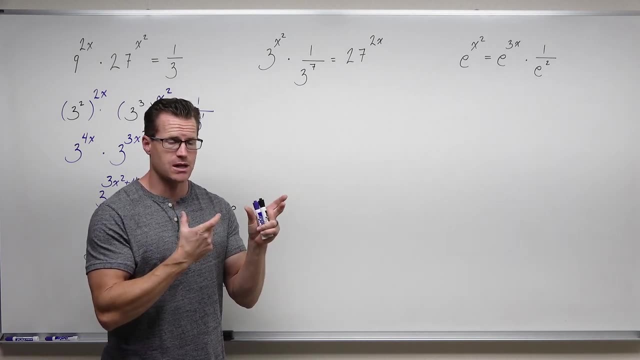 later. Those are typically a substitution idea. So this is what this is what you get when you can combine in such a way so you have one exponential equal to another. That's the only way that these common base solving by common bases work is if you can do that. If not, if you 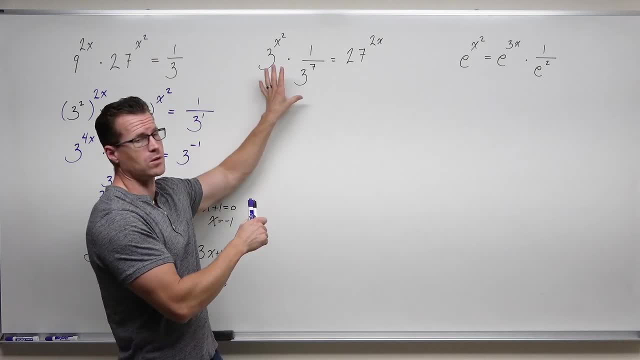 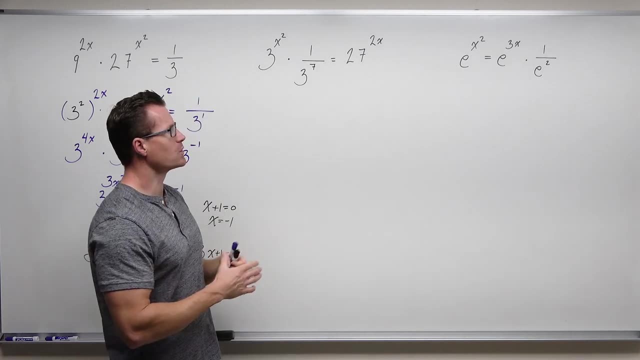 have more than that, more than just one term, this is still one term. It just has two factors that you can combine. If you have more than one term, typically it's a substitution or some other technique. So let's look at it: We've got two terms, but three exponential expressions. We've 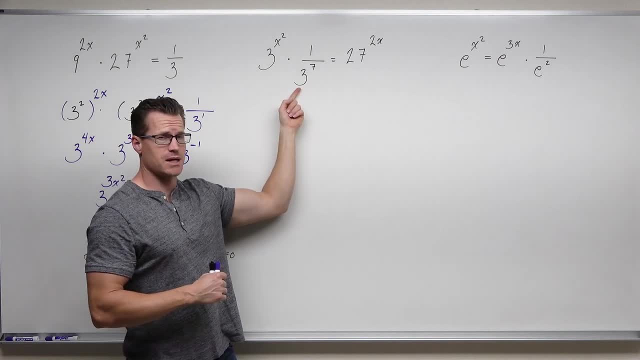 got a base three. We've got a base three. Notice this unpowerable. That is a base three. It just doesn't have a denominator. That's okay, We can deal with that. And we've got a base 27.. So we're. 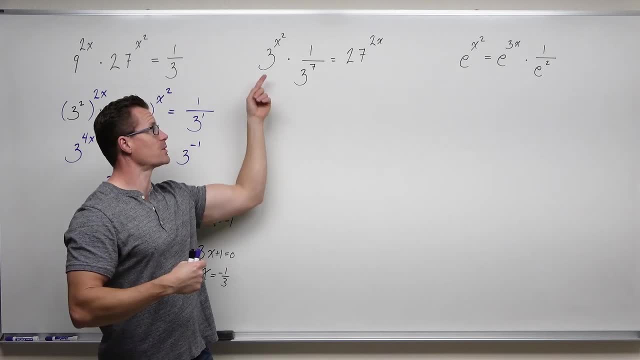 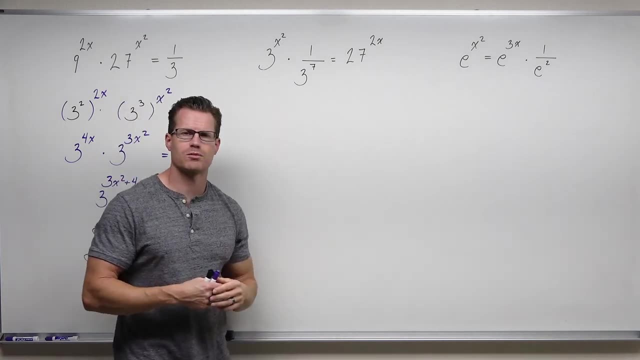 going to look at this and identify our smallest basis three. I've got it a couple of times. That's really good. Can I write the larger base, or bases, as that smaller one? Can I write 27 as a power three, Sure, So what if you couldn't? Well, you combine what you could and then you use. 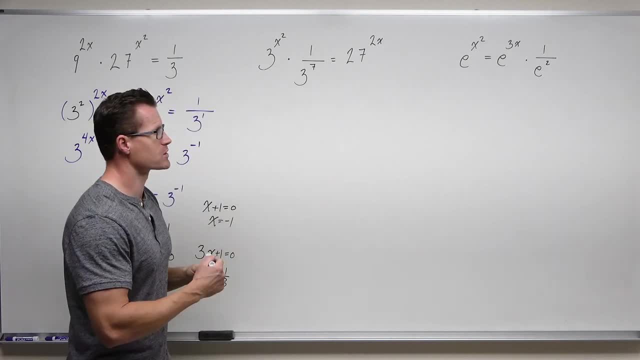 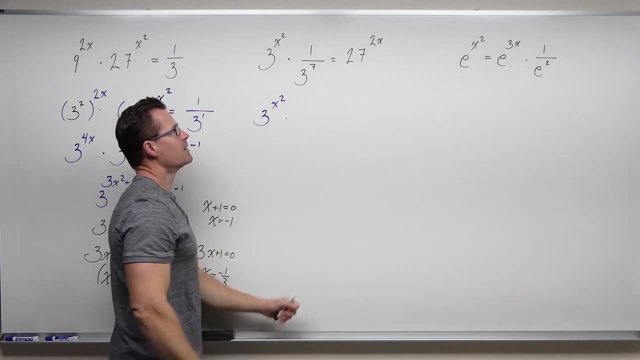 logarithms for what you can't Anyhow, if you don't have a common basis. we have a three to the x squared and we don't need to simplify that. Whenever you get fractions- and I could have given this- different right I could have given- 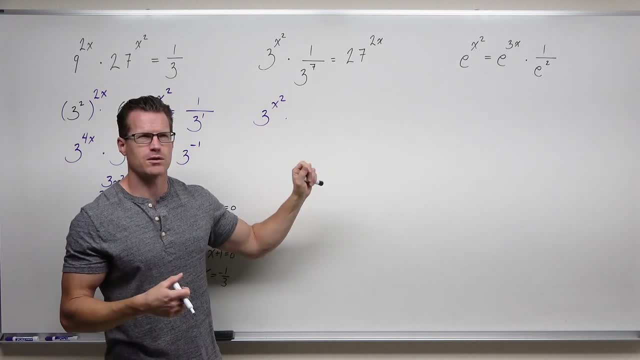 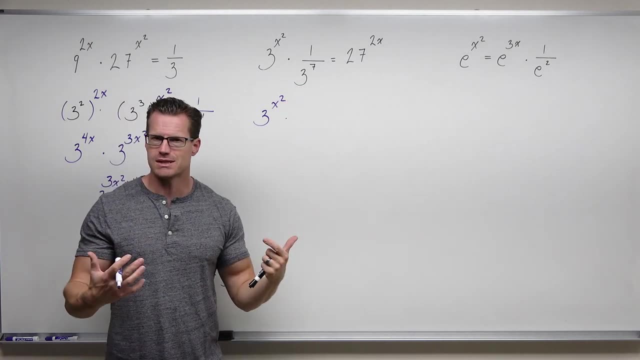 this like the 125. It made you think about that's five to the third and then that would be one over five to the third, so five to the negative third power. We just did that I could give this to you as the number three to the seventh. It's just a fairly large number and so I didn't want to have. 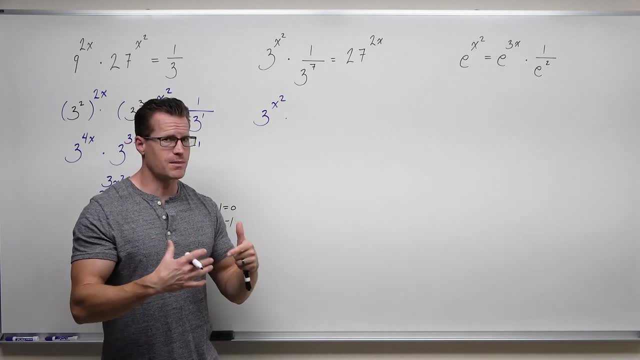 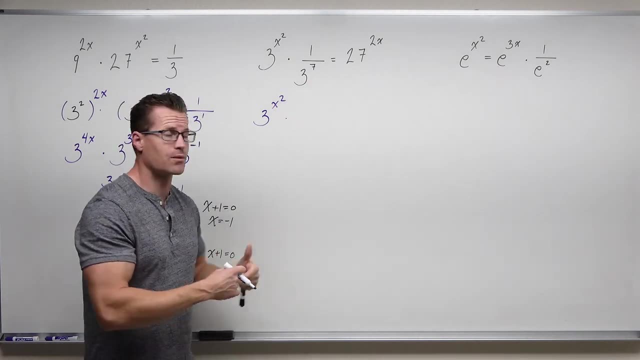 to think about that. So I could give that to you as a number. Just keep that in mind. You'd have to change this to a base of three and then say, hey, this is one over three to the seventh, But that's a fraction. I don't like fractions. Can I write this as a base on the same level as the? 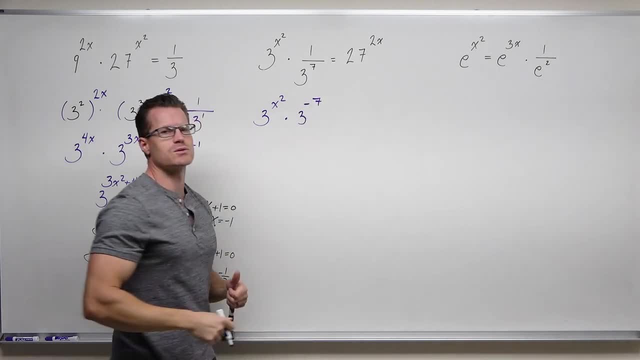 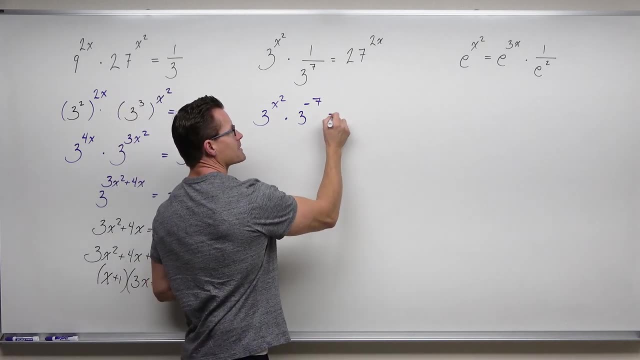 other bases to a negative exponent And the answer is yeah, we can do that, That's appropriate, That's what we want to do to get rid of those fractions. They're very hard to do otherwise. On the right hand side, we are going to immediately write down that exponent. We don't ever want to lose that. 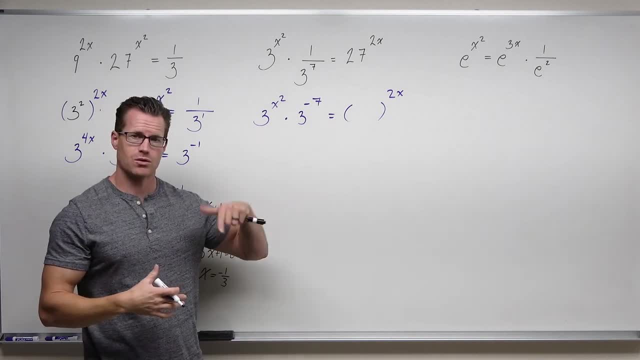 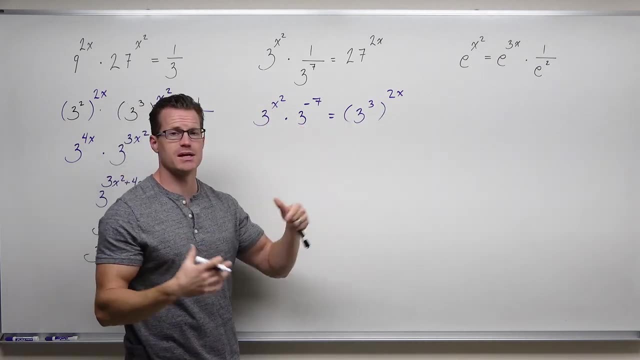 but the 27,. we're going to change, So 27 needs to be written as three. to the third power It says 27,. but to also say I want the same base so I can use this technique If that didn't work. 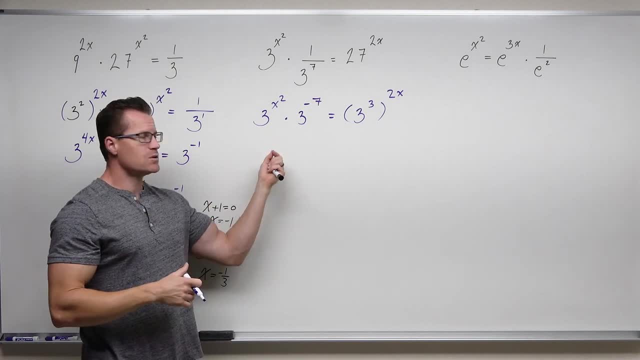 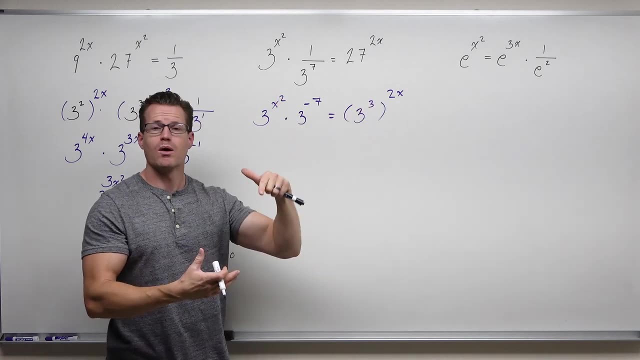 if that was not a three there, well then we'd have to combine these two and use logarithms. And now we're going to simplify a little bit more. We know that an exponent raised to an exponent, we're going to one level below. We're going to multiply those. 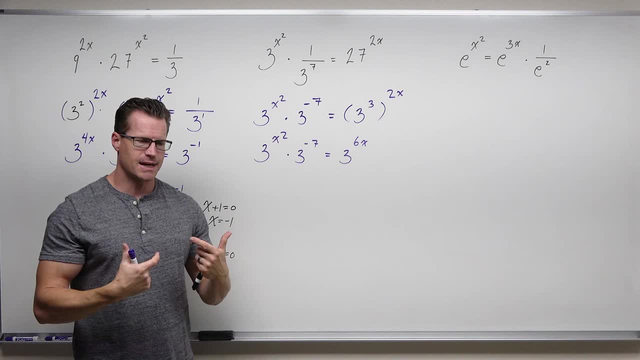 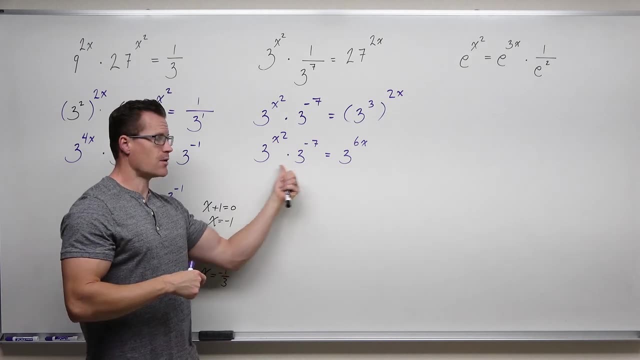 And that's six, X. We also know this common base technique where we set exponents equal, but we know that if we have one exponential on each side, that looks good. This doesn't. So we have common basis. That's great. This would not work if we didn't, But if we have common basis, 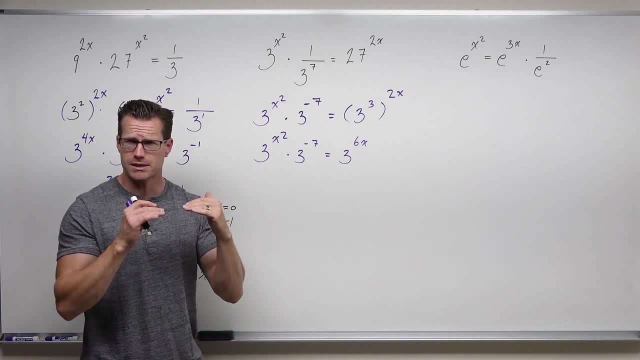 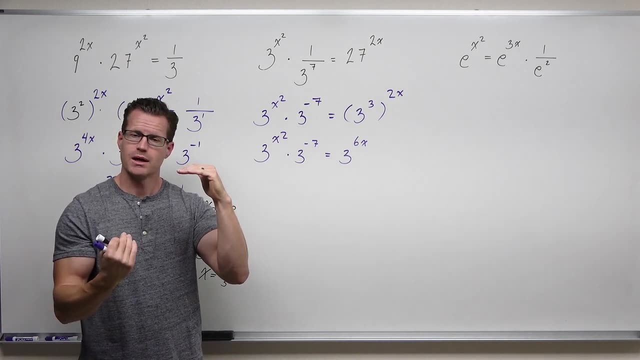 we know that when we multiply these expressions with common basis, we need to add our exponents Multiplication, that's the operation. you see. One level below that addition is what you do with the exponents, And so we're going to keep our base the same. That doesn't change. 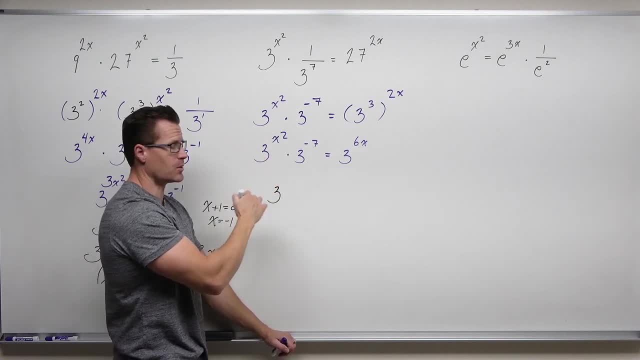 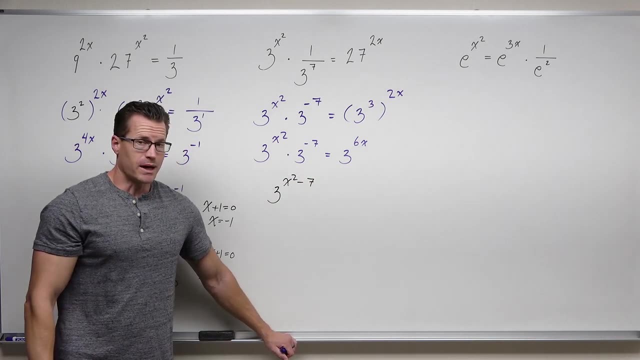 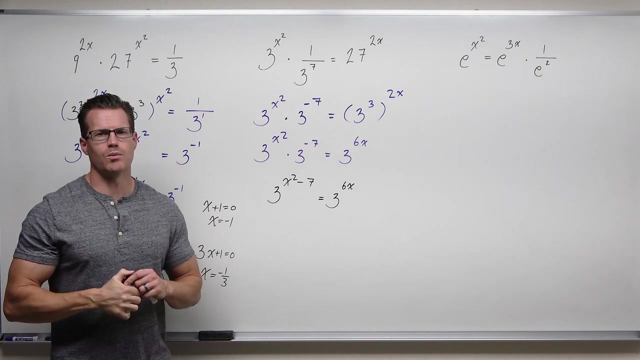 That's how exponent rules work. You keep the base the same. all the math is done with your exponents. If we add those X squared plus negative seven is X squared minus seven Equals three to the six X. This is what we want. I'm going to say it one last time. This is it. 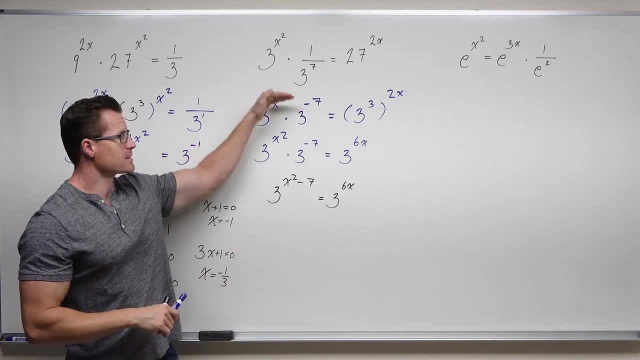 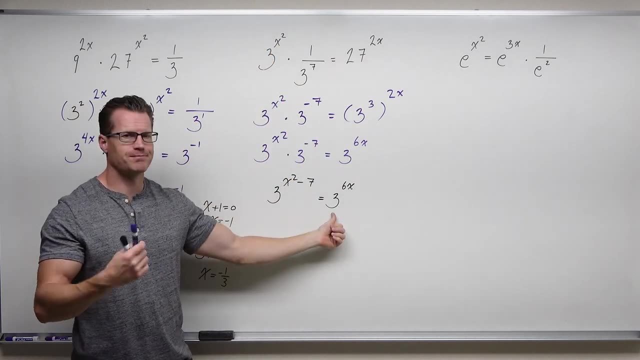 But if these were not the same number, you would have done exactly the same thing until you got down to here. You wouldn't actually even have to do anything with this, but you would have done this until you got here. Let's say that was like a four or something. Then logarithms would come in. 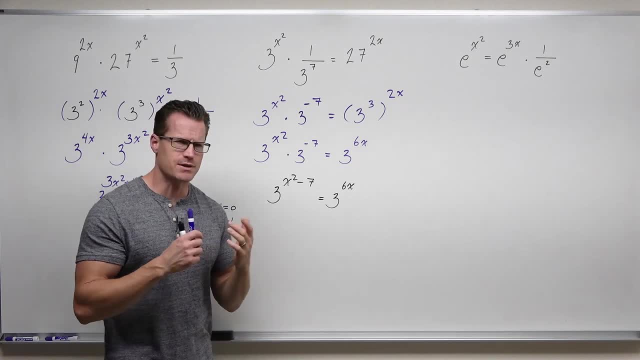 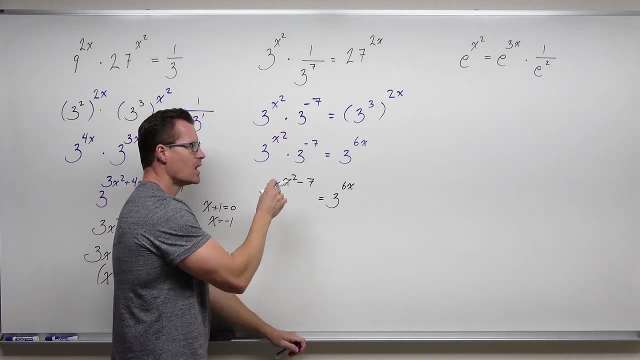 It would be the inverse, and you'd have to do it that way Here. this is a special case. We have the same basis. That's great If you have the same basis and two exponential expressions, one on each side of your equation. the only way that's true is if your exponents 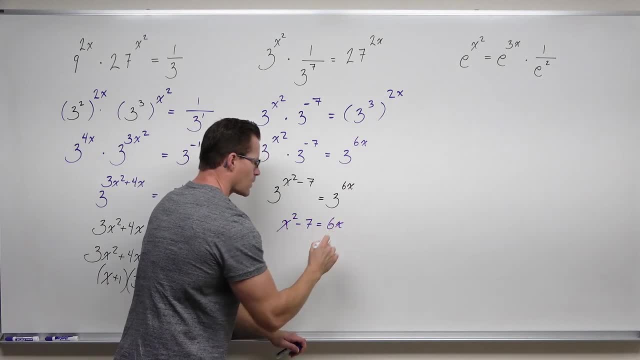 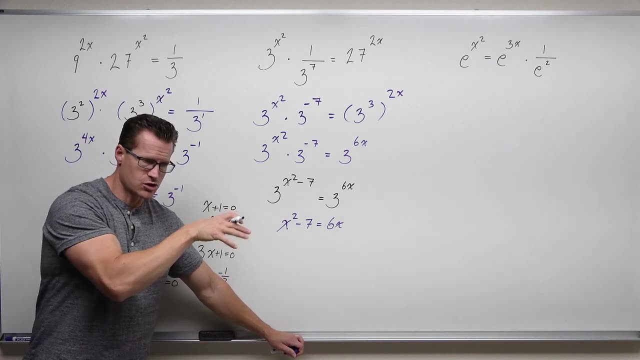 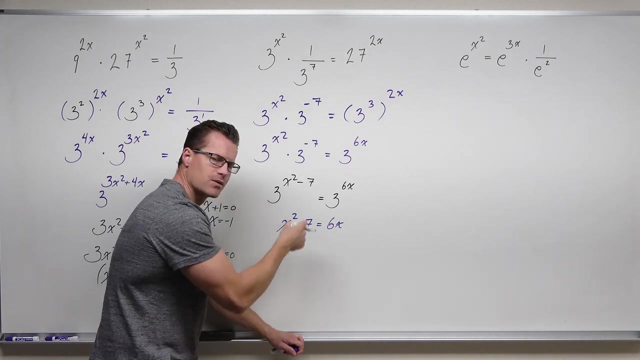 are also equal. We see another: power two. That means that we're going to have to use some technique beyond just solving for X directly. We're going to need to factor this. So let's get everything to power two or higher. This is your technique: Get everything on one side and then check it out. 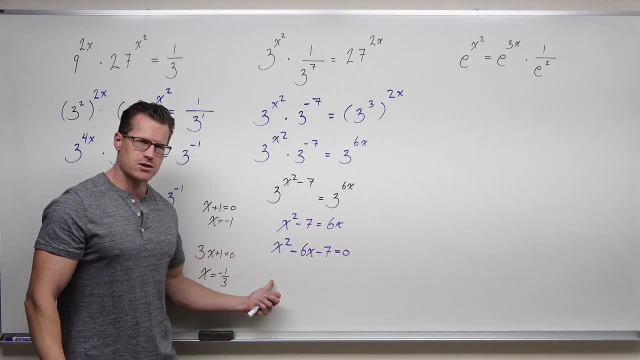 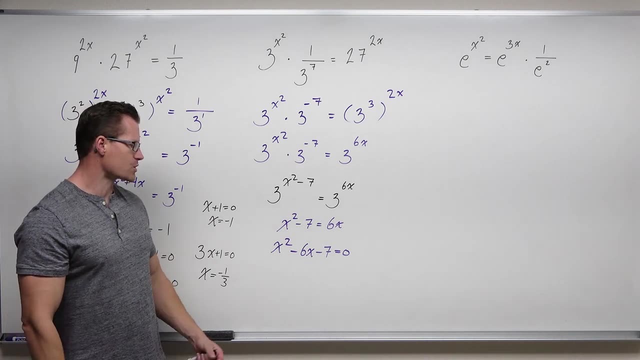 So by checking it out. I mean, how do we solve that? Can we factor it? Can we do quadratic formula? Is there another technique? we have Square root method, different squares, something like that. So here we'd say: yeah, that factors. 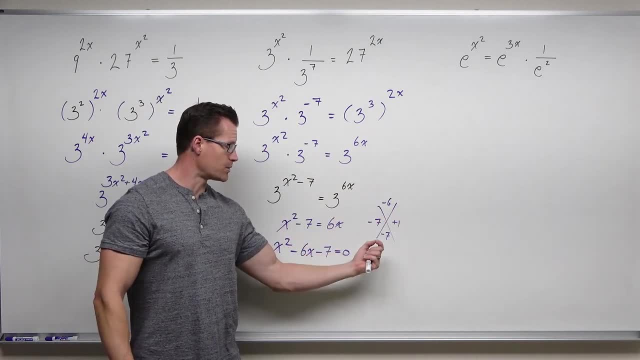 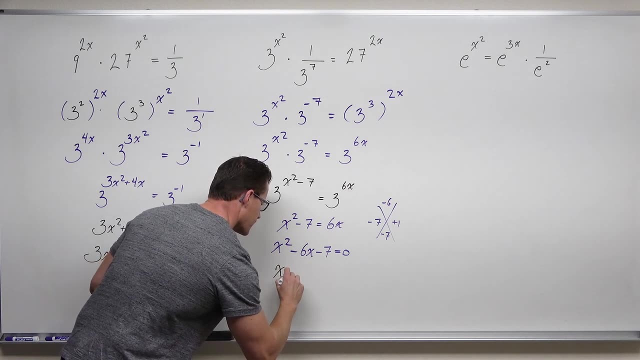 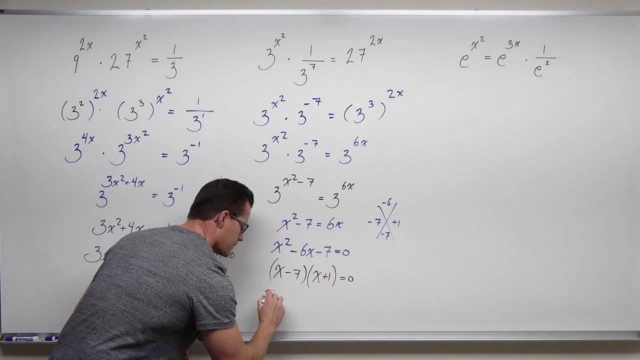 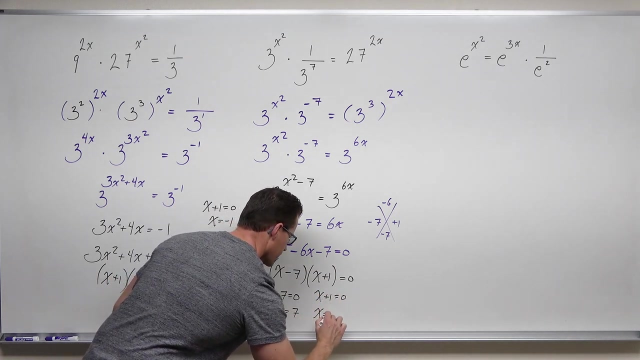 Looks like negative seven, One that adds to negative six, that multiplies to negative seven, because our A is one is a nice factorization for us, And if we use a zero product property, we get two solutions out of it. We get X equals seven. We get X equals negative one. 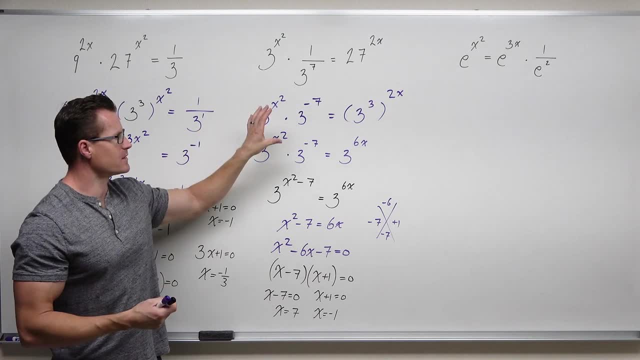 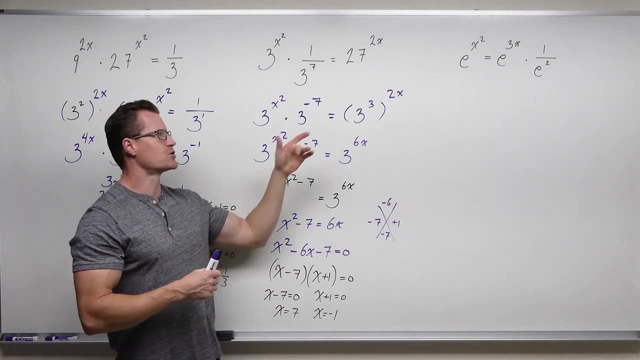 We get X equals zero. We get X equals X. So I hope this makes sense. I hope you're seeing the technique getting your fractions to be negative exponents, combining your like bases or your common basis appropriately and making sure we don't lose those exponents And keeping 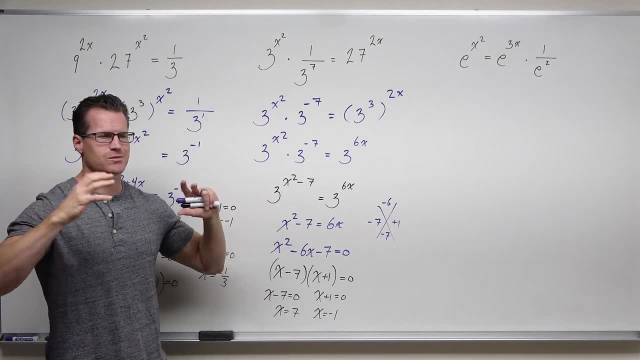 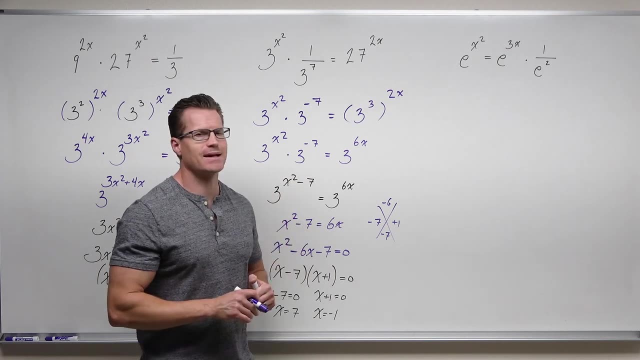 the back of your mind that you know, if you're not able to get those common basis, we have something else later that we're going to teach you. All right, we get the last one, And even though it has those Es in there, this is actually a little bit easier, And the reason is because 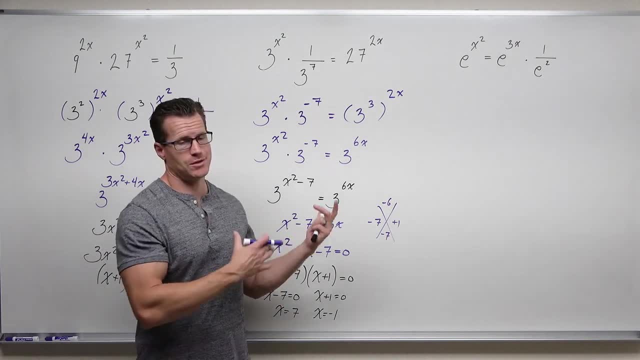 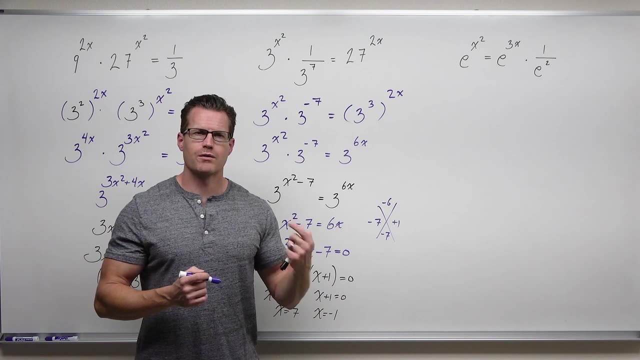 is because there's no argument about what kind of common base you're going to have. It's given to you. You have a base of E and you're not going to have to manipulate hardly any of it. The only thing that we have is that 1 over E squared to the second power We're going to have to change. 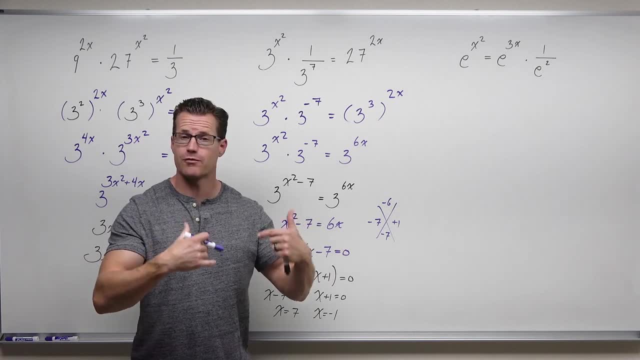 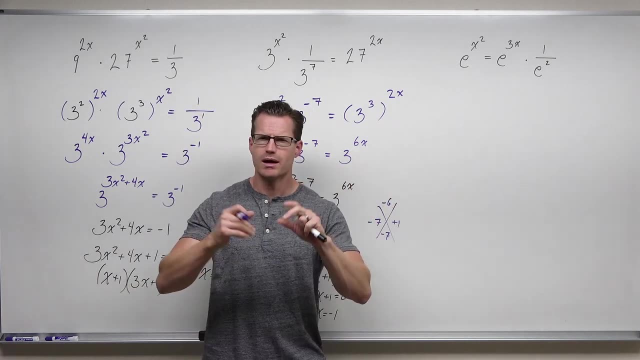 that That's a fraction. We always want to take our bases that are within our fractions and make them a base to a negative exponent. Other than that, this is pretty straightforward. This is really nice. We can see right away that we're going to be able to use the common base technique. 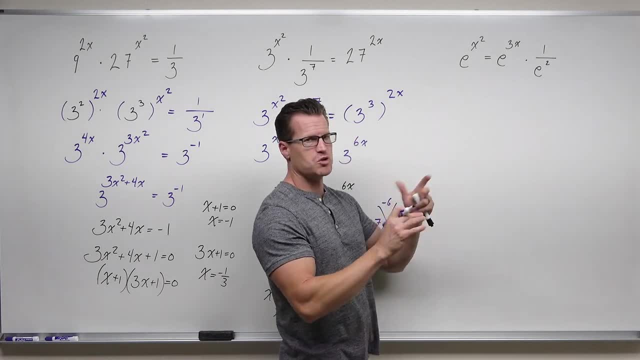 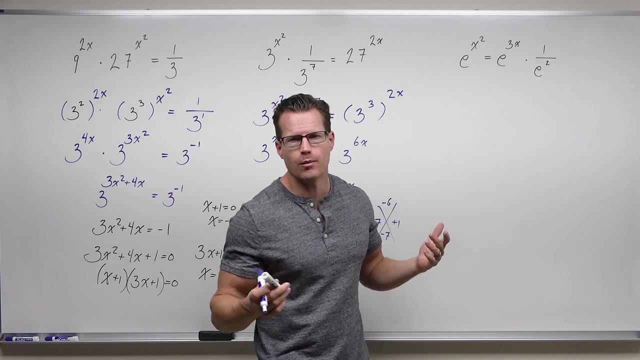 So E to the x, squared great E to the 3x, no problem. Remember, E is just a number. It's like any other number. It just happens to be written as E, It's 2.7.. It's like any other number, It's. 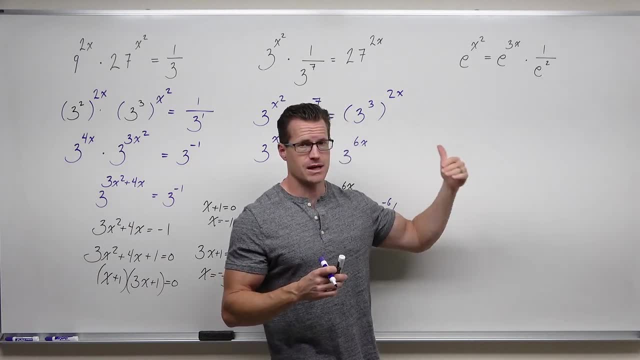 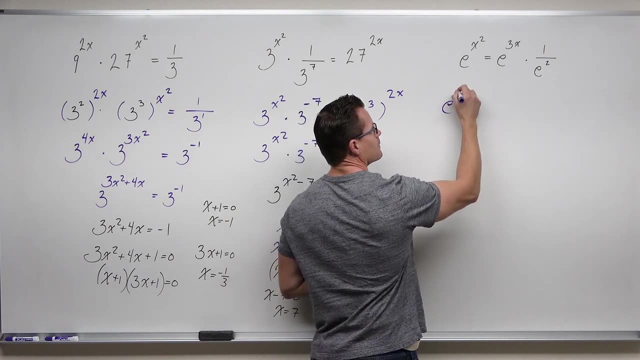 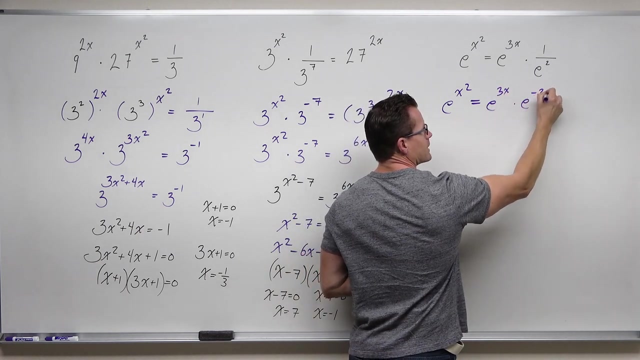 a transcendental, but in that it's not a fraction, doesn't ever terminate, But it is still a constant, And so we can write this as E to the x squared, E to the 3x and E to the negative 2.. And so we can write this as: E to the x squared, E to the 3x and E to the negative 2.. And so we can write this as E to the x squared, E to the 3x and E to the negative 2.. 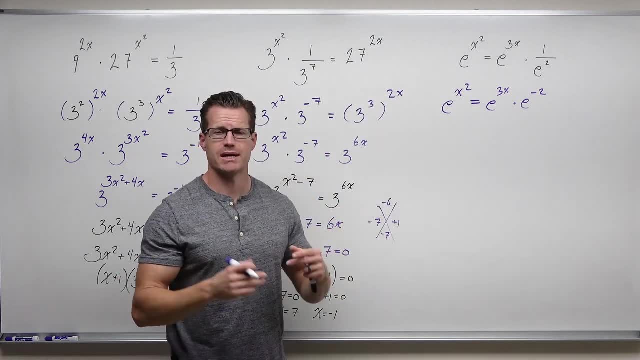 It's just a number, they're just exponentials, and now you have the same base and they're on the same level. Nothing in fractions. that's really good. The next thing we're gonna do is understand that in order to use our technique. 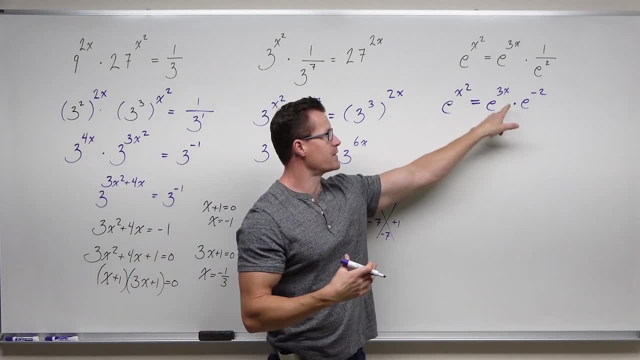 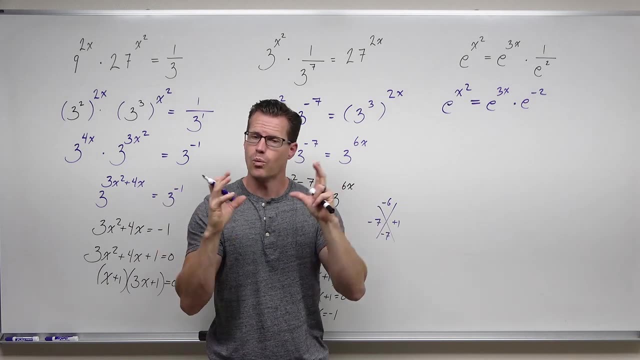 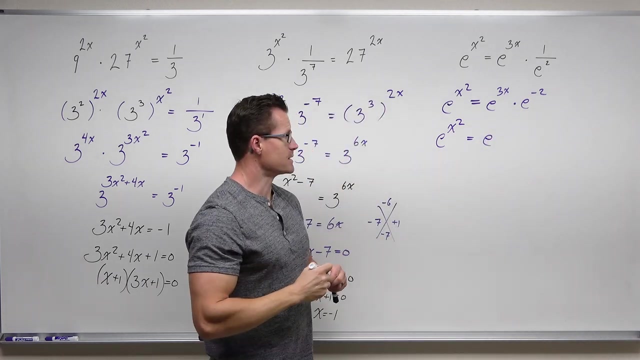 we need one exponential equal to one exponential. This is great. this is not Because we have common bases being multiplied. we know that we can add our exponents together and create one exponential. What that means when we're adding this is e to the three x times e to the negative two. 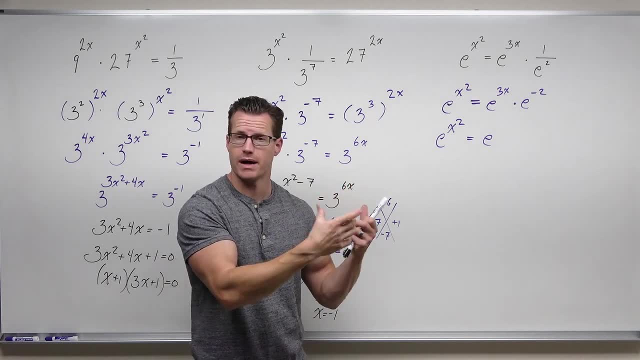 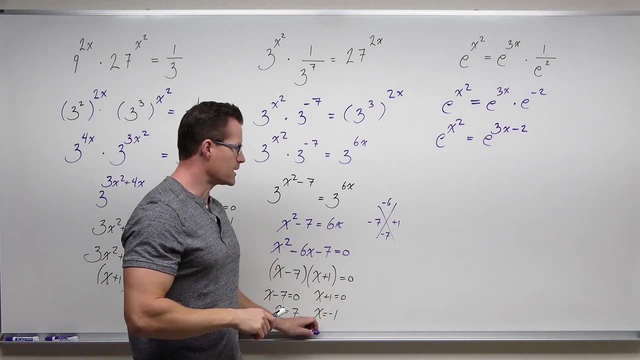 is the same thing as e to the three x plus negative two or three x minus two. And that's what we're looking for. We're looking for with this technique: two exponentials, same base, and that means your exponents also have to be equal. 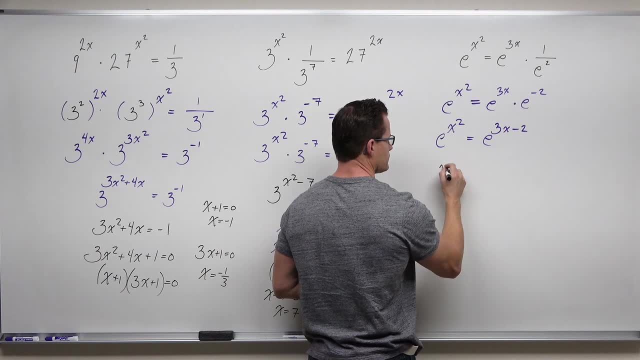 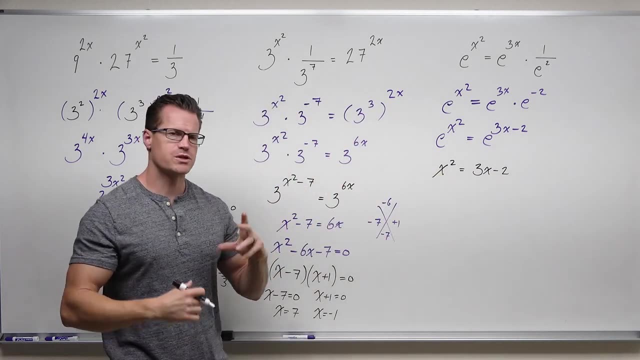 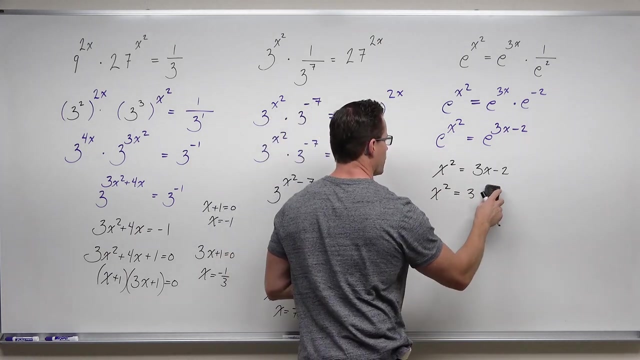 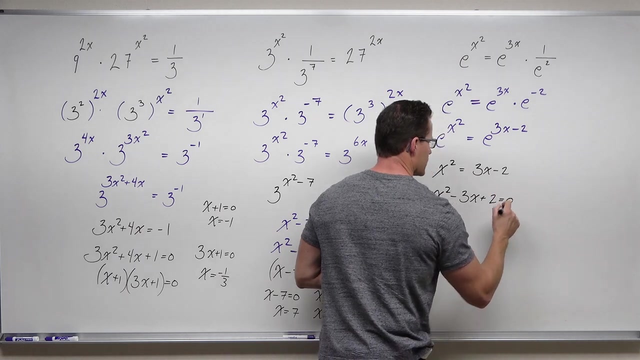 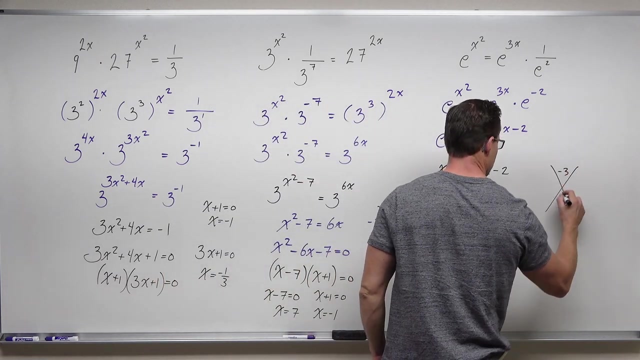 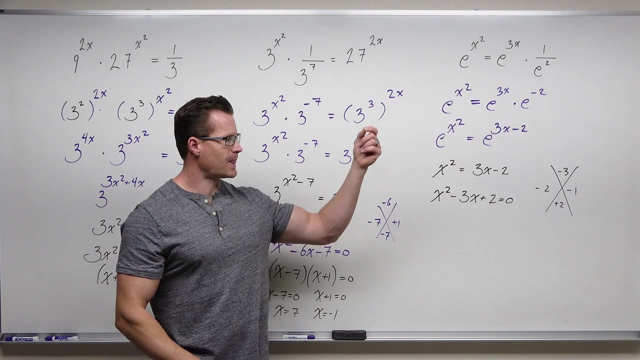 in order to satisfy this equation. So when we solve this, we're noticing the power of two. this is gonna be another factoring equation. So if we subtract three x, we add our two. we can factor it nicely: Negative two and negative one, add a negative three. 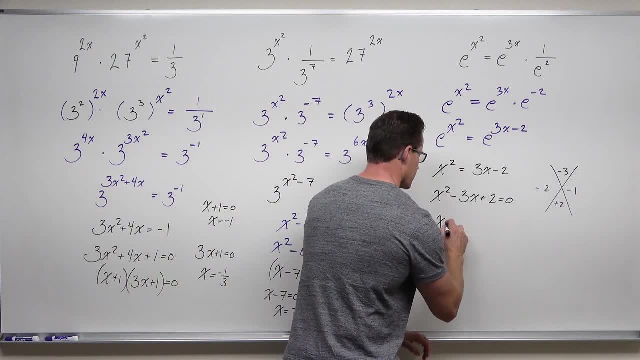 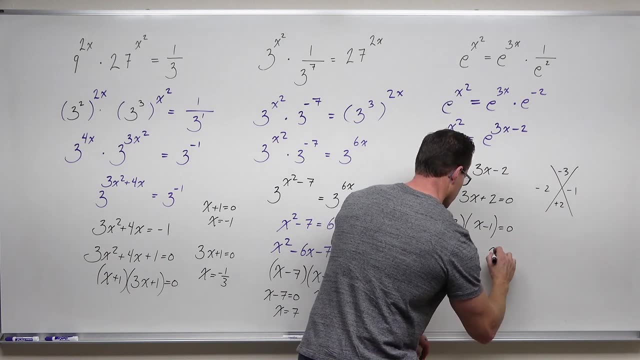 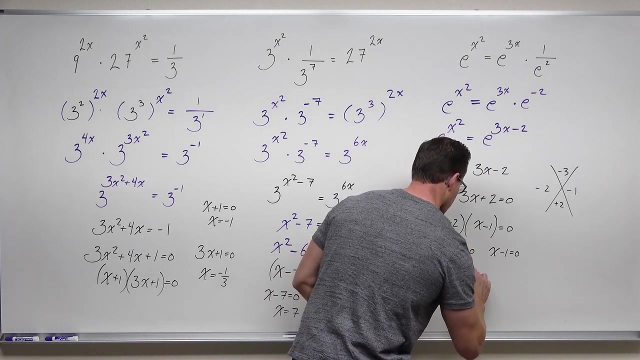 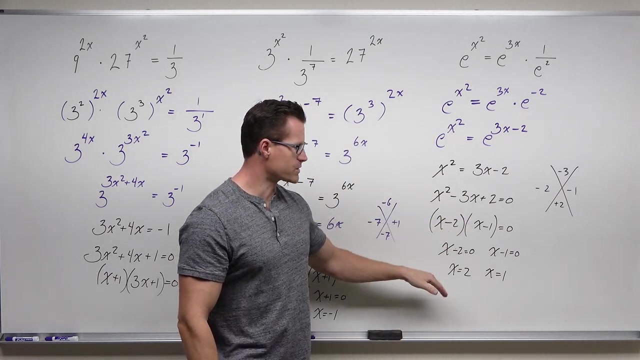 and they multiply to positive two. so those are our factors. So if we look at this, so x squared minus three, x plus two, we said each of those equals zero by zero product property. we solve them straight down, we get two and one. 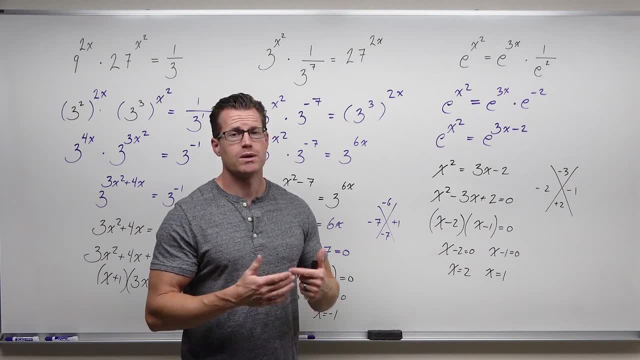 You notice, I haven't been doing this very often, but I'm gonna show you right now that you can, as I said, you can, actually check your work here. It does work. I haven't shown it to you, It's kind of on. 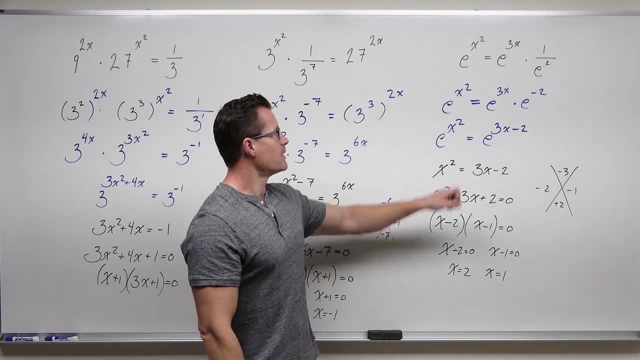 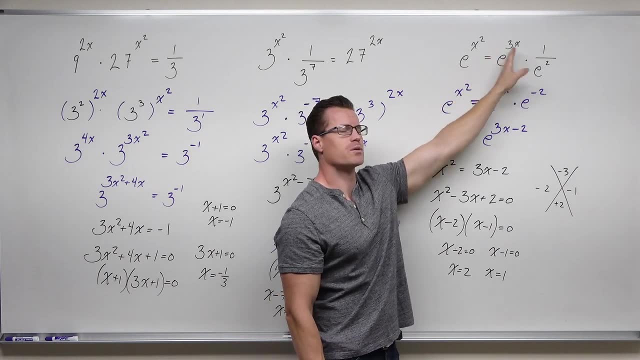 you, but you can do it. If I take 2 and evaluate it, this would be: e to the 4th equals e to the 6th times 1 over e squared. Remember that if I were to divide those, I would subtract e to the. 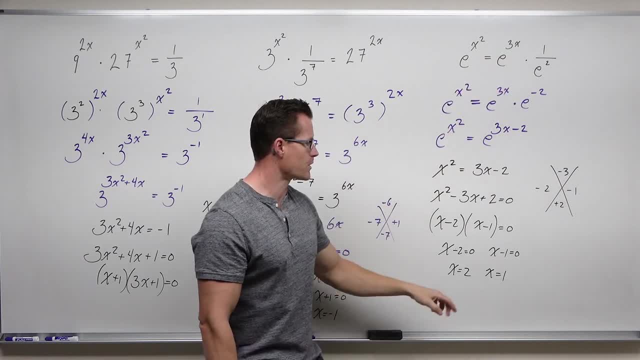 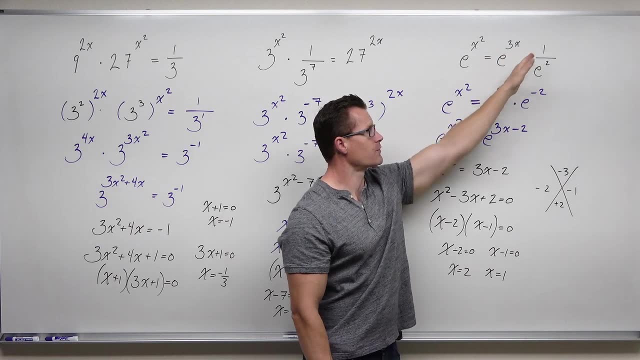 6th over e. squared would be e to the 4th, e to the 4th equals e to the 4th, Or I would have first power. This would be e to the 1st, e to the 3rd and e to the 1 over, e to the 2nd, e to the 3rd. 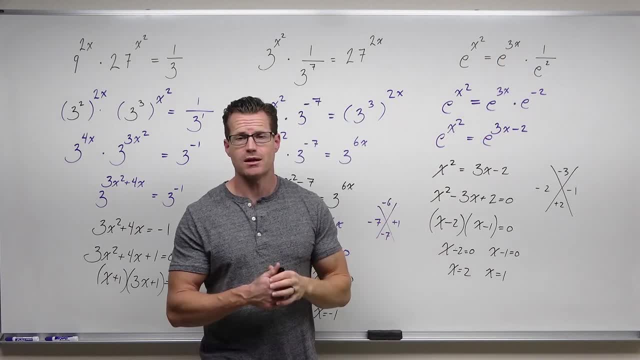 over e to the 2nd would give you e to the 1st. They do work. You can check them in these equations. That's just fine. The other thing I wanted to tell you was what, if you were able to? 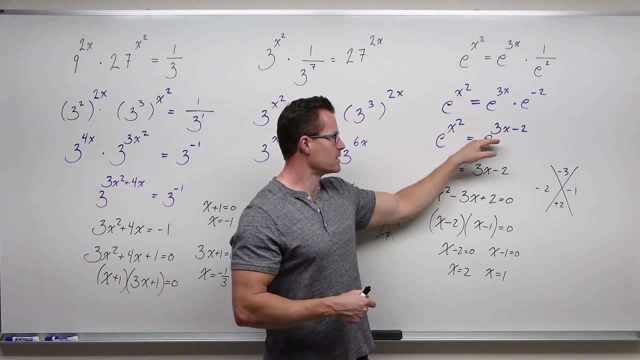 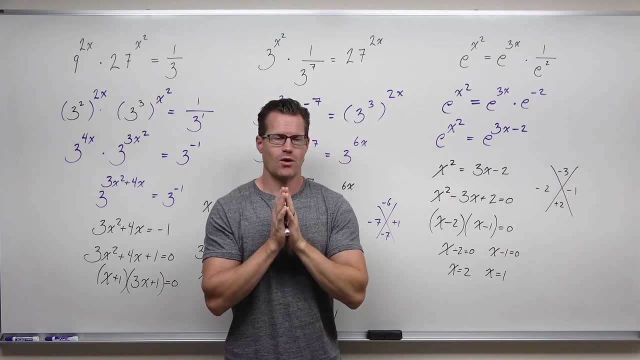 what if you were able to get all the way down here and then you set these exponents equal and you get something that's not factorable? Firstly, try again, because almost always these things are factorable, But if they're not, we already know that if you have a quadratic, that's. 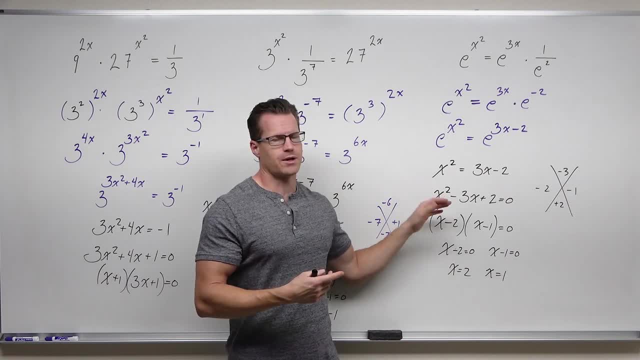 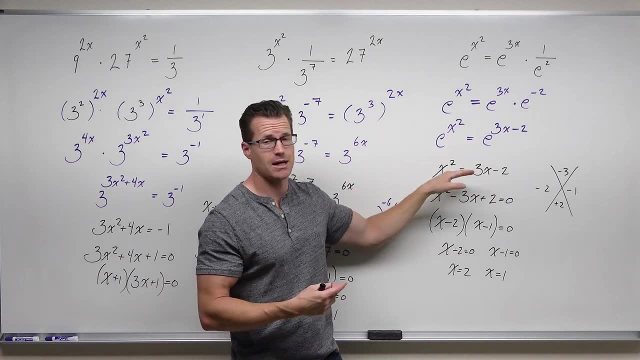 not factorable? well then, you can use the quadratic formula. Don't be afraid You're bad. So this is really. the technique I'm showing you is how to get down to right here and then say, oh, my exponents are equal. Done. If this doesn't work, I'm going to teach you. 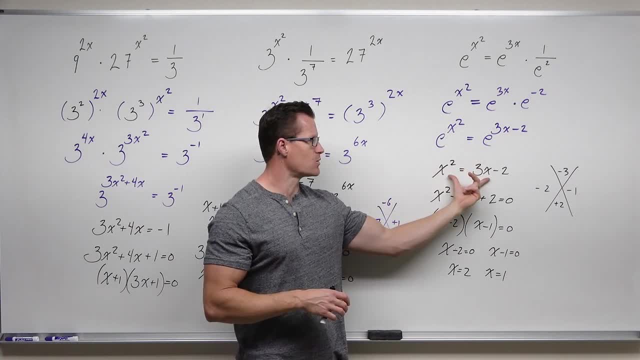 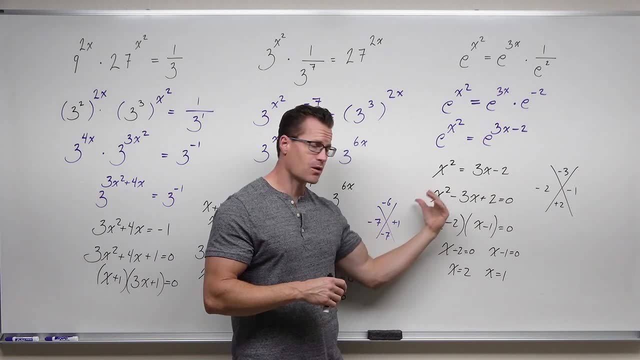 logarithms in a while. But this technique of setting exponentials equal, this opens up the door for anything else to happen. So what I mean is, if you set your exponents equal and you can't, you get everything on one side, you can't factor it well, you might have to do quadratic formula. 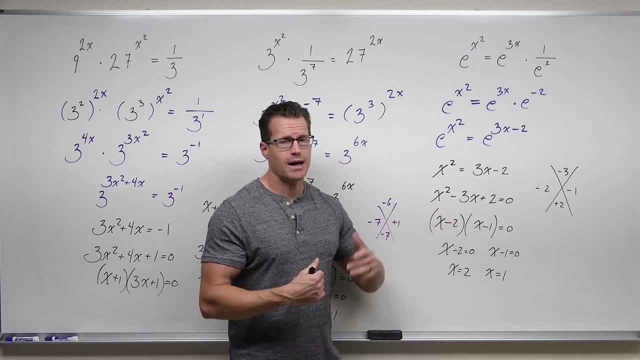 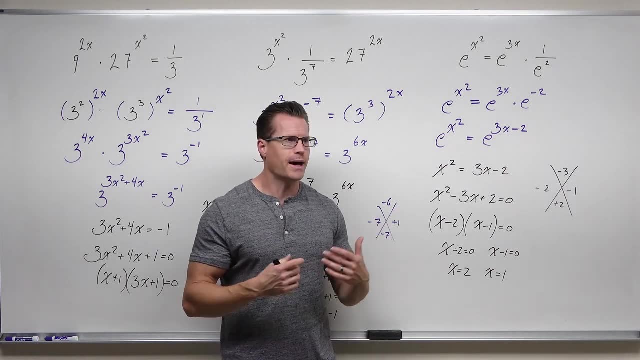 You might have to do man. this would be just nasty. but you might have to do something like rational zeroes theorem. If you do that, you're going to get a lot of things. So if you do that, it's not factorable. You power three or higher. it's not factorable. That's a potential I doubt. 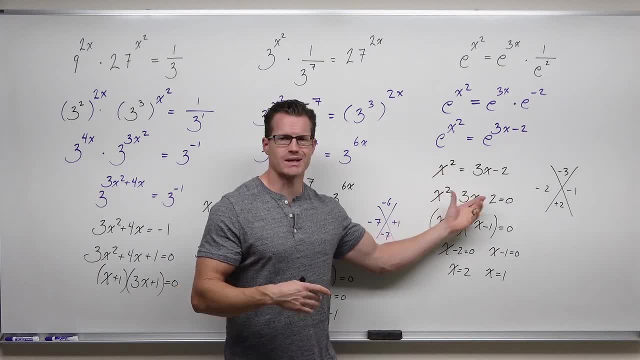 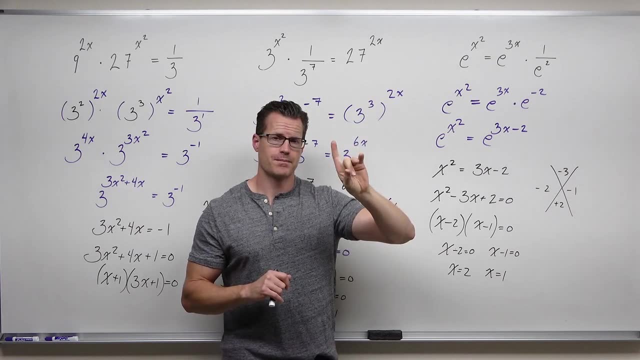 you're ever going to see it. But keep in mind that these are all factorable to keep it nice. They don't have to be, But the technique is, if you have exponentials, one way to solve them is to get two exponentials on one on each side with the same base and set your exponents equal. 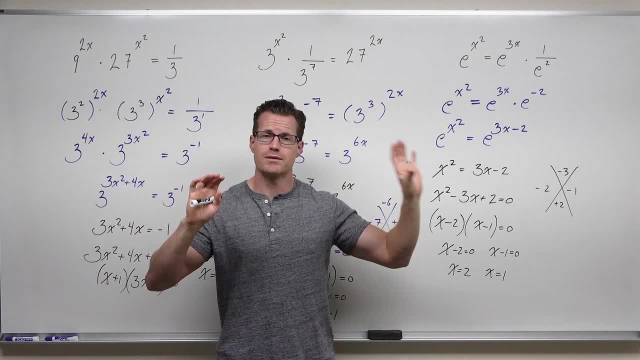 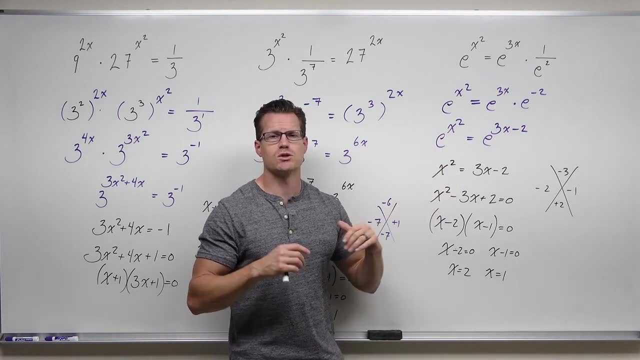 If that does not happen or you can't make it happen, you need another technique. Typically, you'll have more than one term on each side. You need a substitution And then eventually, if you can't get common bases, you will need logarithms. That wraps up. 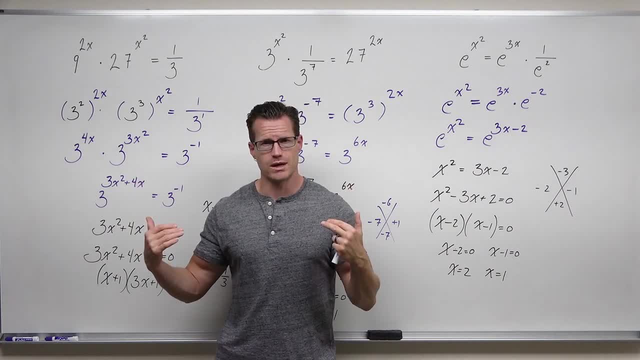 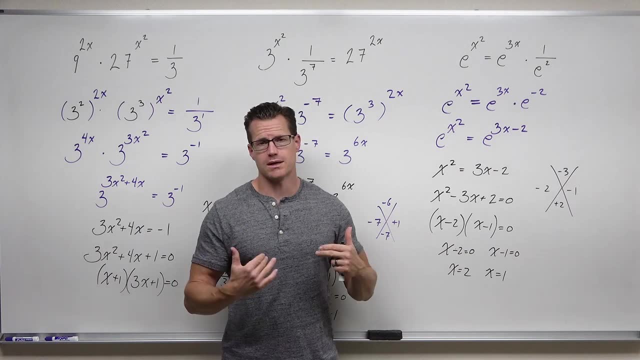 everything I really want you to know about solving these exponential equations with common bases. As far as I really want to go next time, what we're going to do is we're going to start talking about what a logarithm is. We'll start taking that graph of an exponential. We will find the 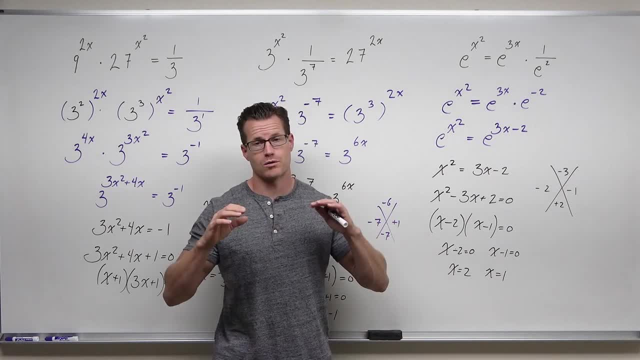 inverse of it. And then we'll say: that's the graph of a logarithm and what logarithms do. So we'll graph logarithms, We'll talk about how to solve logarithms And we'll talk about how they're inverse of an exponential. Hope you're hanging with me. I hope you enjoyed the video. I'll see you for another one soon. 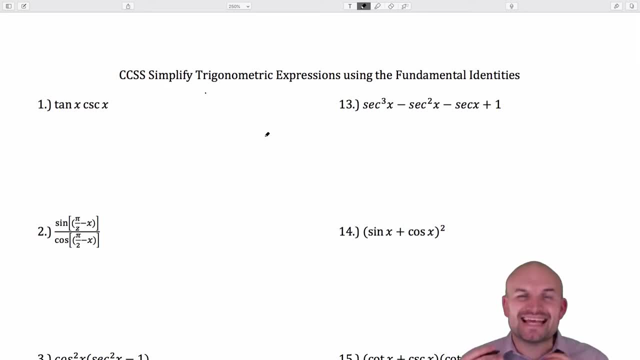 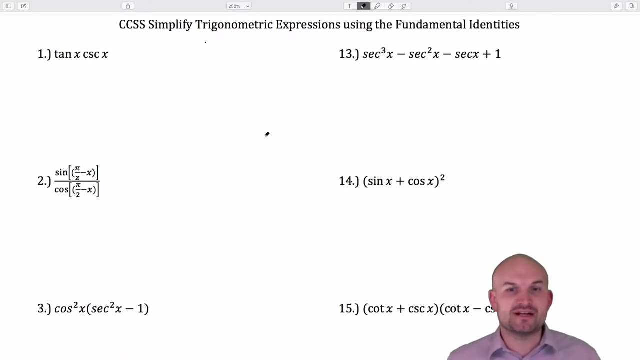 Welcome, ladies and gentlemen. My name is Brian McLogan, and in this video, I'm going to show you how to simplify 24 different trigonometric expressions. Now we're going to do that by applying algebraic and arithmetic operations, as well as using the identities for trigonometric